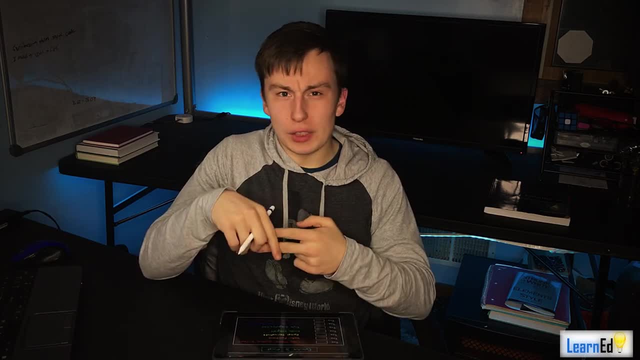 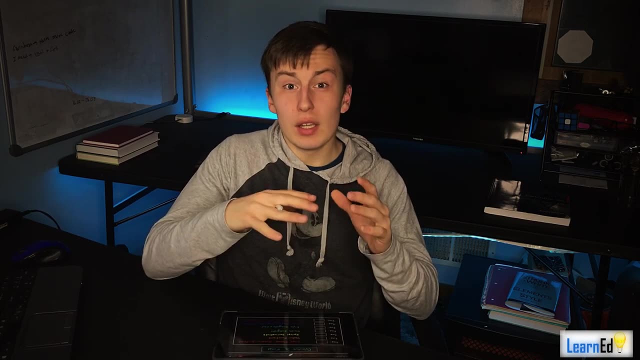 going from the equation of planes to Lagrange multipliers, right. So there's a lot of very different topics and I want to make sure that I can hit on all of those and make sure that you understand them conceptually, Like, for example, when I was in calculus three a few semesters ago. 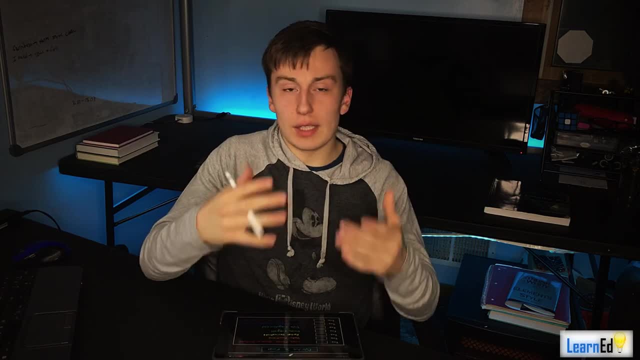 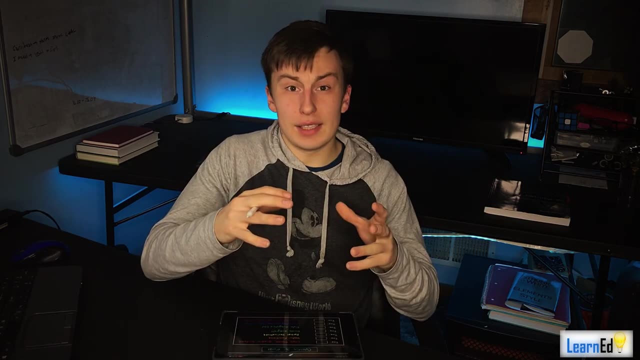 I, you know we. I did directional derivatives, I did gradients, I did Lagrange multipliers, but I never really understood what they meant. and I want to make sure that you understand what they meant, Because then it's going to be, you know, easier to understand what's going on when you're given a 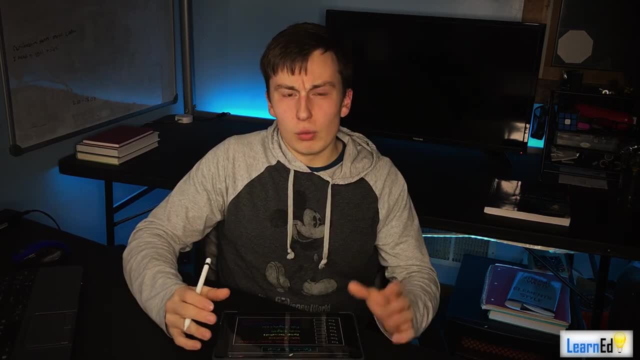 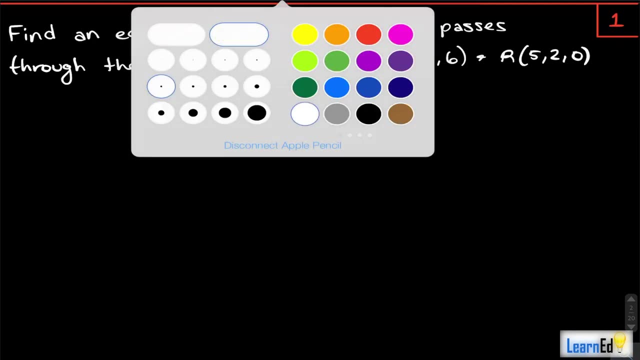 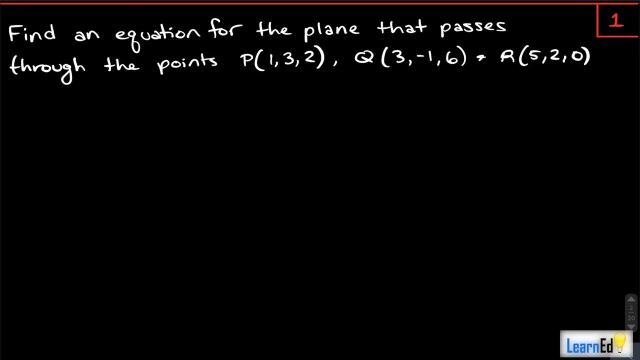 problem with those topics, Okay, so, anyways, let's hop right into this, and we're going to start off with our first problem, which is asking us to find an equation for the plane that passes through the points. We have 1, 3, 2, we have point Q, which is 3, negative 1, 6, and we have point R, which is 5, 2, 0. Now, when we look at the equation for the plane that passes through the points, we have 1, 3, 2, we have point Q, which is 3 negative 1, 6, and we have point R, which is 5, 2, 0.. Now, when we 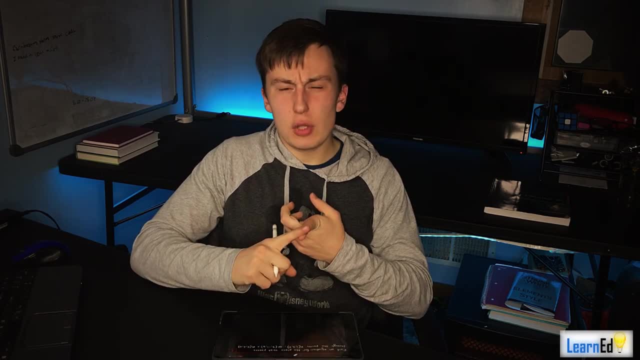 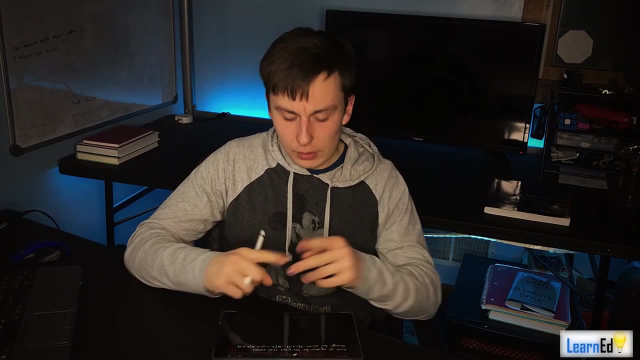 find the equation of a line. what are the two things that we need? Well, we need a point that's on that line and we need the direction of that line, Right? So I'll even write that down here. Okay, I'll write that in gray. So, for a line. 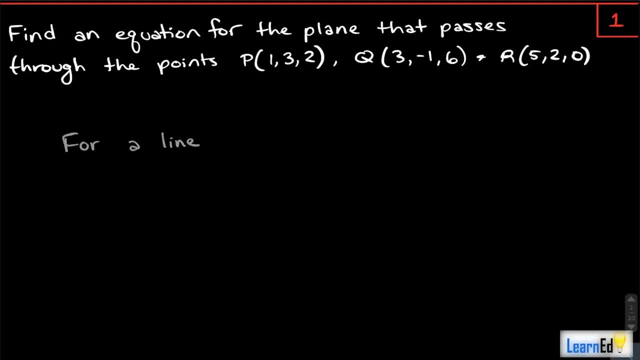 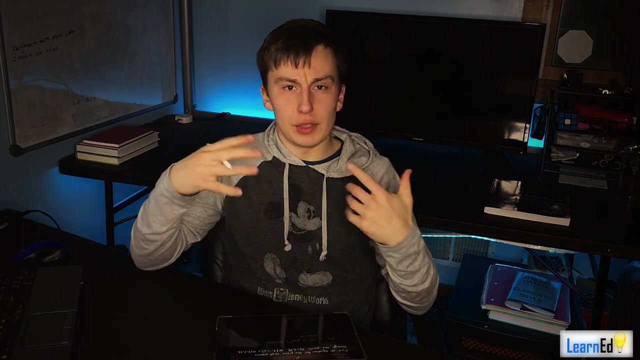 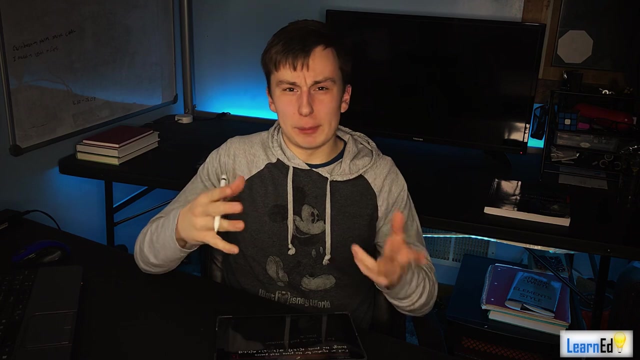 we need point and direction, But for a plane we can't just have a direction right, So that direction, if that's just pointing in the direction of the plane, there could be infinitely many lines which you know that you could draw from. So it's not very specific and what will happen is you can also have infinitely many planes if you. 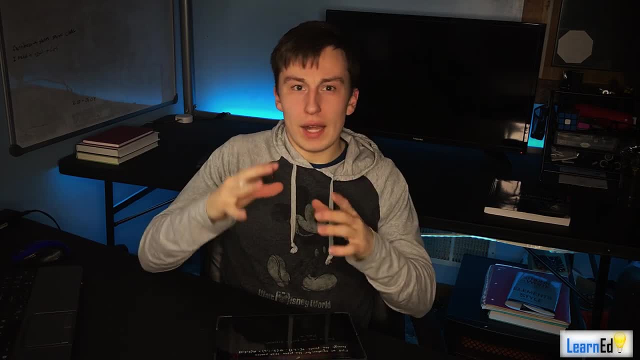 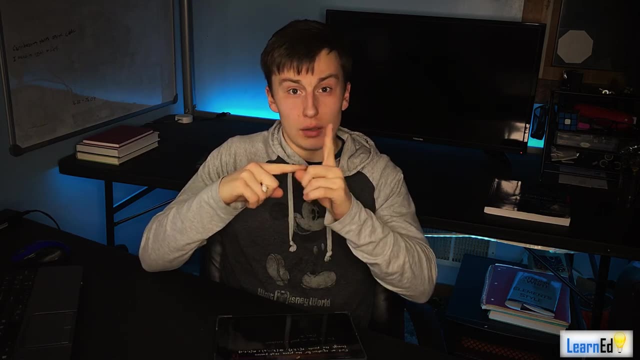 just specify one single direction, So that's not going to work out here. What we end up doing instead is having a normal vector. Okay, so now, instead of that direction being parallel to the plane- so it's in the direction of the plane- it's perpendicular to it. 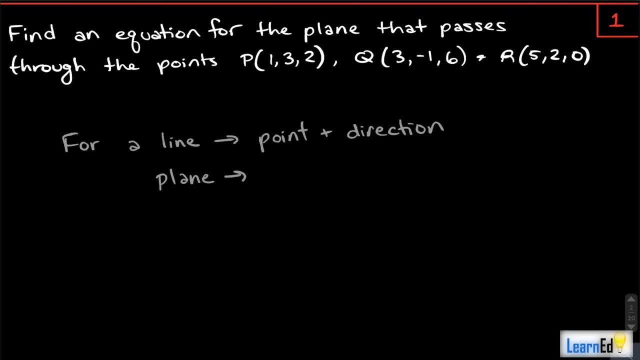 Okay, so we just have a point in the plane and we have a normal vector. Okay, and that's how we can define a single plane, All right, so the first thing that we're going to want to do: Okay, we have the points, we just need to find the normal vector. 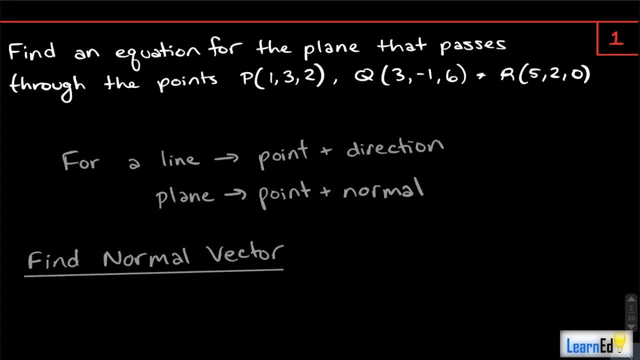 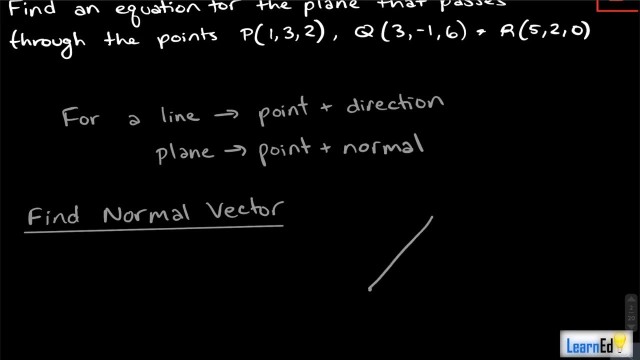 Okay, so how are we going to find that normal vector? Well, We have some points right. We can find two vectors that are in that plane, and if we take the cross product, we'll get the, the, the normal vector right. So I'll even draw that out for you, just so you can get a visual, if you're not already seeing that. 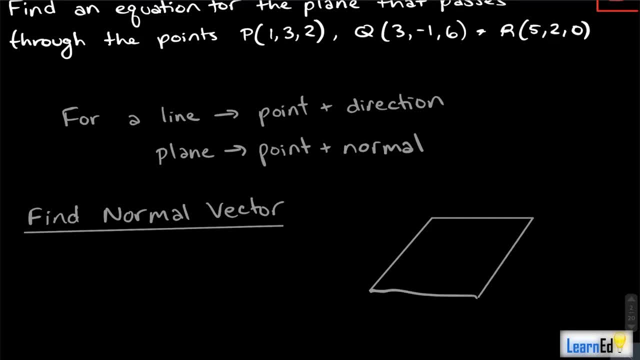 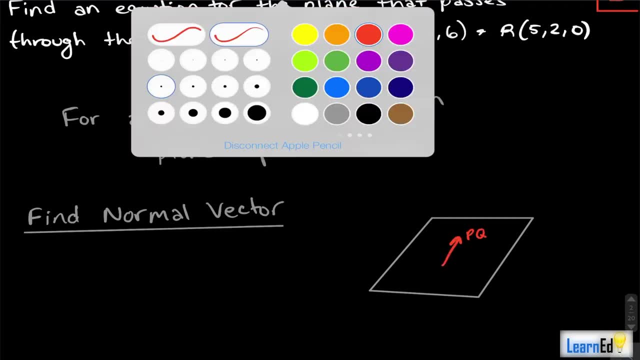 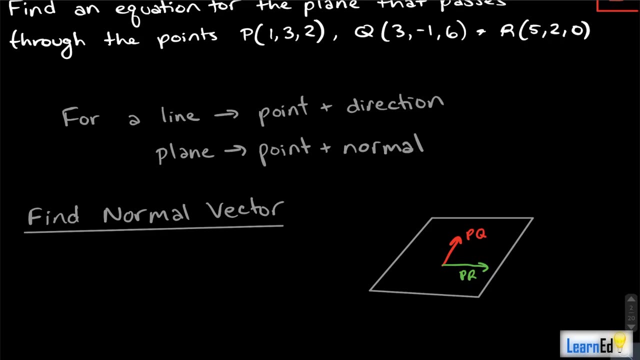 Okay. so we find two vectors. Okay, let's say, we find vector pq- Okay, and we find vector pr- okay, well, we can. what we can do is take the cross product of these two vectors and get a vector that is normal to both these vectors. so it's: 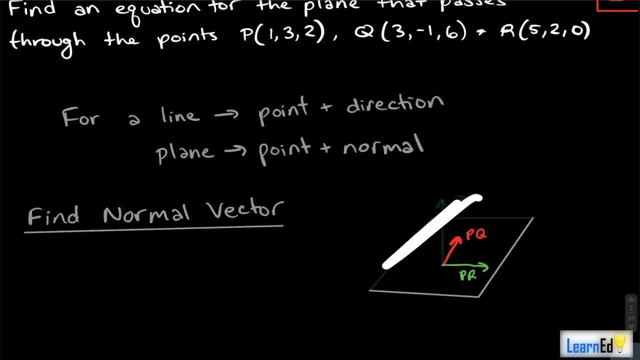 normal to the plane. All right, so that's what we're going to attempt to do here. All right, let's start off and let's find our first vector, which is this one here, Which we will do. we'll do point r subtracted from point p. 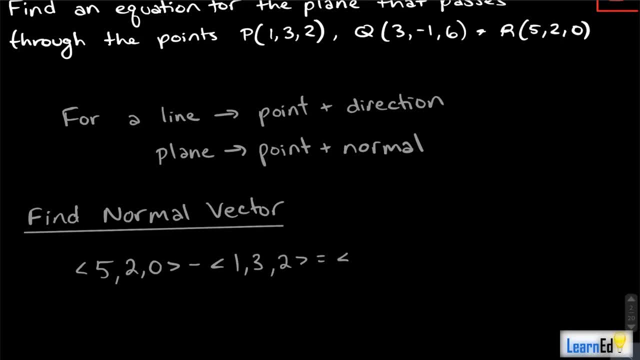 Okay, and we get just: five minus one is four. Two minus three is negative one. Zero minus two is negative two. So we get our first vector. All right, this is a vector in the plane. Now let's get our second one. Let's take that. 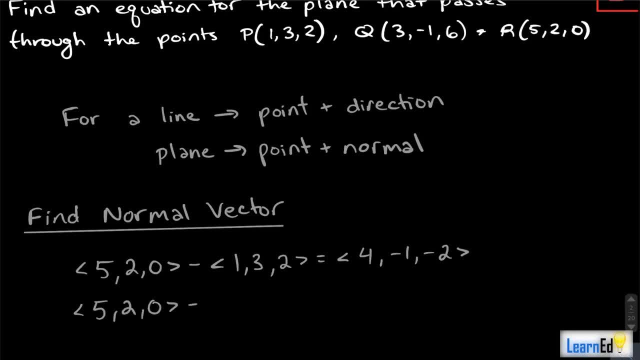 point r again. okay, you can do any points that you want. i'm just doing these because these are what i already have written down. um, we have three negative one, six, okay, and if you subtract these out, five minus three, two, two minus negative one is three and zero minus negative, or sorry, zero minus six is negative six, okay. 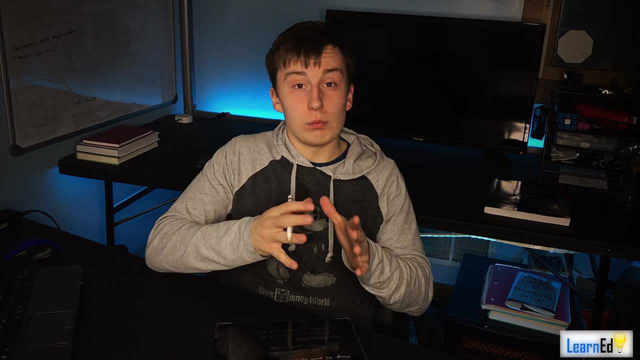 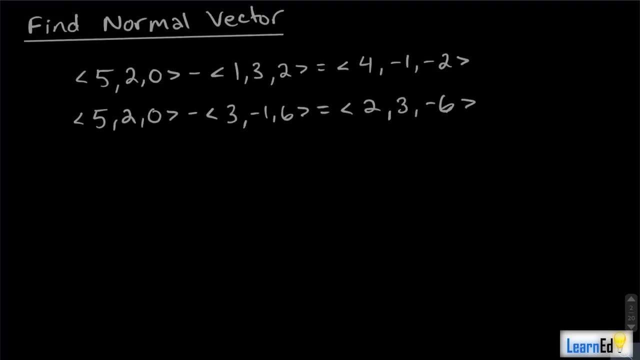 okay. so now all we're going to do is take the cross product and then we have our normal vector. so if we're going to take the cross product of these two vectors, we got to set up our matrix, okay. so we have, i hat, j hat k hat. okay, we have four negative one, two as our first. 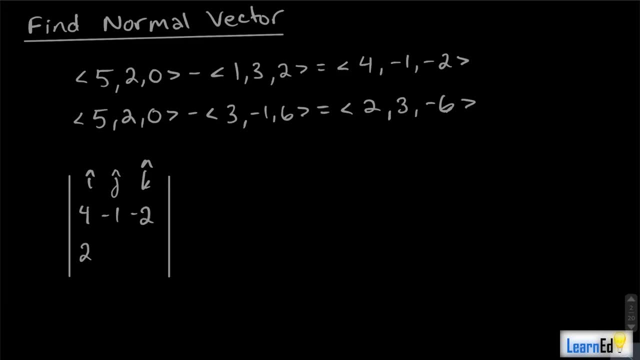 vector: negative two. we have two, three, three, negative six as our second vector. and now we just take the cross, we just find the determinant. rather so we have i hat times. we have a negative one times negative six, minus a negative two times three. okay, and that's your i hat. then you have minus j hat times, it's going to be a four times. 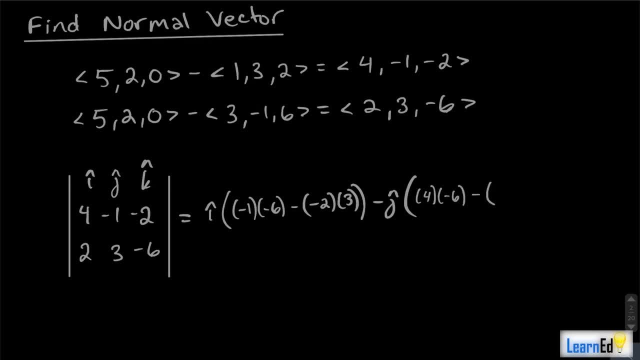 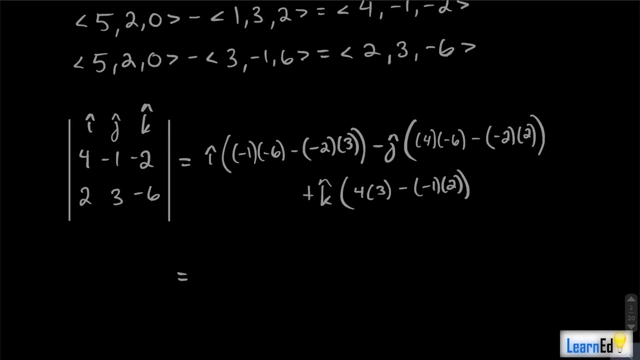 negative six minus a negative two times two, and then you have plus k hat times four times three minus a negative one times two. all right, so simplifying that down- and i'm sure you guys probably skipped some steps if you tried this on your own beforehand. um, i'm just doing this all out for completeness sake. i won't drag on like this too much. 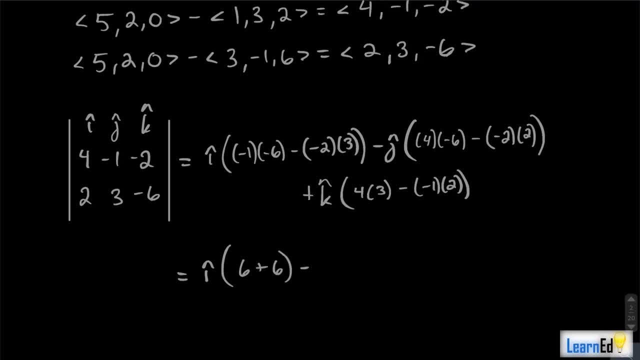 we're gonna have a six plus six here. we're gonna have minus your j hat times, there's a negative 24 plus four. and then we have plus k hat times, it's a 12 plus two. okay, so our normal vector just ends up being 12. i minus, not minus, it's actually going to be a plus. 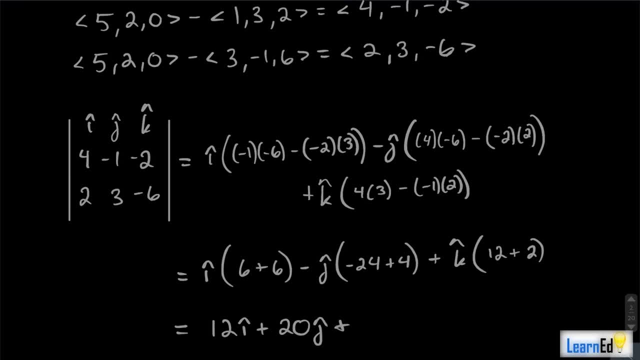 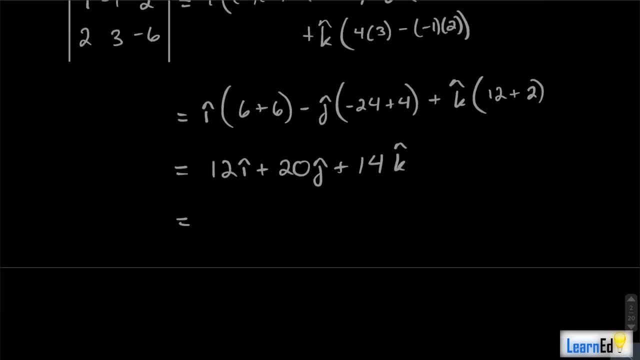 20 j hat and then we're going to have plus 14 k hat and we can also just simplify this down to make things easier for ourselves and make this 6 i hat plus 10 j hat, plus 7 k hat not a big deal. 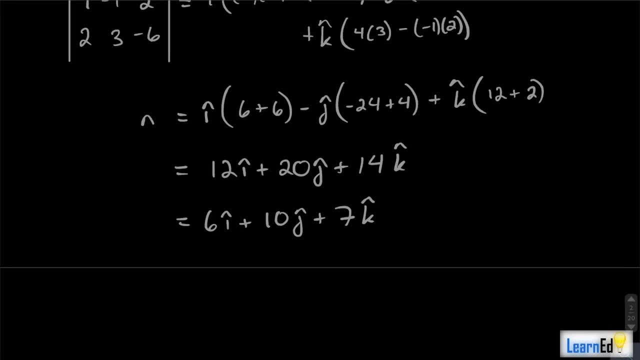 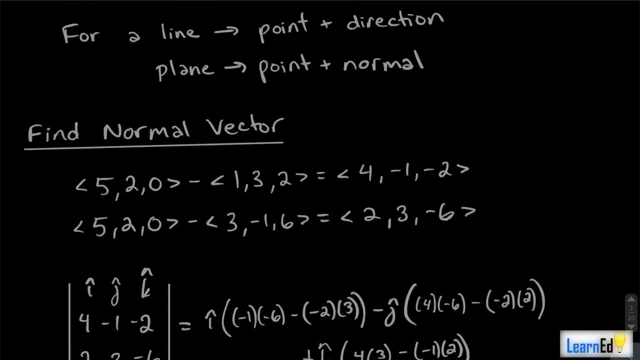 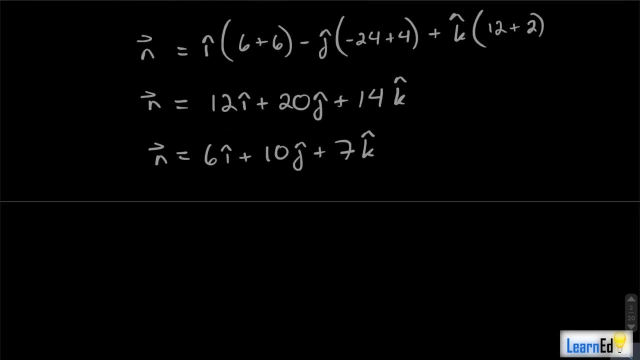 i mean, it's the same thing, okay, and uh, we can say that this is equal to the normal vector. okay, so let's, let's, uh, find a point. so we, we got to use one of the points, and the point that i want to use is going to be the the first, the first point here. i'm going to use point one, three, two, okay. 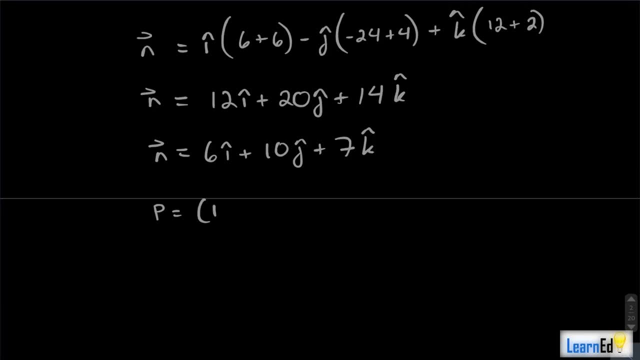 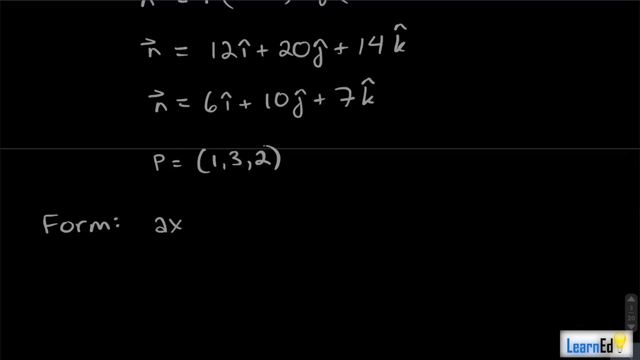 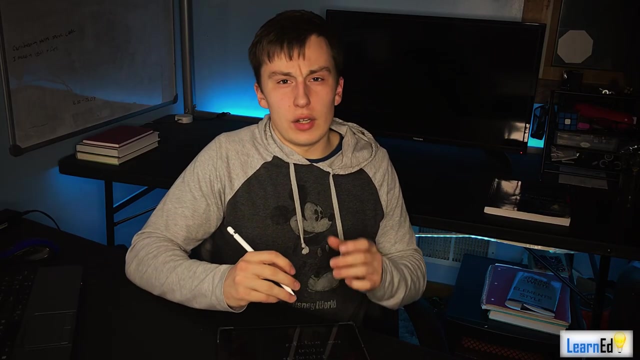 so we have a normal vector and we have our point, which is one, three, two, and now we just have to find the equation of the plane. okay, now, what is that equation of the plane? well, the linear form of the plane is ax. plus by plus cz equals d, and and by the way, as a quick note, you may see that d on either side. 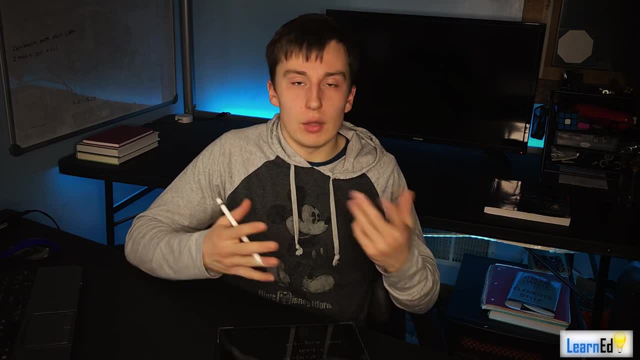 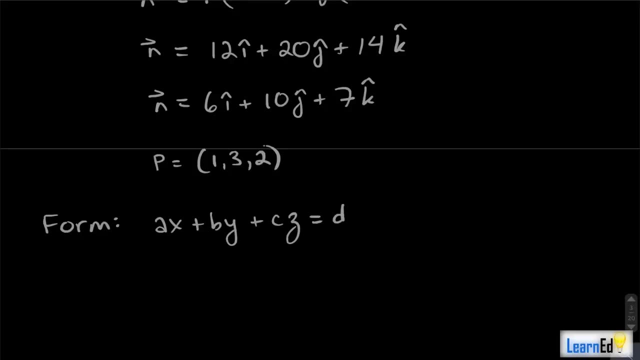 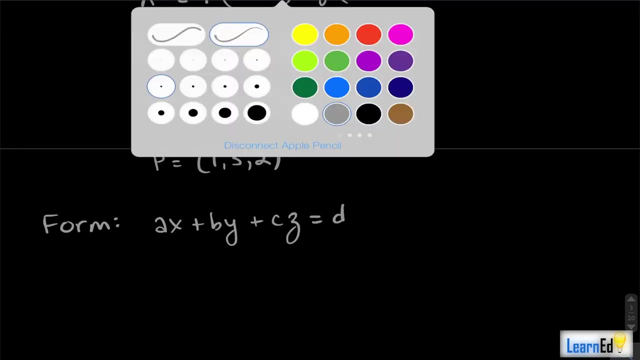 of the equation doesn't matter, not a big deal. okay, some people, you know they're just defining d, as you know, the opposite of what somebody else is. so not, yeah, not a big deal. anyways, what are? what's a, what's x, y, z, what's all that stuff? well, we know that the normal vector 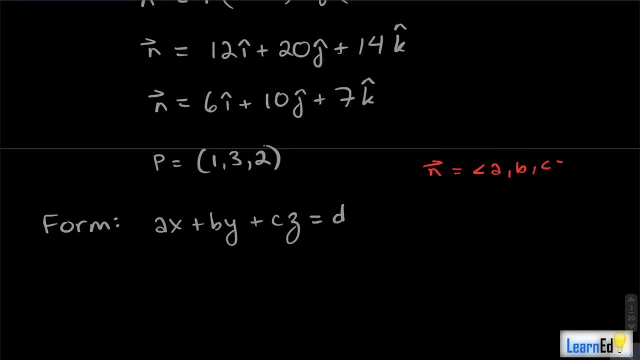 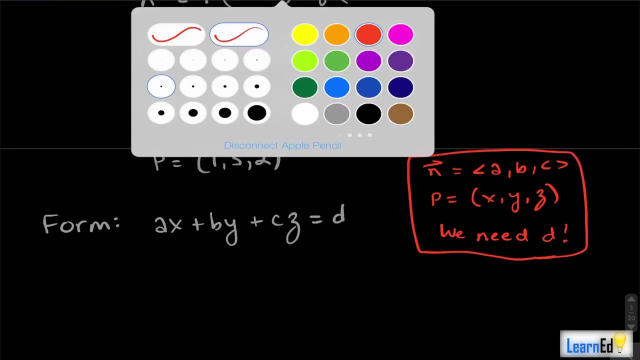 has components a, b, c, and our point has our x, y and z. okay, so what? what about d though? well, we need to find that, so we need d, okay. so that's the whole point right now, and once we find d, we're going to be okay. all right, so let's plug everything in here. 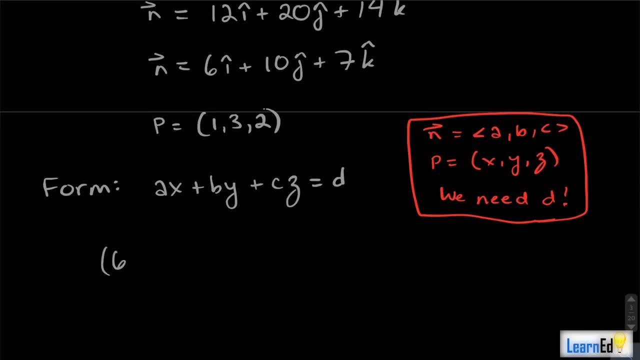 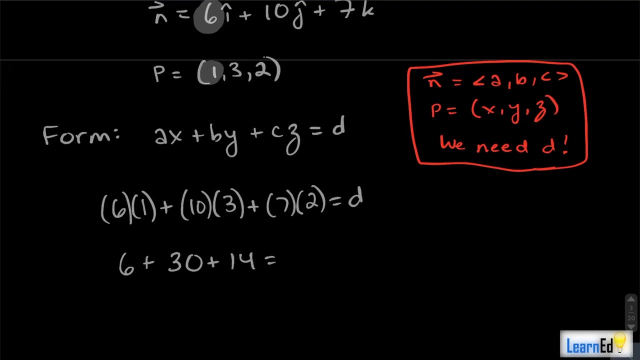 well, first off, we have: a is 6, right? so that's the. that's this guy right here. okay. then we have x is 1 and we're going to go so on through the equation. so we have: plus b is 10, y is 3 plus c is 7, z is 2 and that's equal to d. we get 6 plus 30 plus 14 equals d. 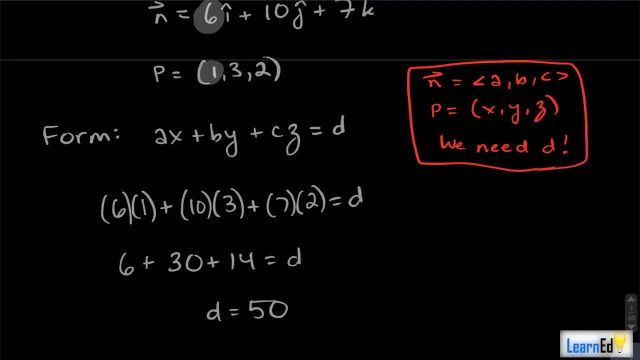 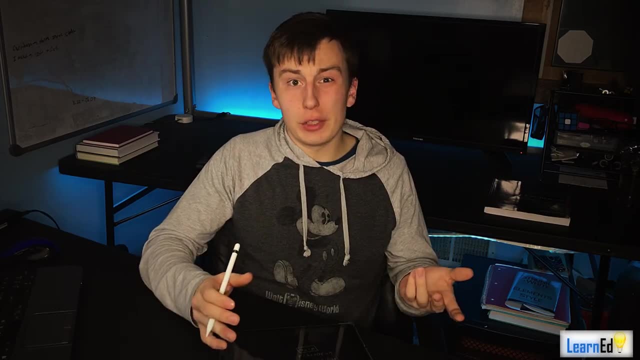 and we get: d is equal to 50.. all right, so that's great. now all we have to do is finish our equation for that plane. so we're not going to plug in for the x, y and z now. all we're gonna do is plug in for a, b, c and z. 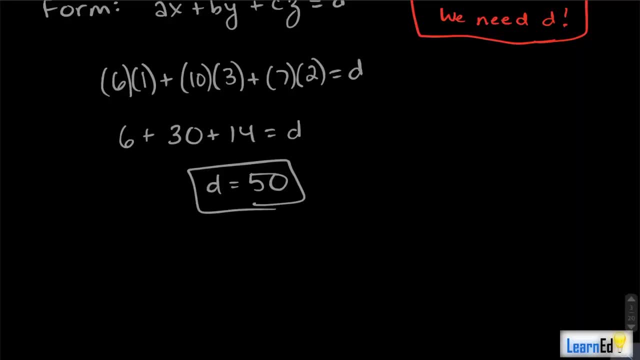 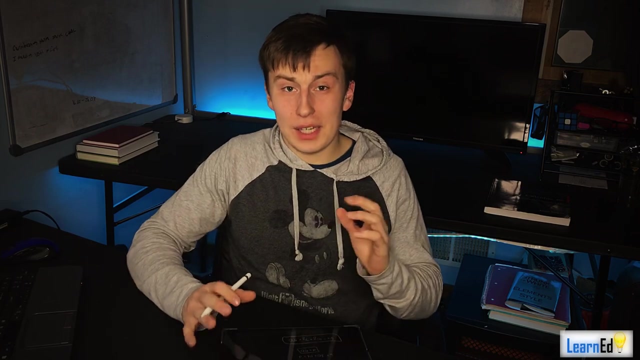 d and we're done all right. so let's get to that. we can rewrite this as 6 x plus 10, y plus 14, not 14. 7 z equals 50. and there you go, all right, so that is our first problem completed. 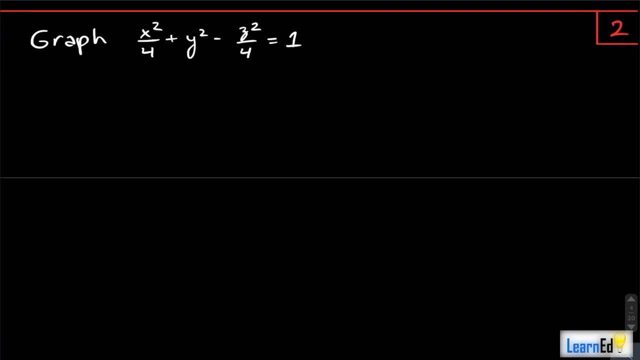 let's move on to the next. okay, so the next problem is asking us to graph: x squared over 4 plus y squared minus z squared over 4 equals 1.. now i'm going to get rid of this line. i don't like this line at all. oh well, i kind of got rid of it, never mind, all right. well, listen, here's the deal about. 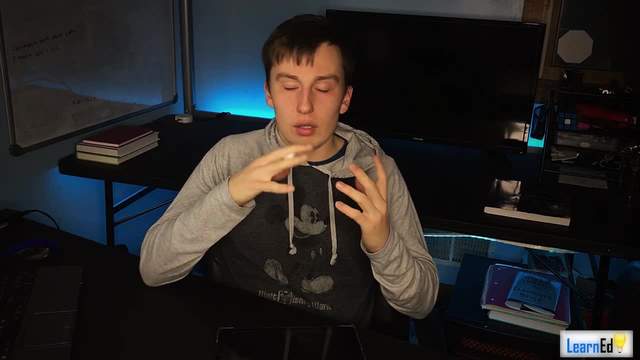 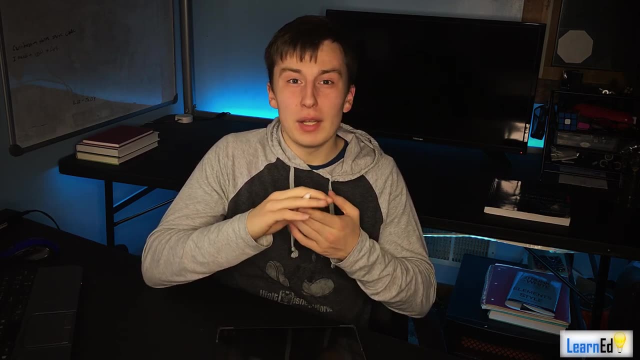 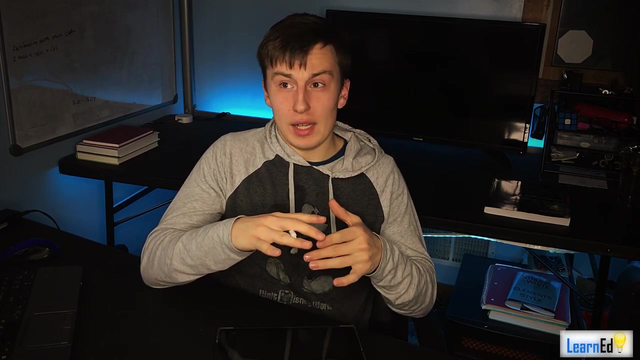 this graphing problem. okay, now, when i looked at these problems when i was in, when calc 3 and earlier on, i kind of just brushed them off, didn't really care about them, kind of just, you know, gave minimal effort, but i didn't realize how important these questions are and you know these ended up being. 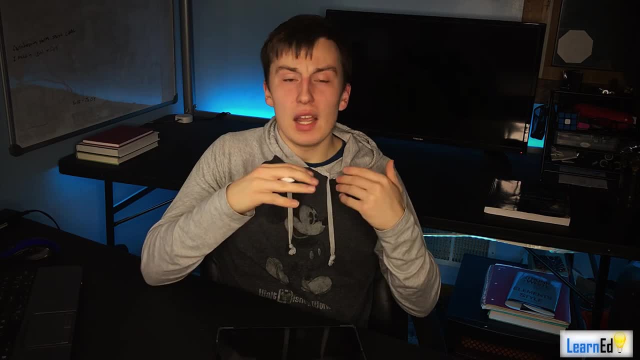 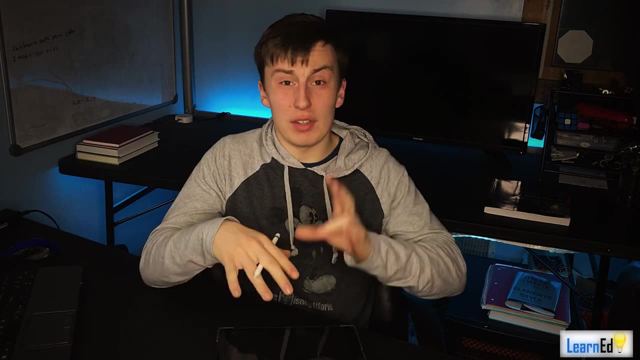 kind of the the pain of my existence when i was in calc 3, because the thing is, these are extremely important for for triple integrals- just visualizing what's going on if you're given a surface like this or you know something of the sort they you know, if you're given a surface like that double. 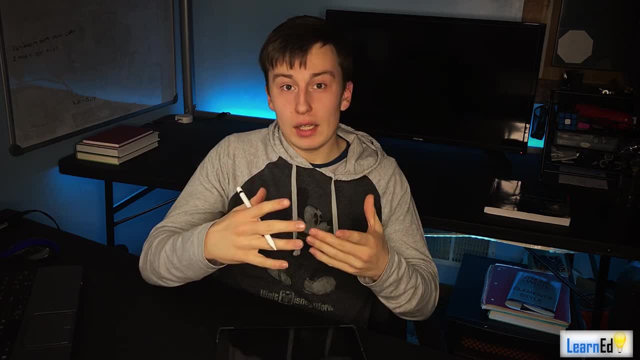 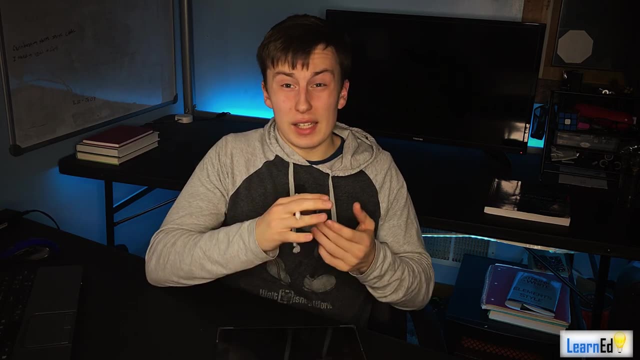 integrals, different things like that. so just understanding what you're looking at is very important. vector calculus, different things like that. so if you don't understand what this looks like, something like that, those triple integral problems, they're going to become really, really hard. so that's why. 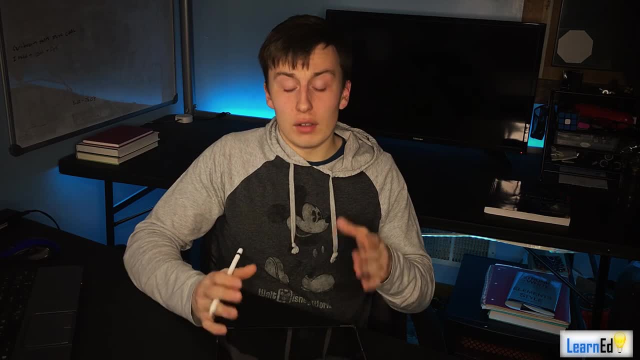 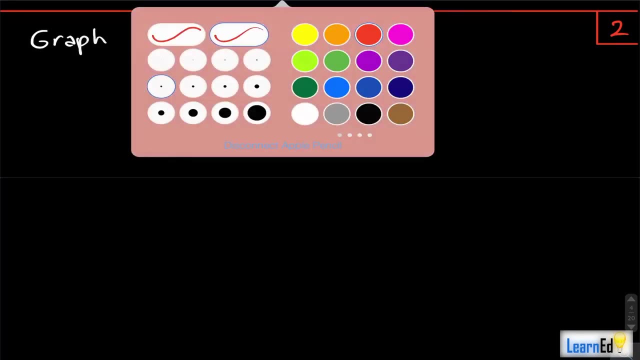 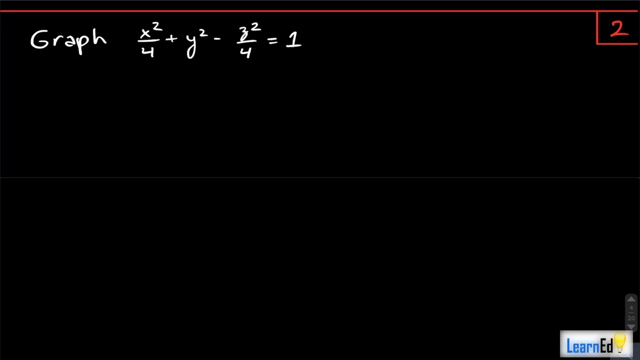 i want to make sure i go over graphing at least one of these, uh, quadric surfaces. okay, so let's examine this. okay, so just try to figure out what we're kind of going to be looking at now if you haven't reviewed your quadric surfaces before watching this video, which is understandable. 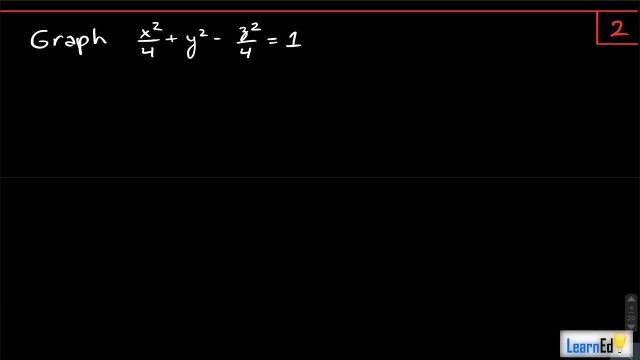 this is actually really easy to see, and the reason why i'm saying that is because this piece right here- what is that? what? what would this become if you just if you just got rid of this and you just have, like this and this piece? this is an ellipse, right? so? 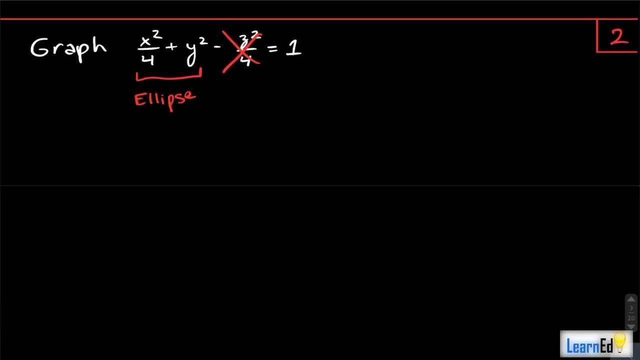 once you get rid of this again. this is an ellipse, okay, and now that i have to get rid of those crosses, okay, and rewrite ellipse, what would the other two pieces? so if we had, like, the y squared and a, um, the minus z squared over four, and we got rid of the x squared over four, what is that piece? 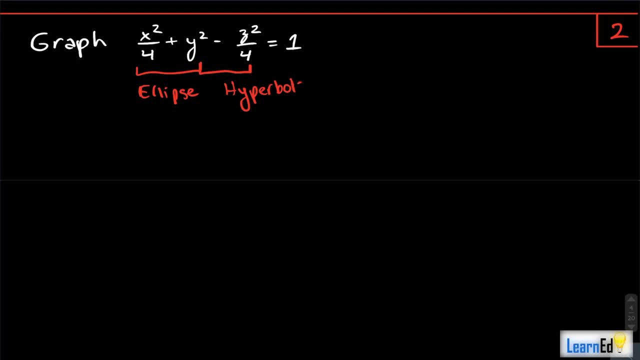 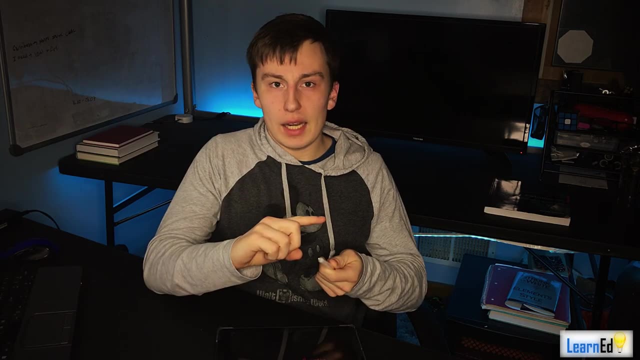 well, that's a hyperbola, right? so basically, what we see now is that our quadric surface is going to consist of ellipses and hyperbolas, okay, and all we have to do to kind of visualize this is use traces and i, if you end, 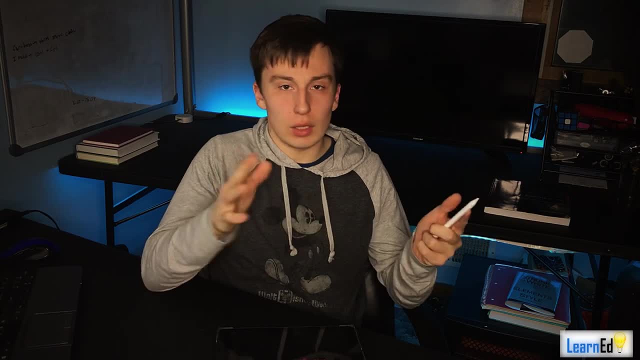 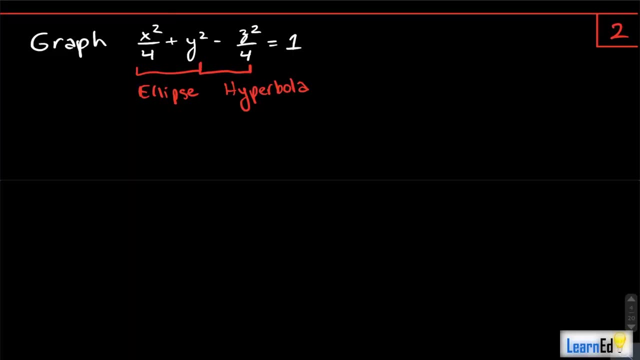 up with a quadric surface in any kind of these integral problems, uh, vector calc problems, just traces are going to be your best friend, just to visualize what's going on. okay, so for these traces, what i want to do, and first off, before we get into that, i'm actually going to set up my axes. 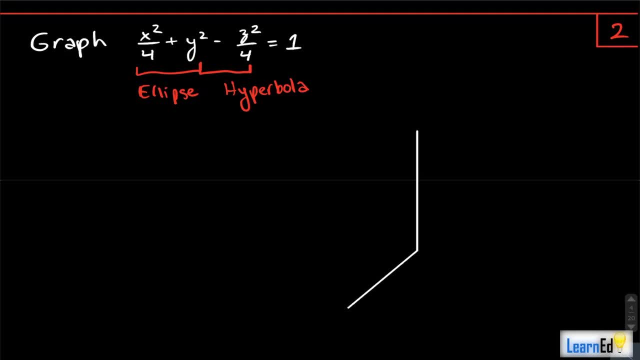 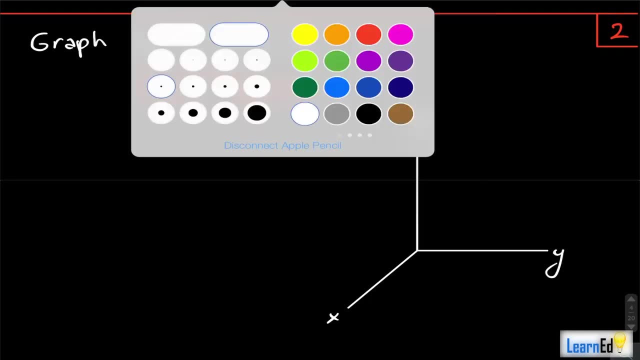 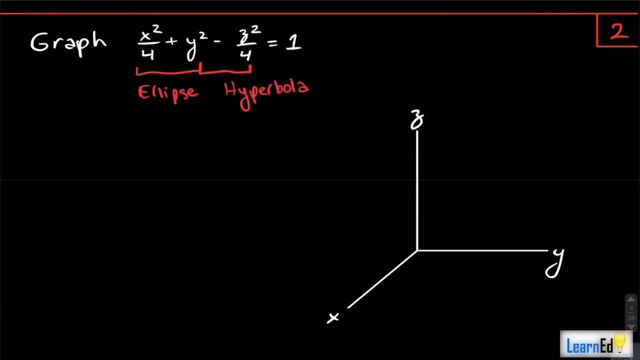 okay, and there we go. we have x, y and z, and i bet you guys wish you could do this. on the final right, have perfectly straight axes and uh, yeah, anyways, our first trace is going to be on x equals zero, okay, or actually, you know what let's do? 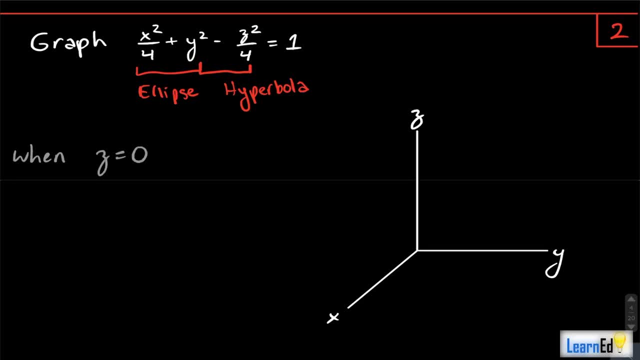 what this is. what we're going to do is we're going to set up our axes. Okay, let's do this. z equals zero. so when z equals zero, because this is going to be the easiest case, now that i look at it, we get x squared over 4 plus y squared equals 1. okay, so what is this? well, remember we said before: 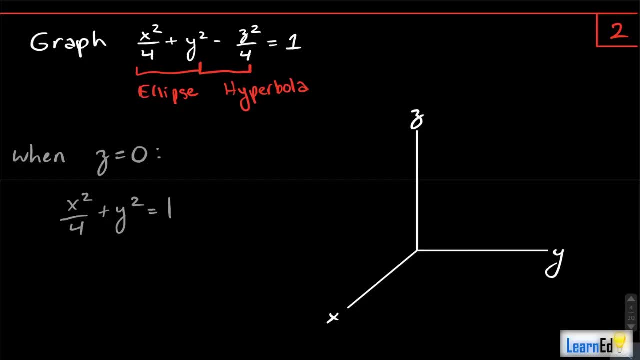 this is an ellipse. okay, this is an ellipse, so we'll just graph it as such. now, if you're confused- and this is something i would probably be be confused with, um, you know, if you're confused, what does this over 4 actually do? just set y equal to zero. okay, because then you're like, if 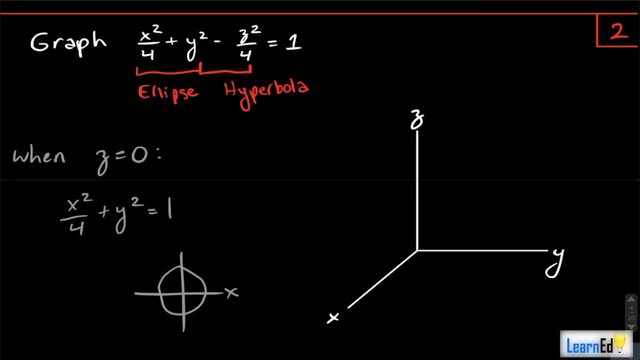 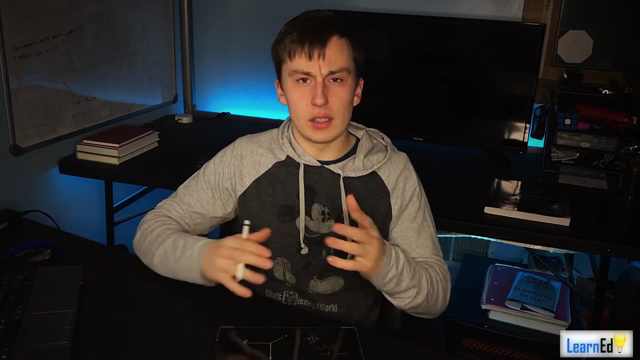 you have a circle in the xy plane and that's an awful circle, i know. but if you set y equal to zero, you're looking at either this point or this point, so you can tell how far that ellipse is shifted over on the x-axis. now, okay, that's the idea. that's why i'm saying: set y equal to zero. 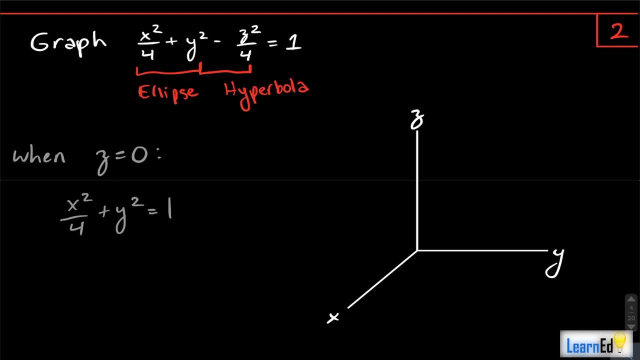 so you're kind of doing a trace of a trace, all right. so if you set y equal to zero, you just get x squared over 4 equals 1, so x is going to equal plus or minus 2.. so that kind of tells you that the x 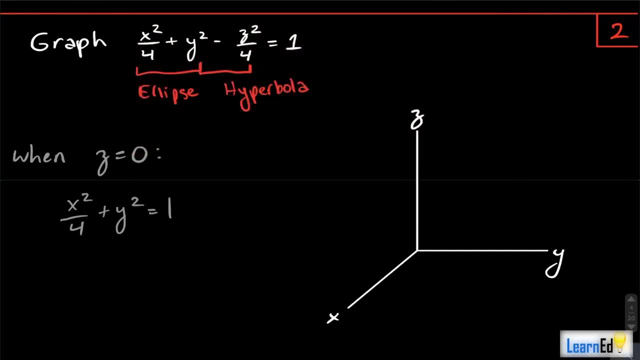 part is going to be longer than the y part, so we're going to have something like this: all right, so that's your. your z equals zero trace. okay, so next up, let's look at when- and honestly it's going to be really not fun here to do- uh, you know, setting z equal to multiple things. so what i'm just? 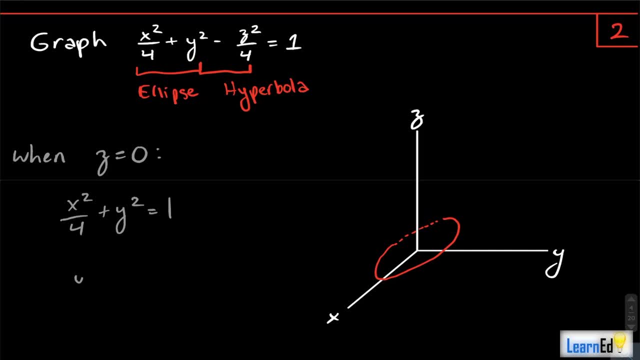 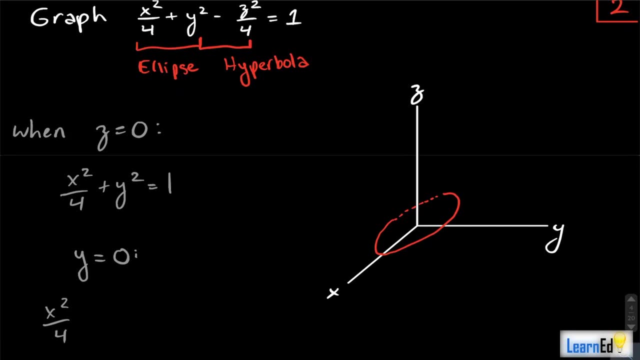 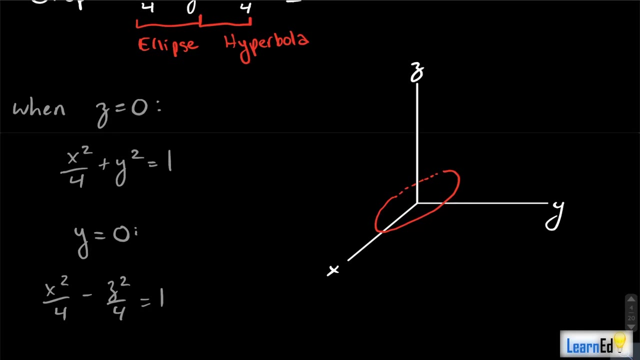 going to do is set y equal to zero next. so if we set y equal to zero, we get x squared over four minus z squared over four equals one, and this is just a hyperbola. okay, so we know that between our, that if we just have a our graph on the the x- z axis, it's just going to be. 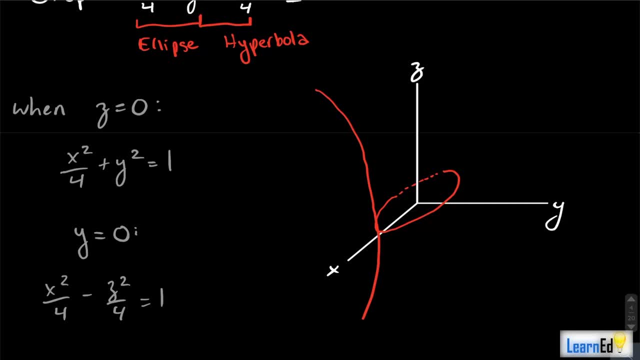 a hyperbola. so we'll have a hyperbola right here and a we'll have one in the back right here. all right, excuse the drawing at- i'm not the best artist in the world if you haven't already, but anyways. uh yeah, so that's our y equals zero trace, and then we're just going to do our x equals. 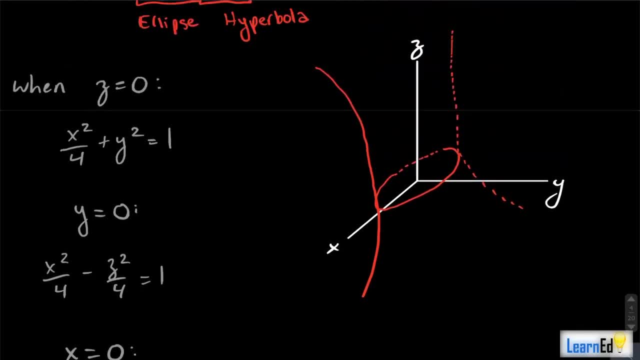 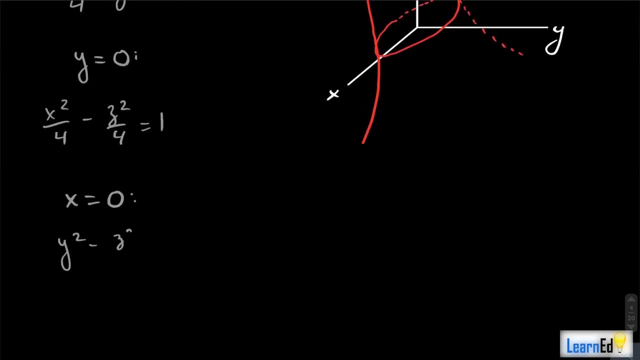 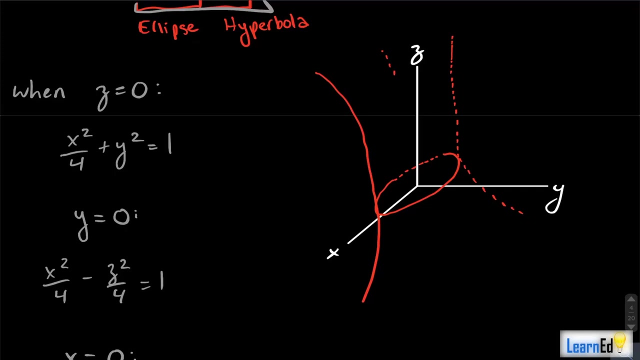 zero trace, and i'll do that down here. and when x equals zero, this equation up here is just going to become: y squared minus z squared over four equals one another hyperbola. so we can just see that that would come in the back here and uh, we'd have like one coming down here. but that looks. 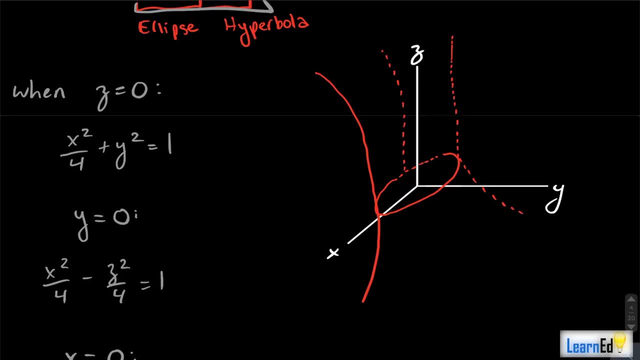 really gross now. so i'm just going to get rid of these and but you understand, like, what it looks like now. so i'm just going to erase those for just like, since it's going to be easier to look at it, and i'm going to try to draw this, not bad. 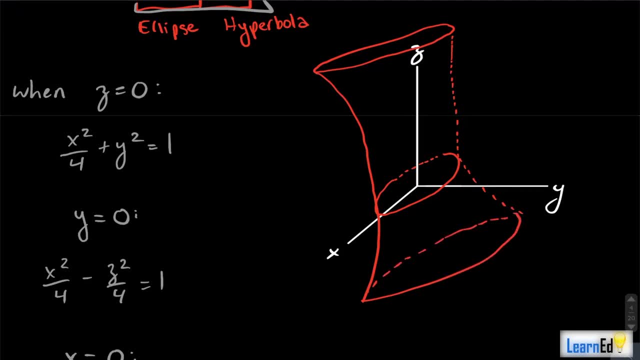 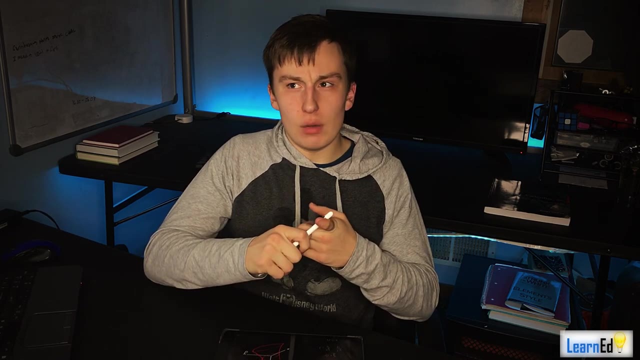 okay, okay, could use some work and good, all right, yep, that's as good as it's gonna get guys. so, uh, that's all i can do now. you may be wondering: how do i know if it's a one-sheeted hyperboloid versus a two-sheeted? 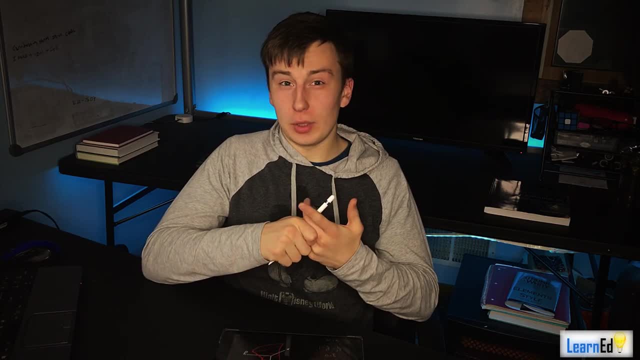 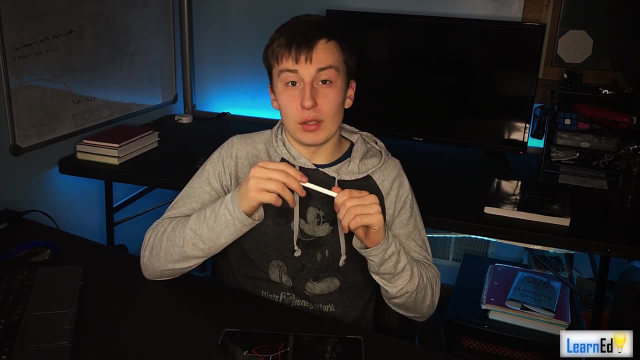 hyperboloid. now you can figure this out from traces, but uh, you know it may. it may just be easier to remember that a one-sheeted hyperboloid is a one-sheeted hyperboloid and a two-sheeted hyperboloid is a one-sheeted hyperboloid. 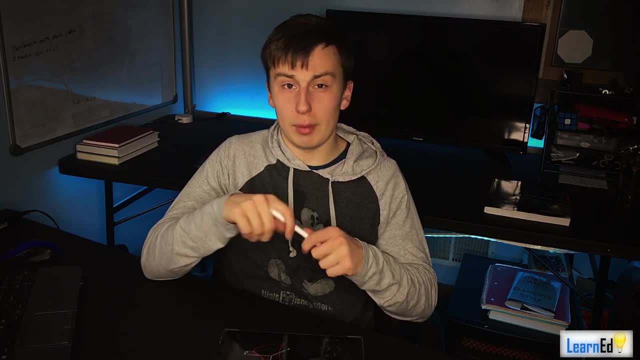 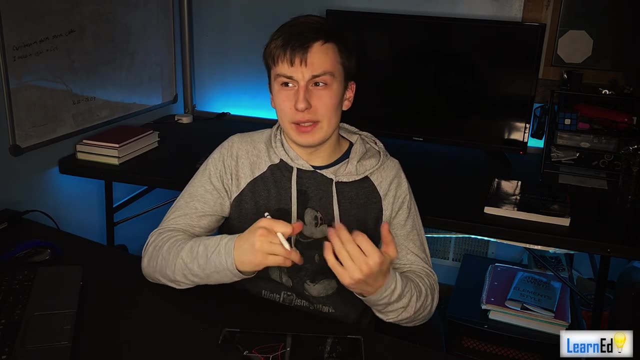 is when you have one minus in the equation and a two-sheeted hyperboloids, when you have two minuses. right, so one sheet, one minus, two sheet, two minuses. okay, that's how i would remember it, just because it's it's quick and simple. that's not too hard to remember. um, you know one and one, two and two, but 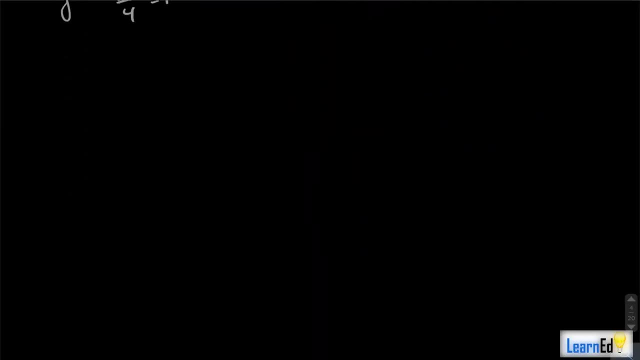 yeah, anyways, let's move on to our. our next problem, and this will kind of be the last of our graphing problems- this is going to be with vector functions now, since we are in the orange section, okay, and we are being asked to sketch and find the domain of the vector equation r of t. this should: 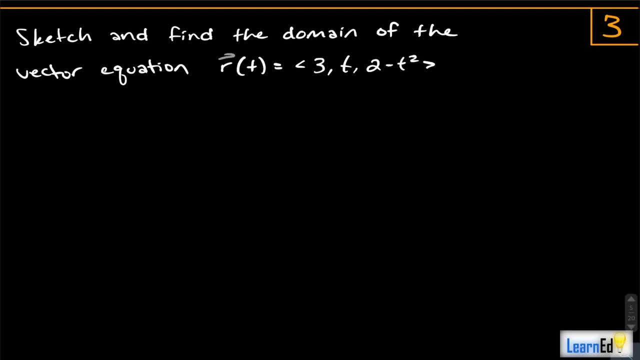 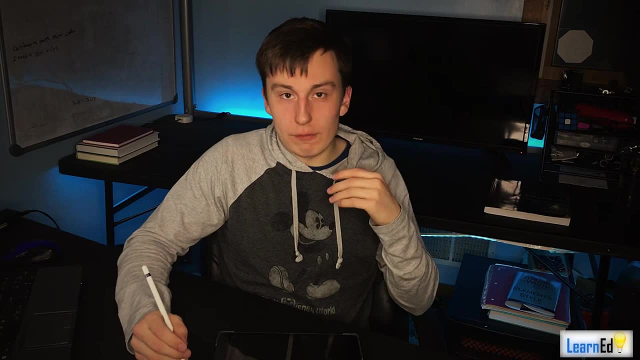 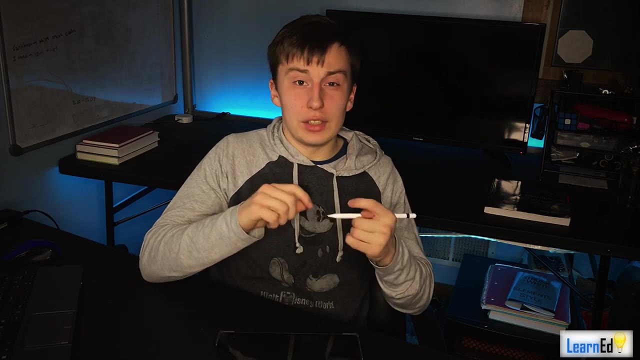 have a arrow here equals the vector. we have three t and two minus t squared. okay, now go ahead and try this on your own if you feel comfortable with it. if you don't, you know i'll go through it again, but it is good it. it is really good to just try these problems on your own, and maybe you are more. 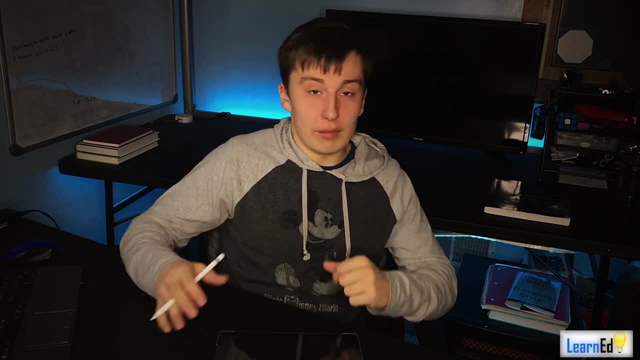 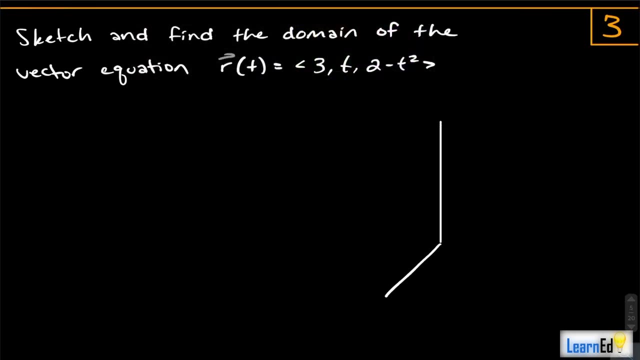 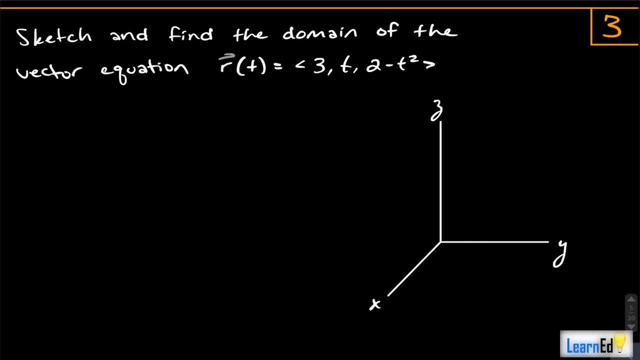 is just see how each individual parameter is behaving. so, for instance, since three is in our x entry, we just have x equals three. okay, this is something that's constant. so this entire curve is going to be happening where x equals three. okay, if you have a constant. 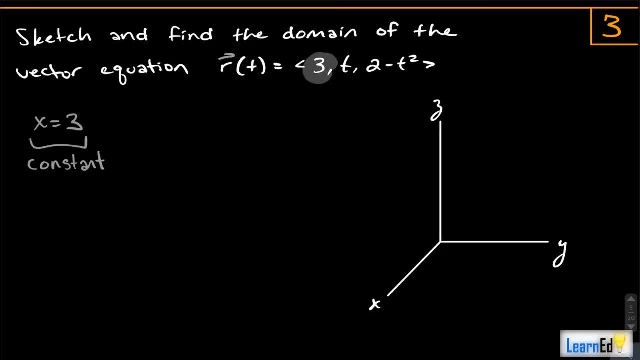 like that in a vector equation. it's really really nice. okay, so we go one, two, three- okay- over in the x direction. so everything that is going to be happening for our graph is going to be happening in a shifted y- z plane. okay, so now let's look at our other stuff, our other parameters. so we 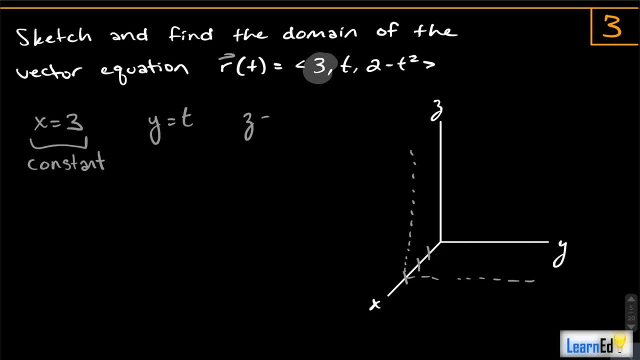 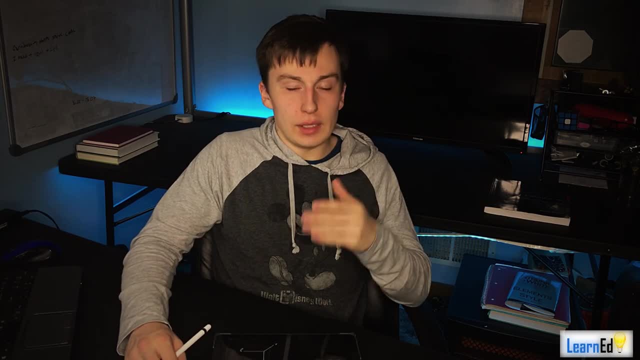 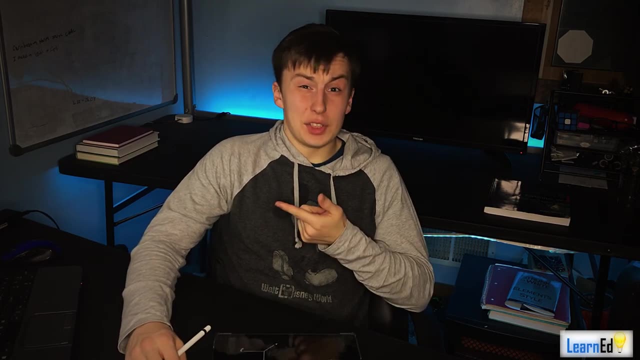 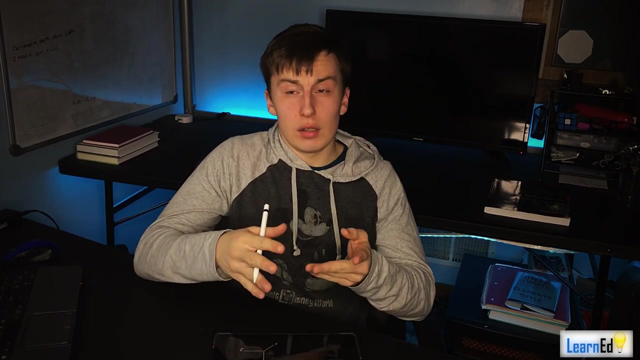 have y equals t and we have z equals two minus t squared, okay, so y is just increasing by t. now if y is t, okay, then we can just plug that in to the z equation, honestly, and, and then we have. since we're only dealing with something on the yz plane here, we'll just have an equation with: 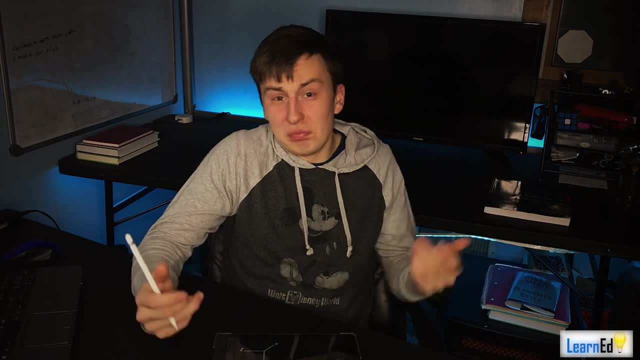 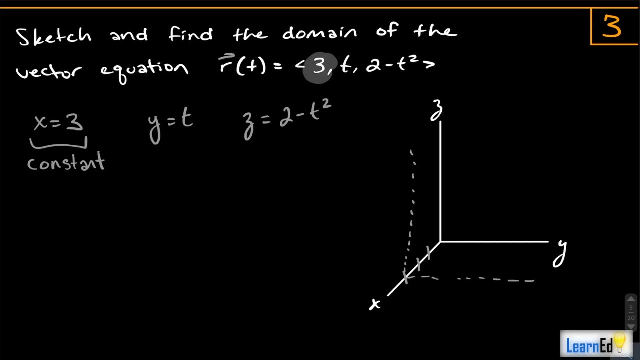 of z with respect to y, which you know. that'll work out pretty well, especially since you know we already have y equal to t. so if we do that, we combine these two equations, here we get z equals two minus y squared. what does that mean? well, we're just going to end up with. 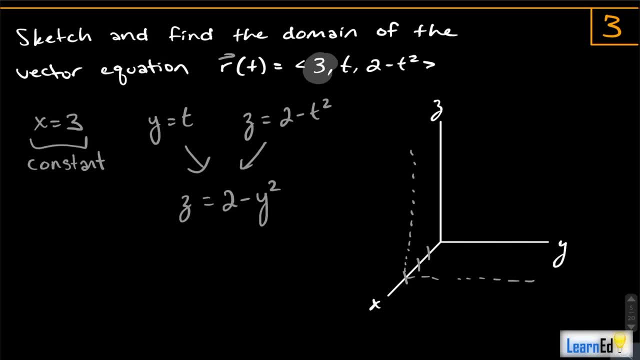 a really nice parabola here and the졳 quer הא�能 91, Poinat. it's just going to look something like this: okay, And I'm not going to include that arrow. actually, Let me redraw that. 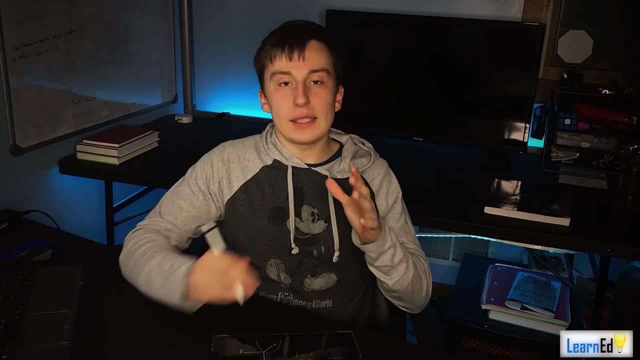 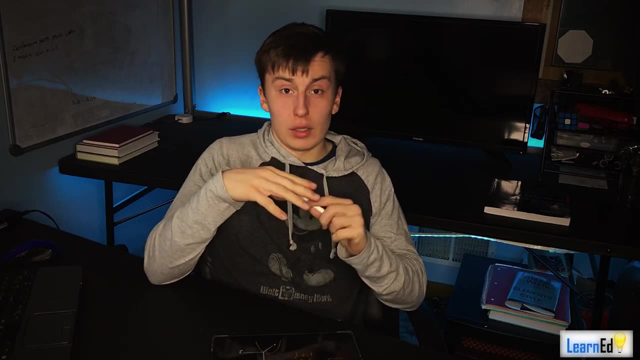 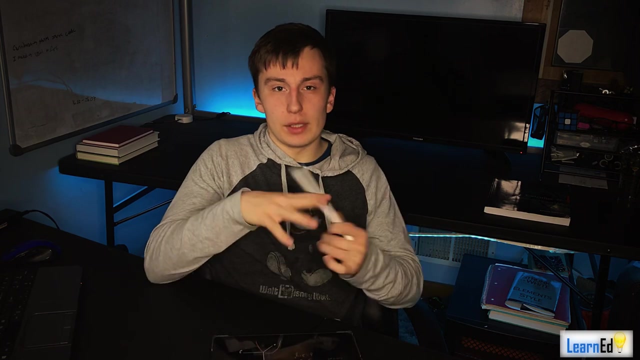 Nice, okay, Because the last thing that we're going to have to do is draw some arrows to denote the direction of the vector function. okay, So try to get that right now. If you haven't been able to get this so far, just because you looked at this problem and you were like 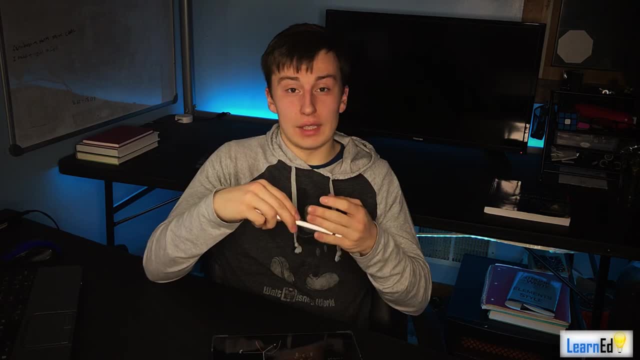 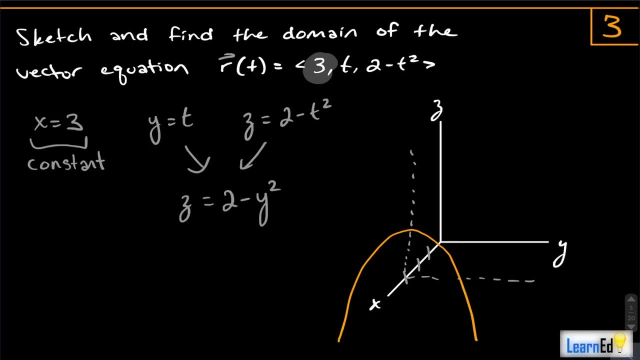 what do we do? Because that's exactly what I would have looked at it with before I reviewed this, honestly. So how are we going to tell what direction it's moving in? Looking at this, all I would do is: okay, y is equal to t. 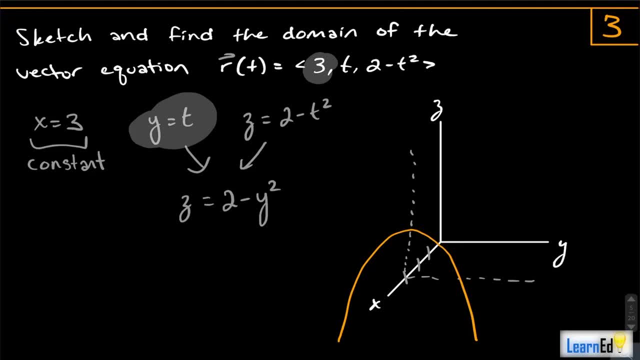 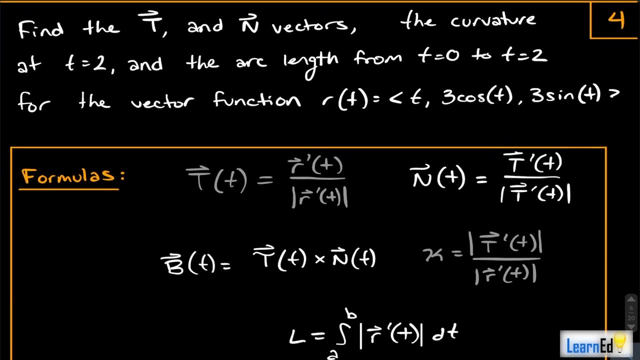 So as y increases, t is increasing. So that gives it right away, y increases in this direction. So this parabola is just moving in this direction. okay, That's that All right. and then we have number four. We're going to find the unit tangent and unit normal vectors. 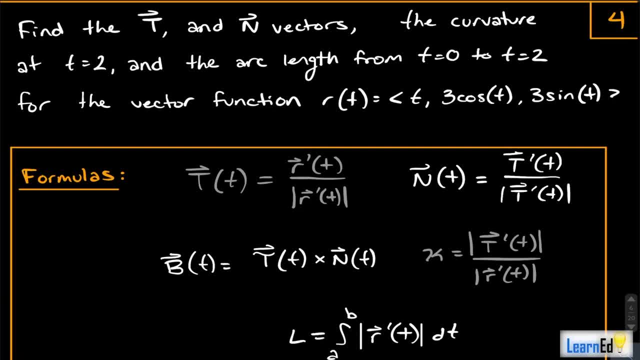 We're going to find the curvature at t equals 2 and the arc length from t equals 0 to t equals 2, for the vector function r of t equals t 3 cosine, t 3 sine t. I have all the formulas that you're going to need right here. 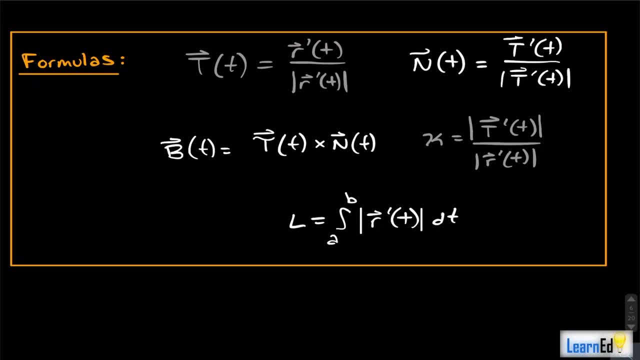 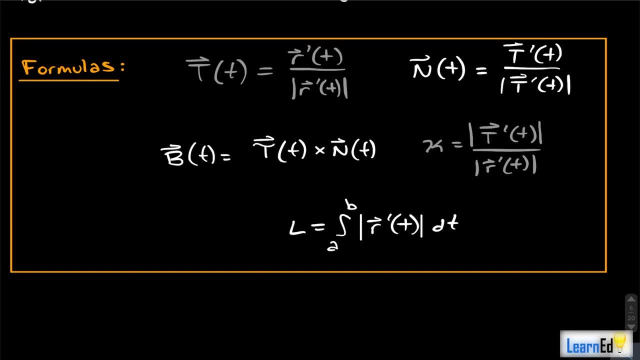 I'm not sure if you'd be given those on a final exam. I assume no. But if you're, You're given like a sheet or something. if you you know you can walk in with a piece of paper. These are definitely formulas you want to put on there. 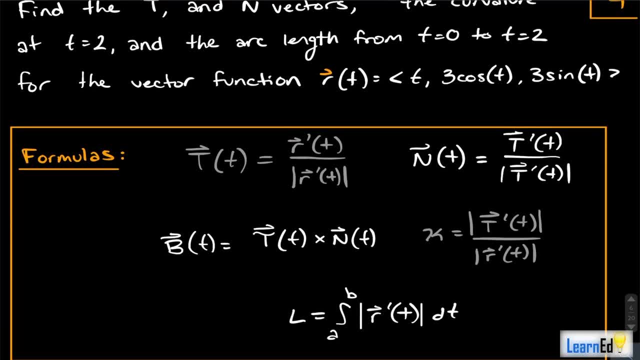 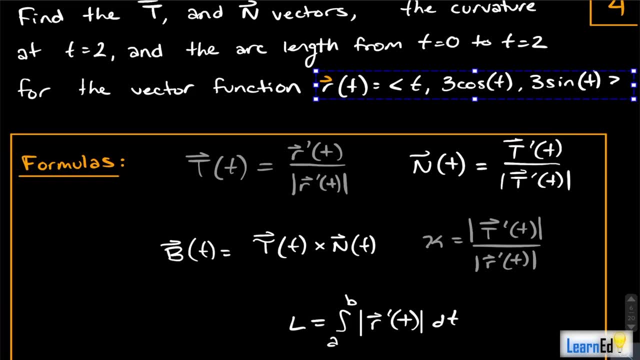 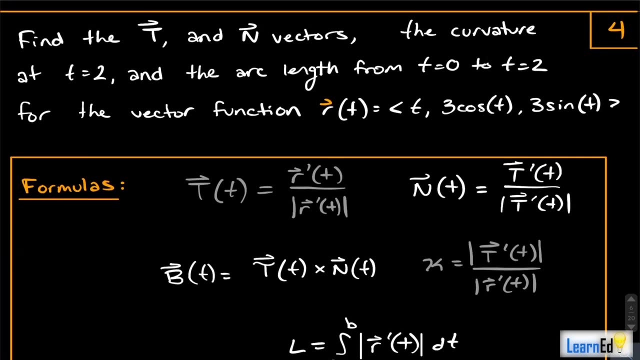 And so let's kind of just get on with this. So if I copy this equation, okay, If I copy this equation down here, we can just start off by finding our unit tangent vector right? That's the first guy we got to accomplish, okay. 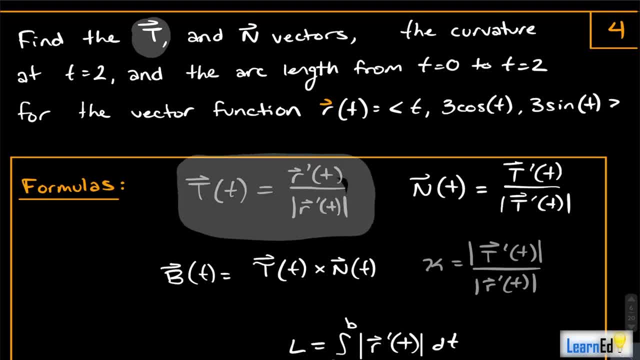 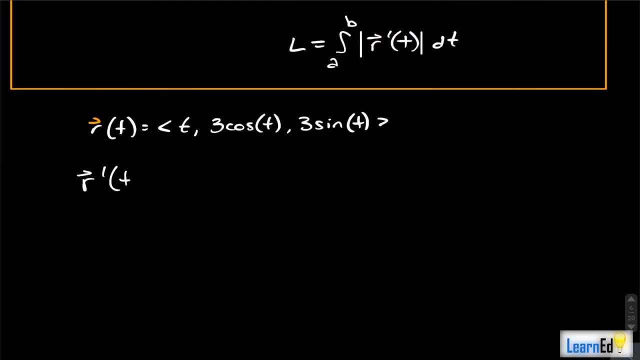 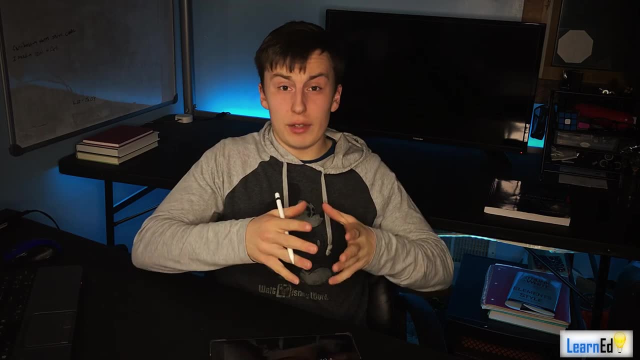 The unit tangent vector is just equal to r prime over the magnitude of r prime. So the first thing that we're going to have to do is find r prime. okay, And how do we take a derivative of a vector function? Well, all we have to do is just take a derivative of each component, right? 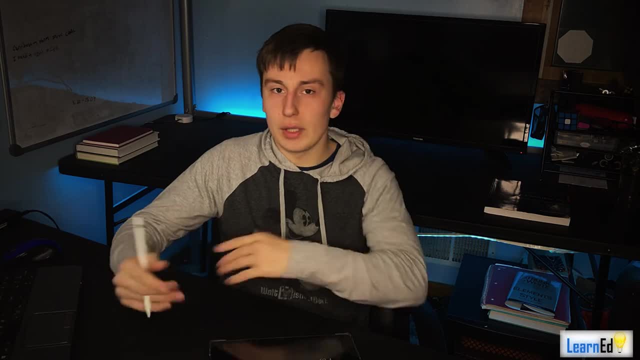 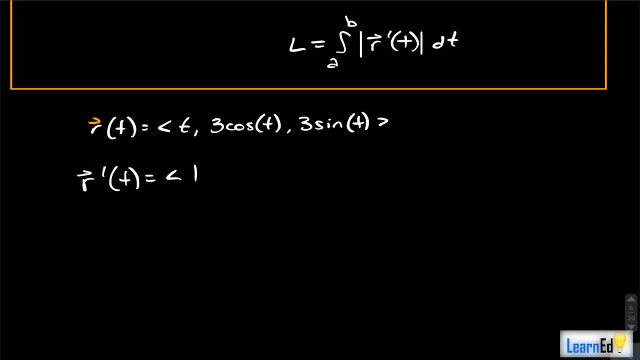 That seems pretty intuitive. We just- you know, it doesn't matter that they're all separated, We just take a derivative separately. okay, So r? prime of t, the derivative of t is 1.. The derivative of 3, cosine t is going to be negative, 3.. 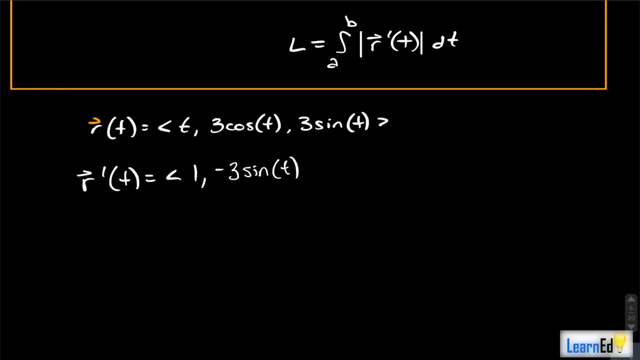 3 sine t and the derivative of 3 sine t is going to be 3 cosine t. all right, Great, We have r prime of t. Now we have to find the magnitude of r prime of t. How do we find the magnitude of a vector function? 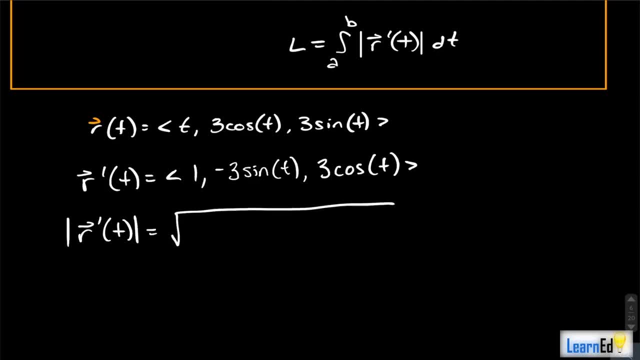 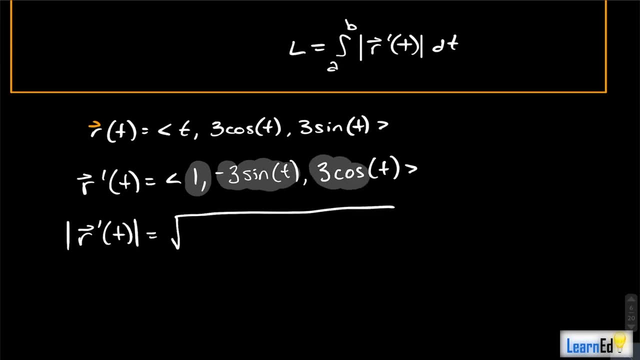 Well, all we have to do is take the square root of the sum of the squares. okay, So we take the square root of the sum of the squares of these guys right here. So we have 1 squared plus a negative 3 sine of t squared plus 3 cosine of t. 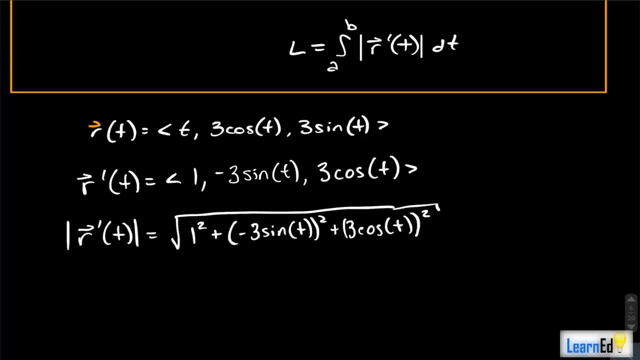 and this whole thing is also getting squared. okay. So we get the magnitude of r prime of t equals now this is equal to the square root of 1 plus 9 sine squared t. So we get the magnitude of r prime of t equals. now this is equal to the square root of 1 plus 9 cosine squared t. all right, 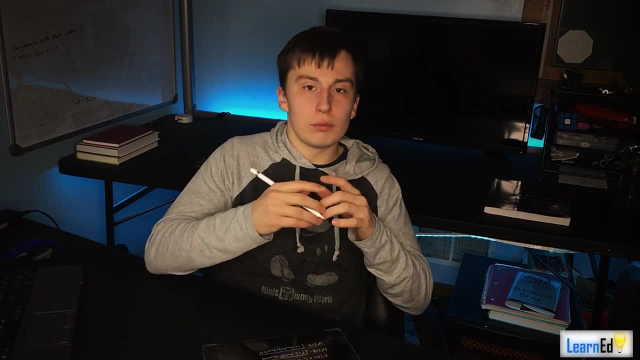 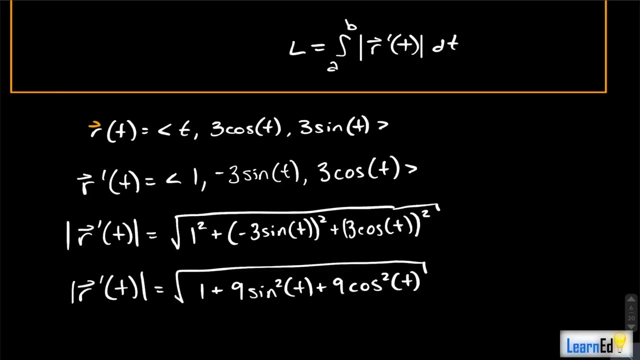 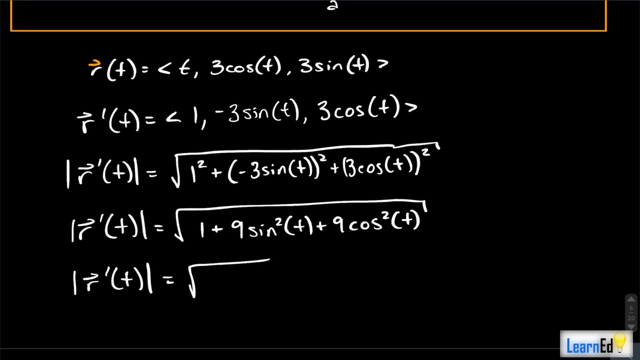 And now what do we do? Well, we know we have a sine squared, a cosine squared. Let's use that Pythagorean identity and just get that over with, and then we'll just have a really nice radical. So we get the magnitude of r. prime of t is equal to the square root of. 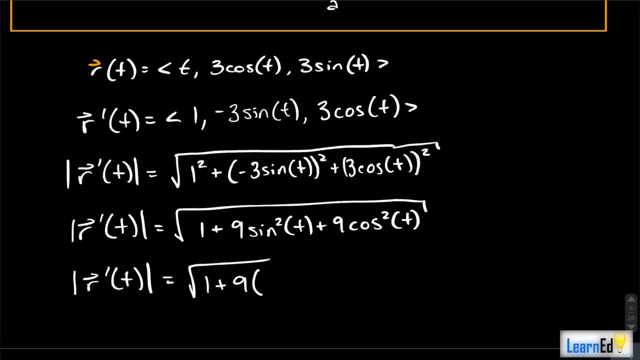 I'll just go the extra step so everybody is on the same page here. We can take a 9 out Of these two terms. we get a sine squared t plus cosine squared t, And that gives us square root of 1 plus 9, which is 10, okay. 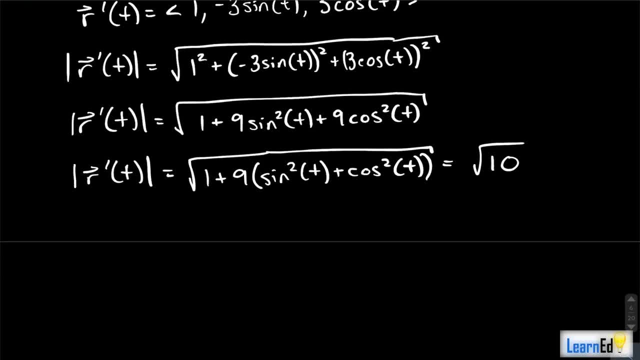 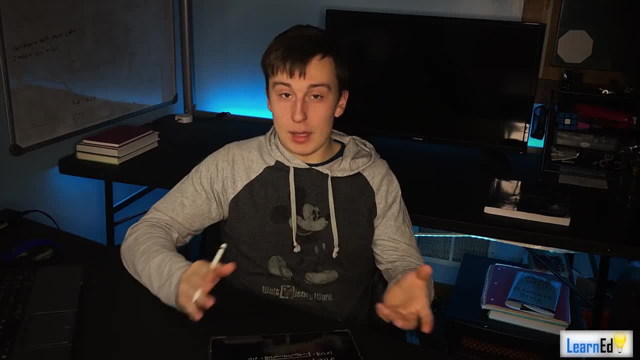 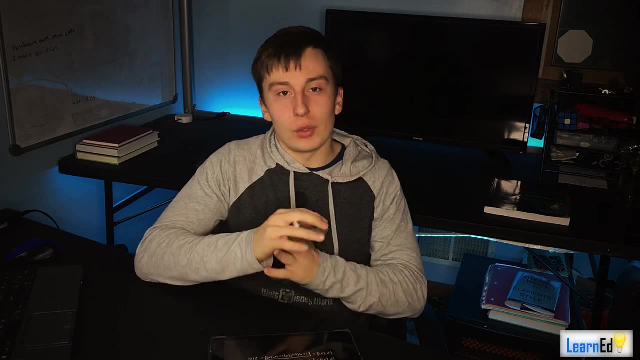 So that is r prime of t and we already have, or sorry, that's the magnitude of r prime of t, which means it's the length of r prime of t, just in case anybody was confused on what magnitude means. I remember our physics teacher always had in my high school physics teacher I mean. 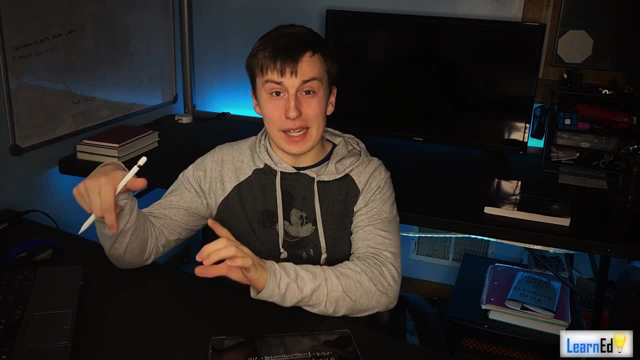 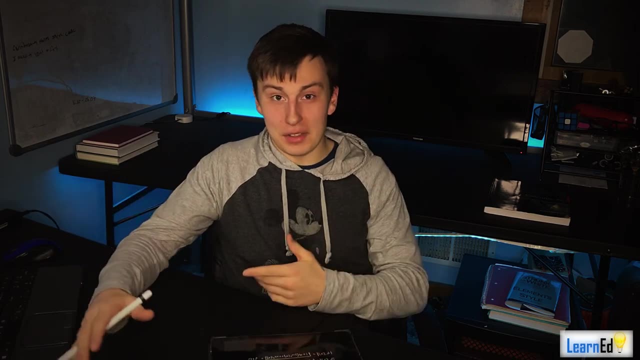 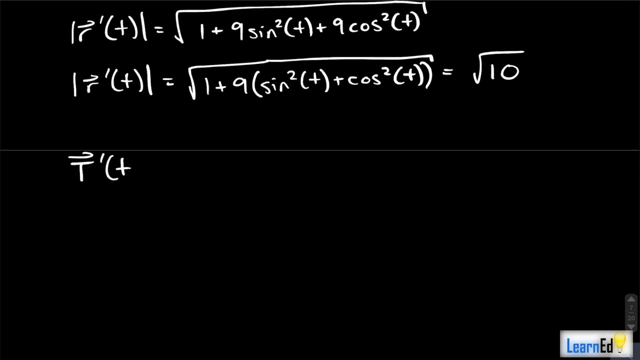 always had a sign up in his room that said magnitude means size or amount. okay, So I may be a little privileged understanding what magnitude meant at a younger age. So, anyways, enough of that. We get that t prime of not t prime. 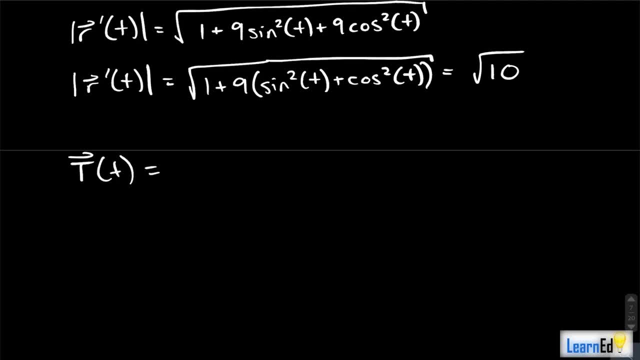 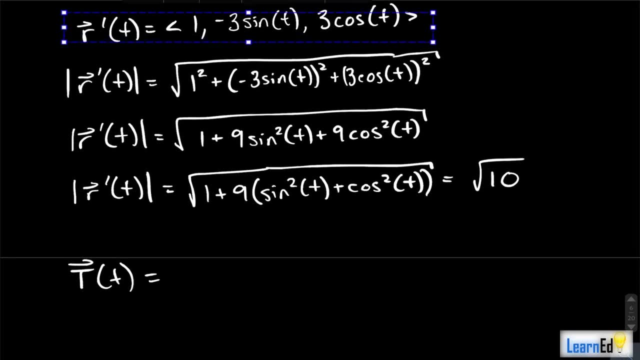 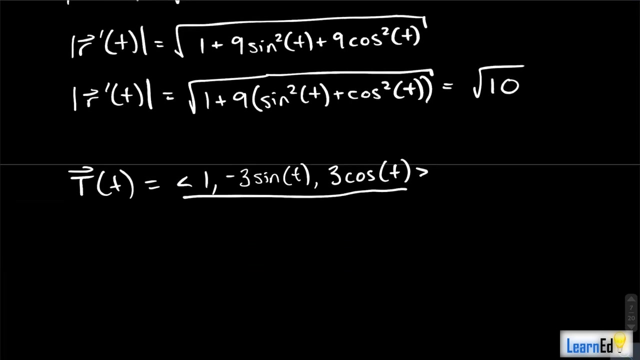 We get that the unit tangent vector as a function of time is going to equal. we have this r prime of t, This guy right here, So let me get this was inefficient, I'll use this guy And I'm going to divide by the square root of 10, okay. 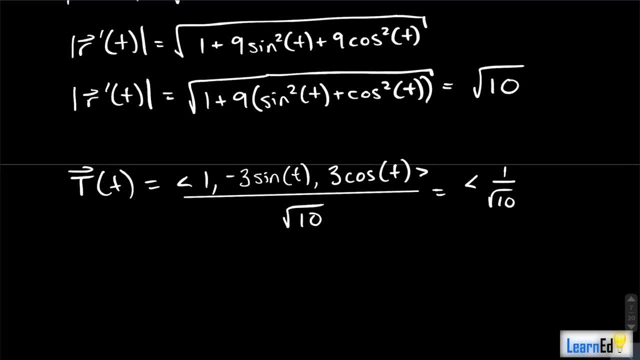 And we get 1 over square root of 10, negative 3 over square root of 10, sine t. And since I don't have enough room, let's move this down here And finish down here, Because this is going to be 3 over rad 10, cosine t. 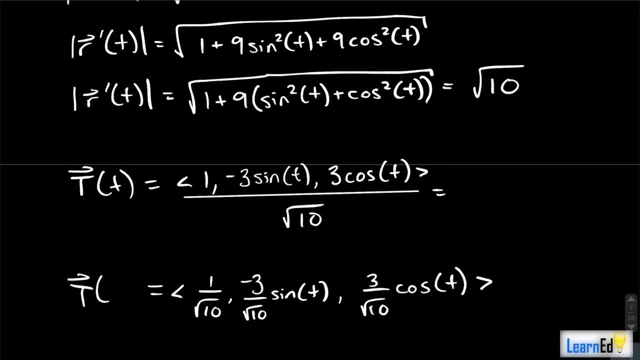 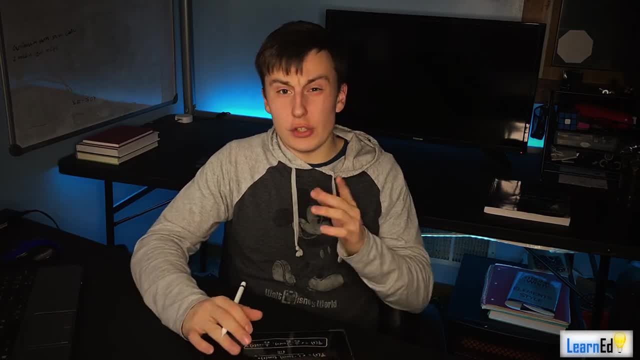 All right. So if that is our finished unit tangent vector, then what is the next thing that we have to find? Well, it is the unit normal vector. So how do we find that unit normal vector? Well, we have to use this equation over here. 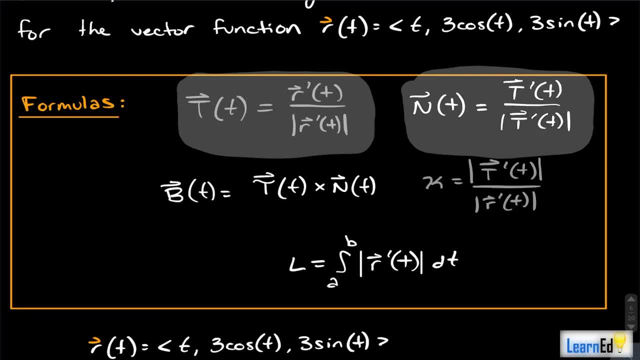 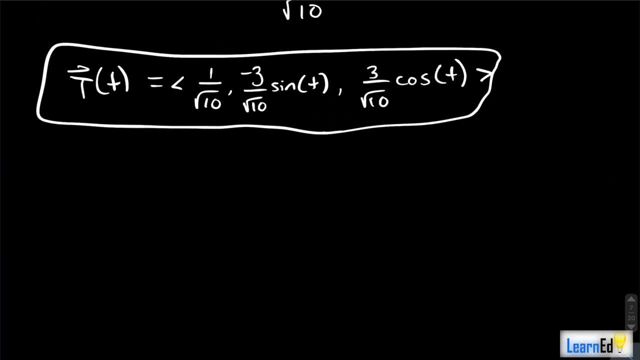 We have just now. we have to use that unit tangent vector. We take a derivative of it And we put that over the magnitude of that unit tangent vector. Okay, So the first step is to find t, prime of t. All right, 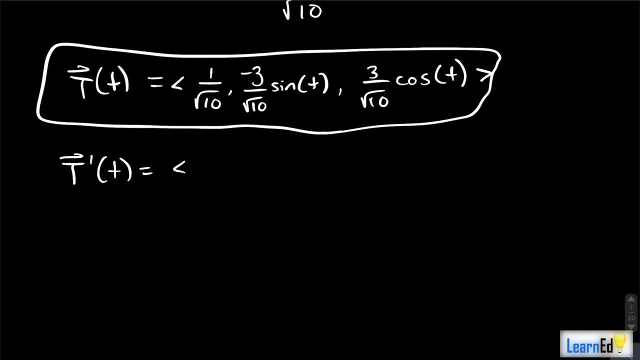 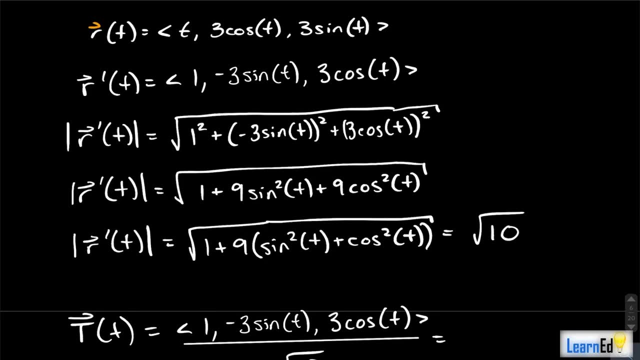 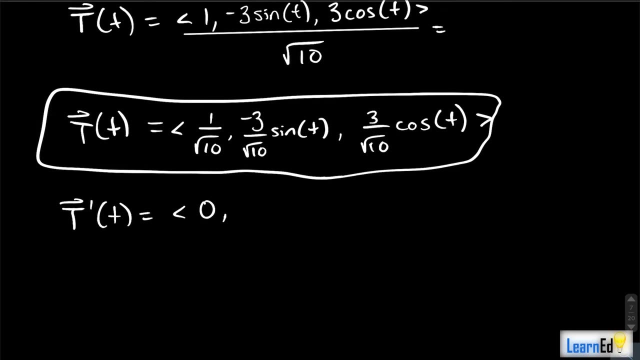 And t prime of t is going to be well. first off, the derivative of 1 over the square root of 10 is going to be 0.. And then we have, we have the derivative of negative 3 sine t over rad 10.. 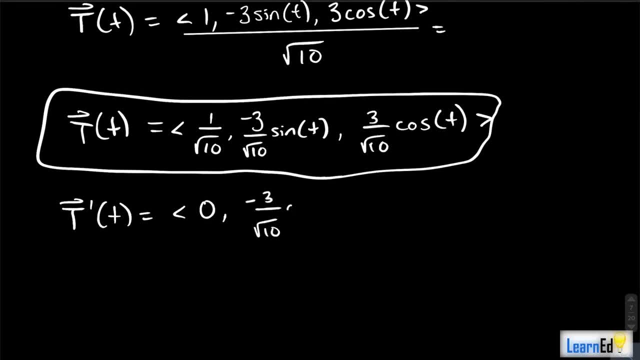 That's going to be negative 3 over rad 10 cosine t. And then we have the derivative of 3 over rad 10 cosine t, which is going to be negative 3 over rad 10 sine t. All right, We are going to put that over the magnitude of t, prime of t. 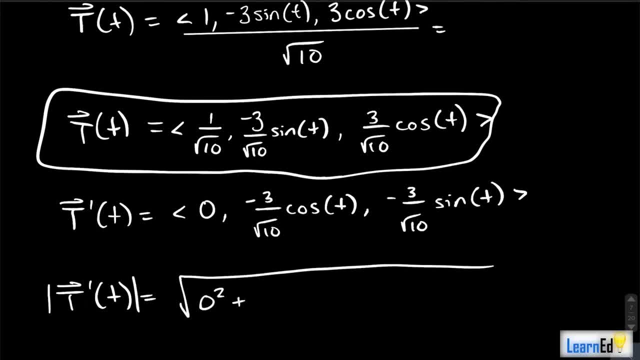 Square root of the sum of the squares, We have 0.. So what's it going to? she't Trying to pelo glass, So here's going to do the derivative. So we're going to typically put it together by any two u's. 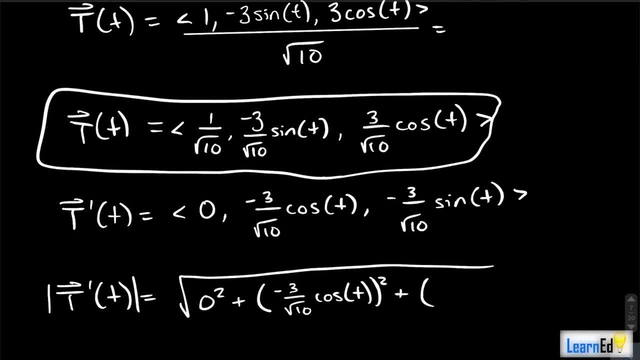 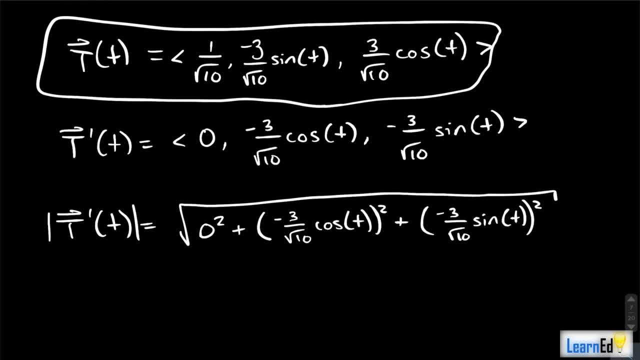 So we got to put this any two u's and then we're going to put it over here. All right, So again, what's going to happen here is that we are going to get the derivative of this cose. Well, of course. 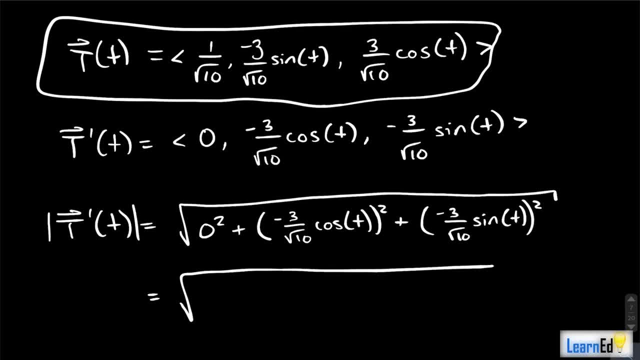 we're going to pull down. So cherry, cherry, cherry, cherry, cherry. Okay, and we'll pull that out and just have a cosine squared t plus sine squared t on the inside. so we get that the magnitude is equal to 3 over rad 10.. okay, so that's the magnitude. 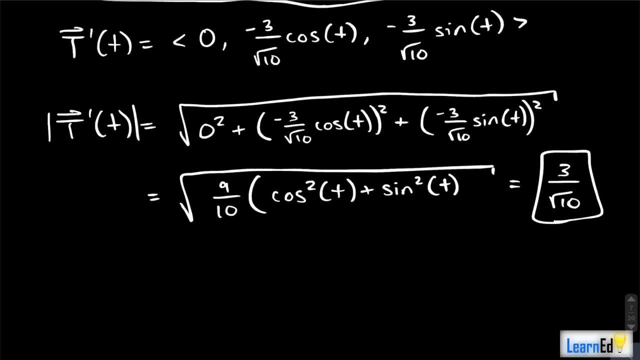 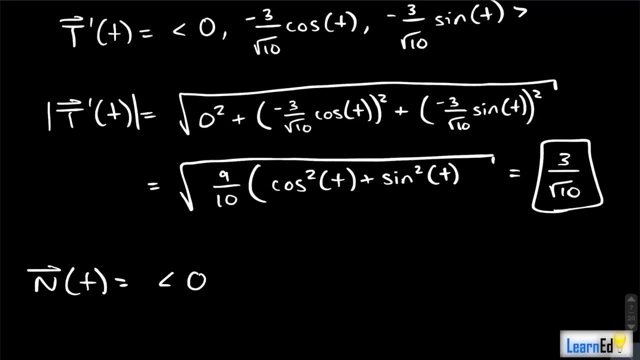 all right. so now all we have to do is put these things over each other. so we have that the unit normal vector is equal to that vector. 0 negative 3 over rad 10 cosine t, negative 3 over rad 10 sine of t, and that's going to be all over. 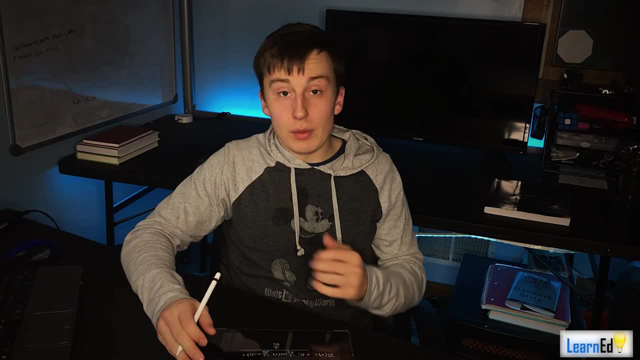 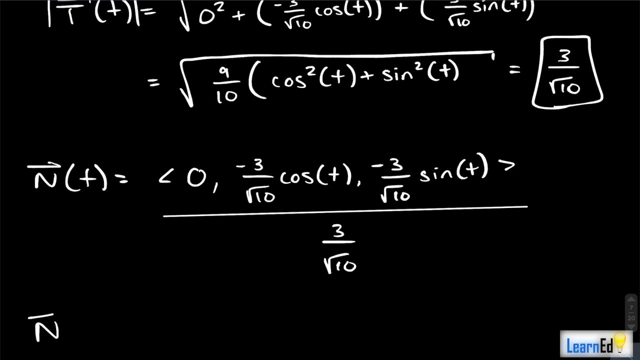 3 over rad 10.. all right, so now you see that we're going to get some really nice cancellations here and we will wind up with a nice unit normal vector that is just going to be 0 negative cosine t and negative sine of t. 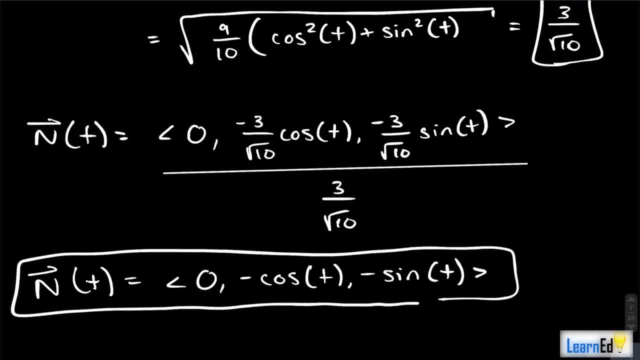 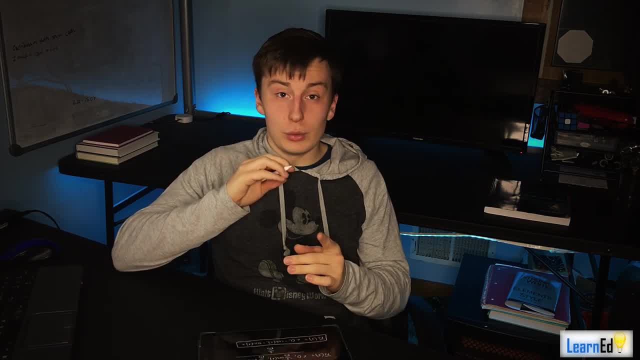 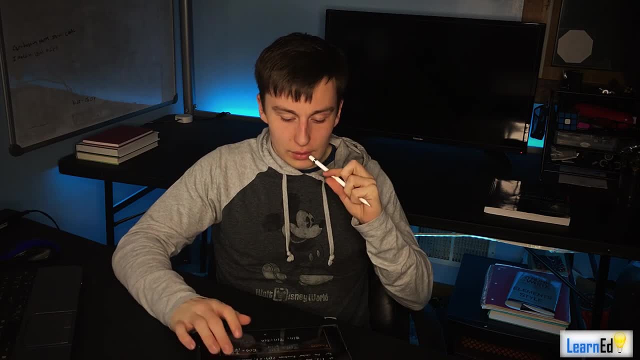 all right, that right, there is your unit normal vector. okay, so we have two out of the four things that we need to find now. we just got to move on to curvature and we also have to find what was the other thing we have to find. we have to find the arc length and the curvature. okay, so the first thing we're going to find is the. 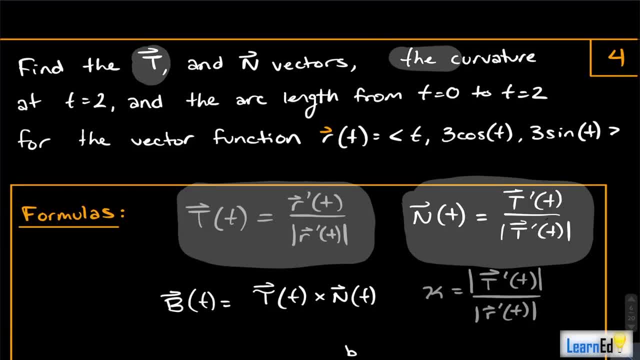 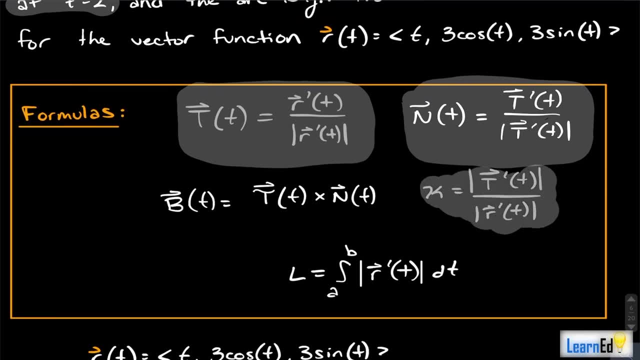 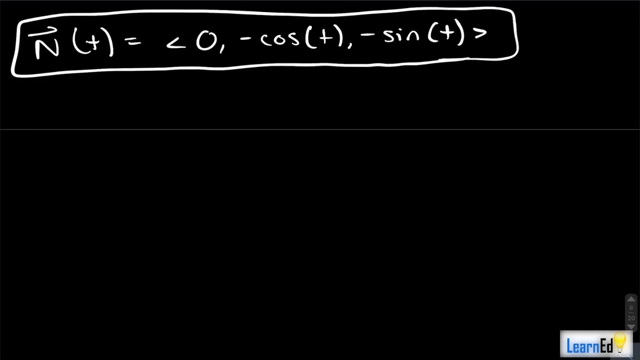 curvature. okay, we need to find the curvature at t equals 2. the equation for the curvature is the magnitude of t prime of t over the magnitude of r prime of t. okay, and remember, we're finding the curvature at t equals 2.. okay, so curvature. 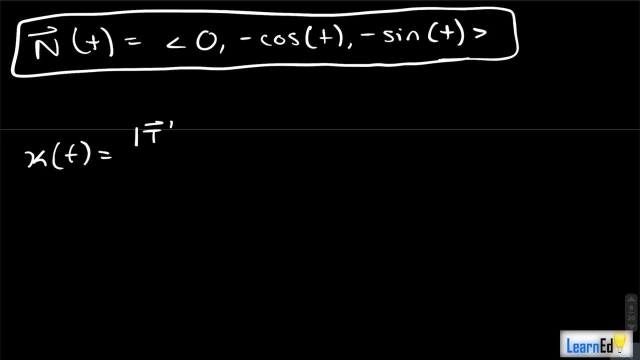 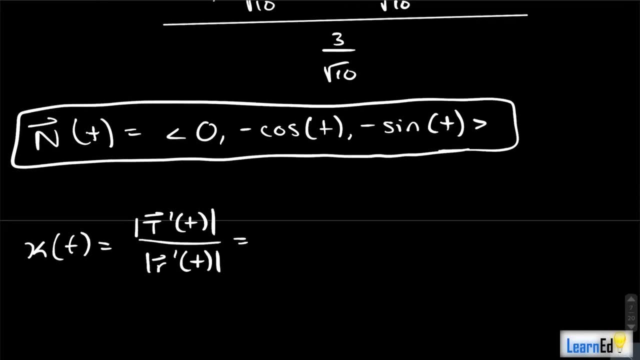 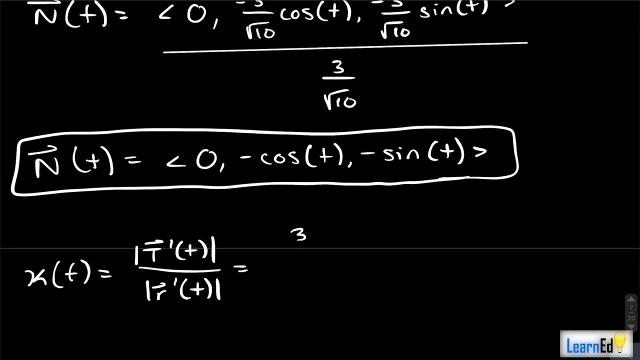 of t equals the magnitude of t prime of t over the magnitude of r prime of t. now, what was the magnitude of t prime of t? it was this quantity right here, right that 3 over rad 10. so we'll put that right over here: 3 over rad 10. and then, what was the magnitude of r? 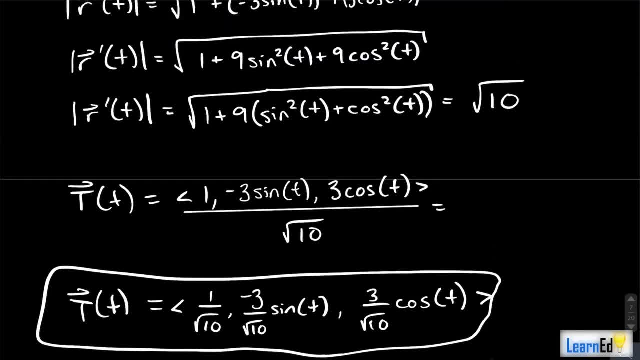 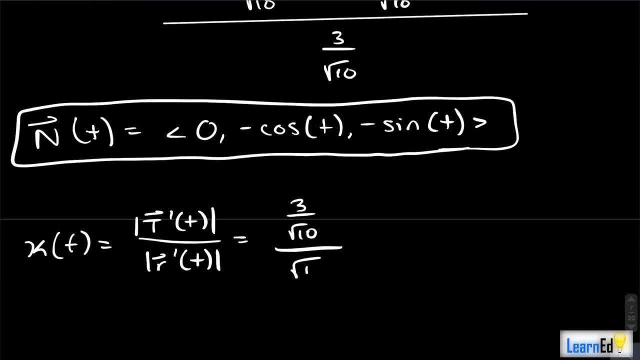 prime of t. we've already found these things right, so it's just, it's just a plug and chug from here. the magnitude of r prime of t was rad 10.. So we're gonna put that down. it says rad 10, so we're gonna put that down here and we're just gonna wind up this very, these rad10s are gonna. 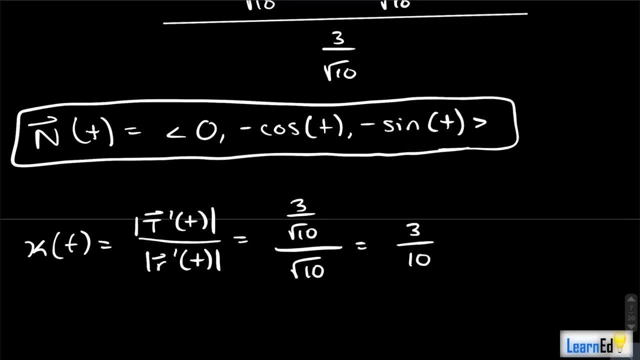 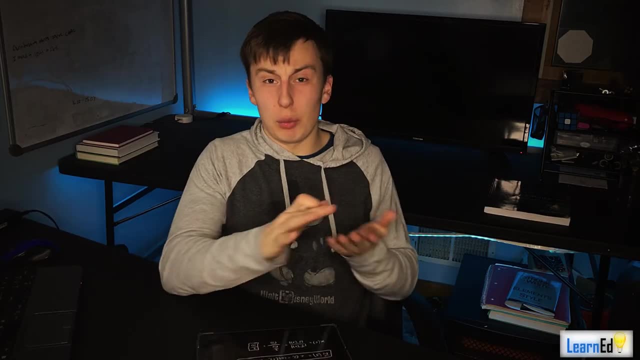 get multiplied together. okay, don't think that they get cancelled out, because this bottom rad 10 is not in the denominator of the denominator. so anyways, we get 3 10ths. so that is the, the, the curvature, and that's not even that's gonna be the curvature everywhere. that's not just the curvature. 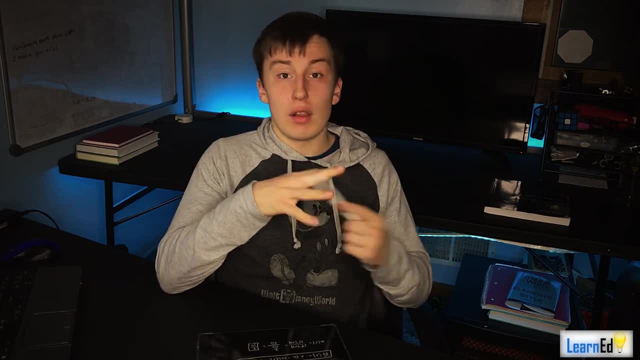 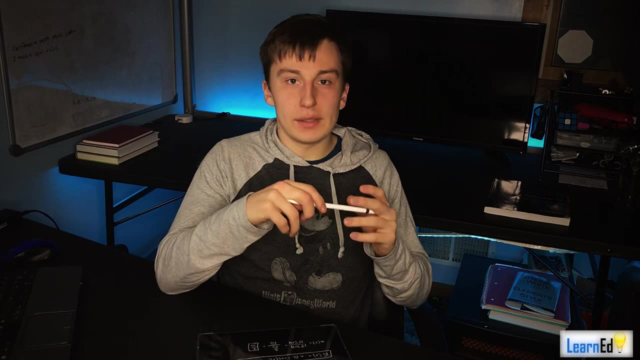 at t equals 2, that's the curvature, and b1 at the bottom in the primer 6.. now, if you're gonna do some everywhere, because that thing wasn't even dependent on t, right, the magnitudes didn't have any variables in them. that stayed through, okay, and the reason for that being, by the way, 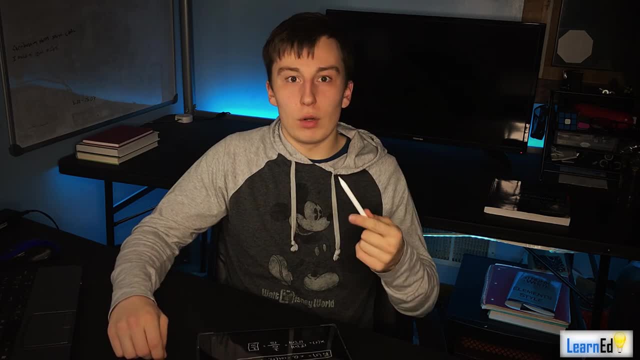 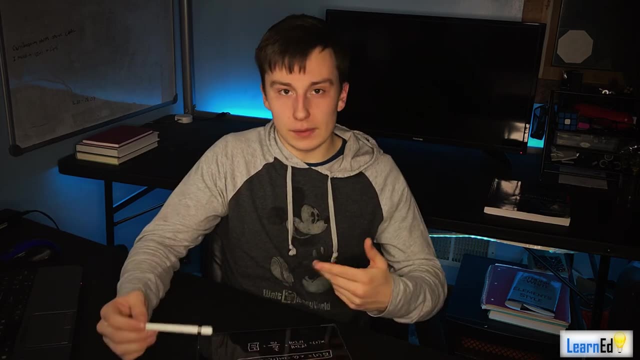 is because we had the. the only things we had that would have contributed is like the cosine t and the sine t, and those went away with that trig identity that we used. so that's why we don't have any variables in the curvature. last thing we got to find here is the arc length and then 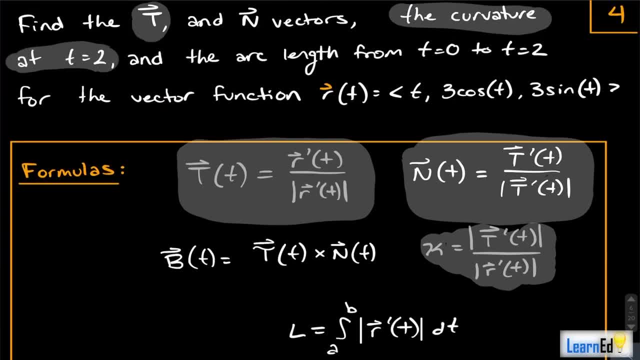 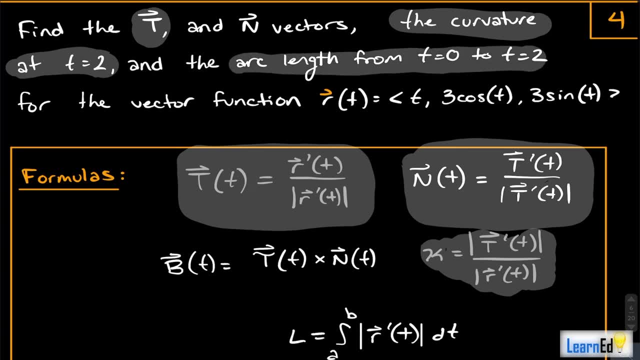 i'll let you guys take a break, a five minute break preferably. that's probably going to be best for y'all. um, that's what i would do. at least we got to find the arc length from t equals zero to t equals two, and we got to use this formula right here. okay, the arc length equals the integral. 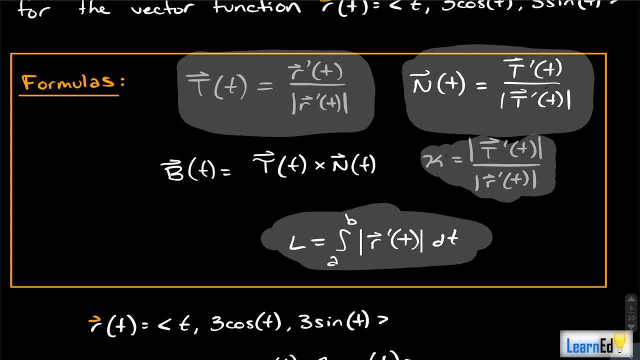 from a to b of r, prime of t, dt, and that's the magnitude of that. so i'm going to copy this, okay, and you guys can jot that down real quick. that's going to be the formula that we're about to use you. okay, we are going to go, bam bam. 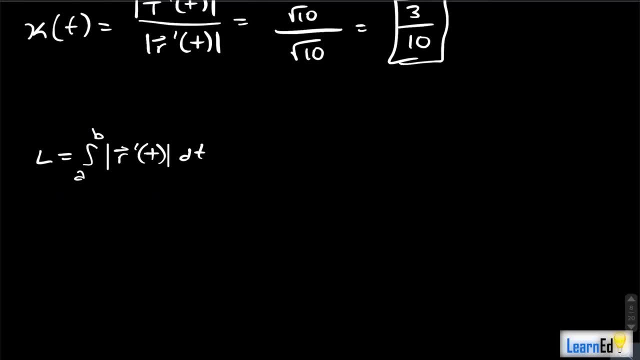 okay, um, yeah, so we're taking the integral from zero to two. what is that magnitude of r prime of t? that, uh, the magnitude of r prime of t is just rad 10. so we have the. we have rad 10 dt. okay, so when we integrate here, we get t rad 10. 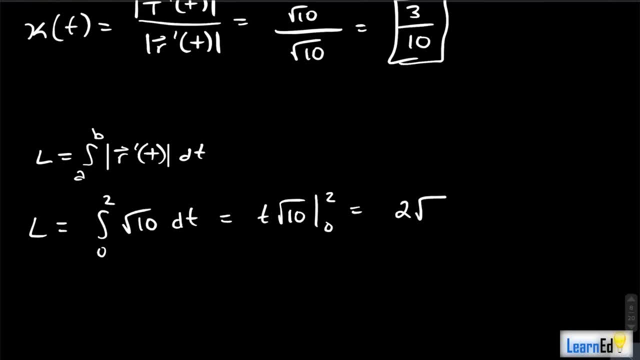 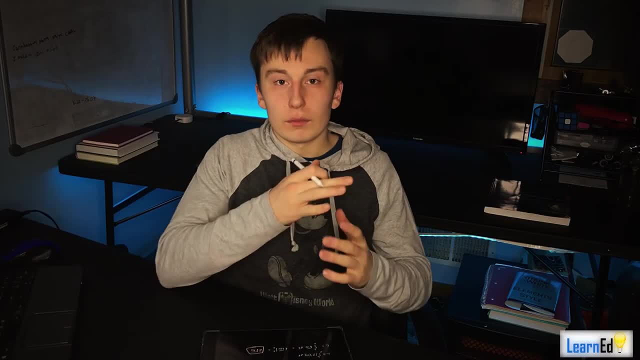 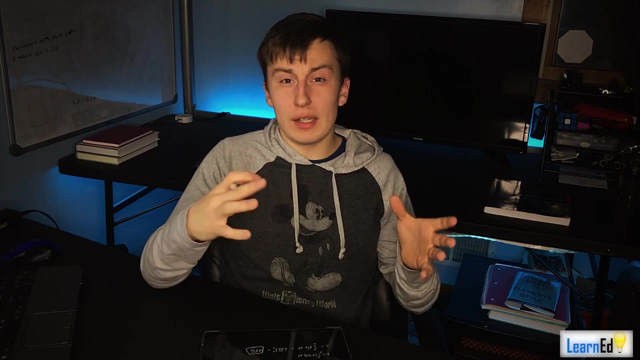 evaluated from zero to two and we just get to rad 10, is our arc length from zero to two. okay, so that's kind of like all the intro stuff, that. um, that's all the problems i'm gonna do on the intro stuff that we kind of did before. partial derivatives: okay, because 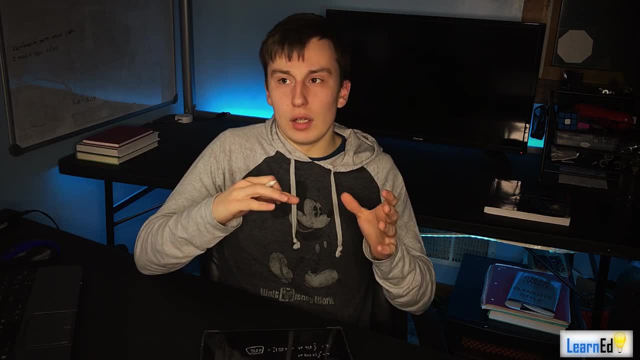 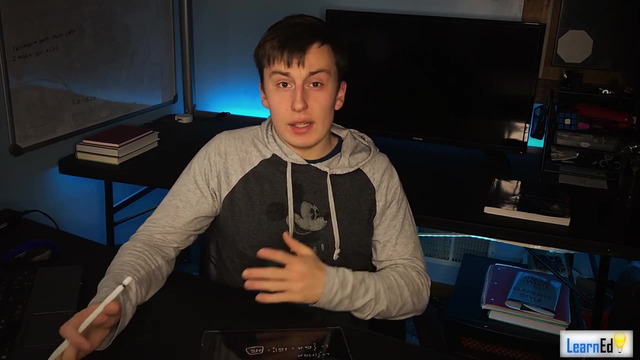 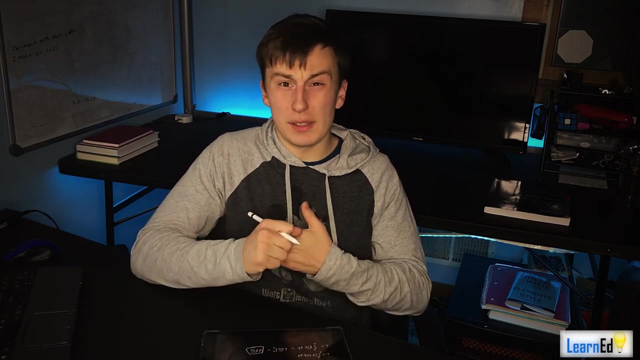 your final is probably going to be a lot more focused on partial derivatives and um, multiple integrals and vector calculus. at least mine was. mine almost didn't even touch on anything except for vector calculus. it touched on a little bit like lagrange multipliers and max and mins and 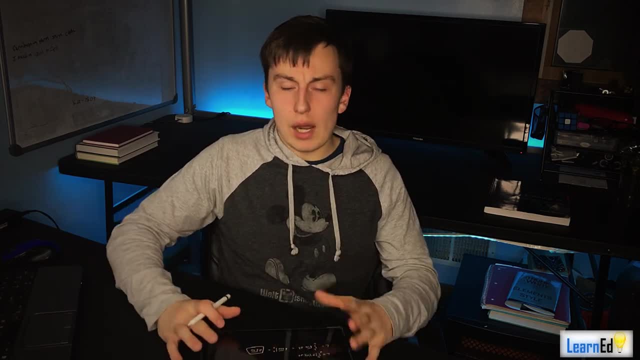 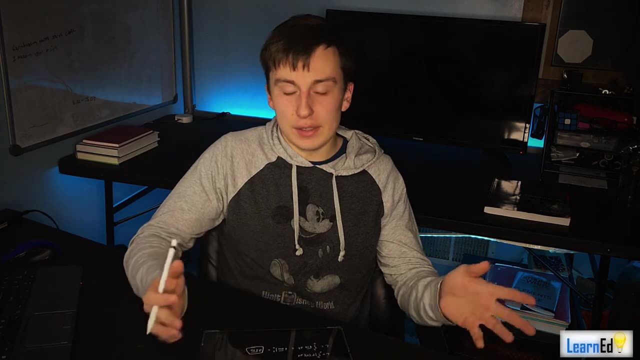 stuff like that, but really it was a lot of vector calculus so i'm not going to spend too too much time on these, like earlier problems that you learn in, like the earlier times of calculus 3. okay, so moving on, we're going to get right into some partial derivative stuff here. 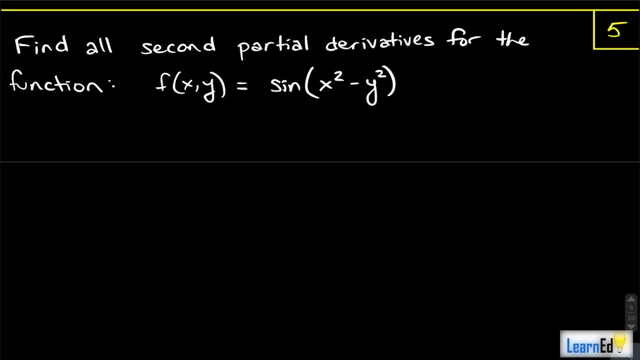 all right. so for number five, we want to find all the second partial derivatives for the function f of x. f of x and y equals sine of x squared minus y squared. okay, so we're finding the second partial derivatives. okay, so the first thing that we'll have, we'll have to do to get to this goal. 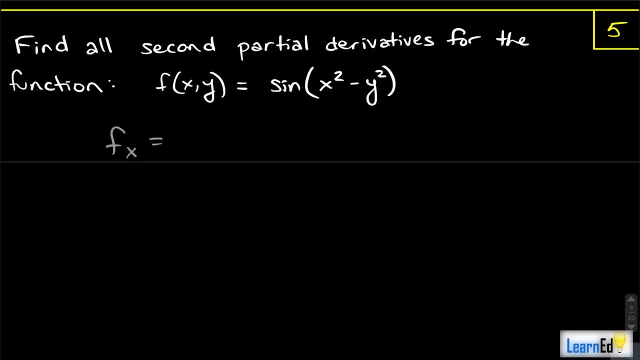 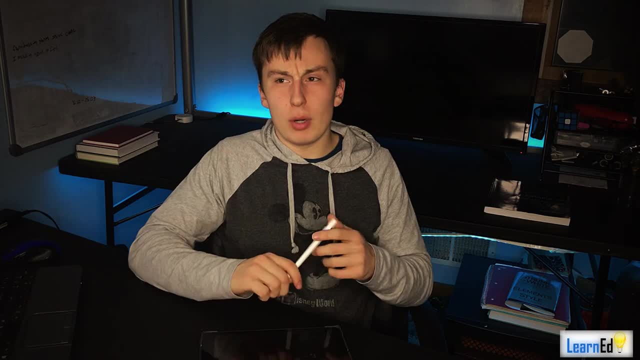 is to find the partial with respect to x and the partial with respect to y. okay, so we're going to find the partial with respect to y and the partial with respect to y. so just the first partial derivatives. now, how do we take a partial derivative? and actually, before we 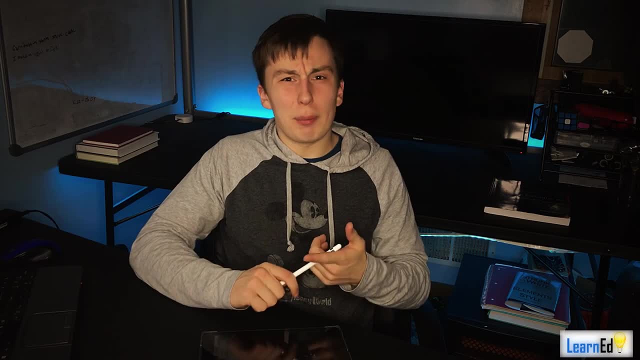 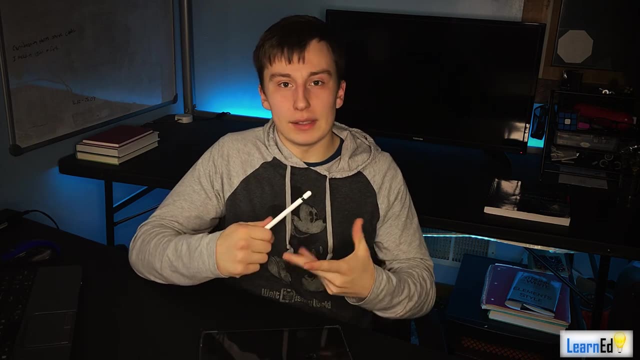 even, uh, talk about that. what is a partial derivative? what is it actually telling us? right, a lot of people learn partial derivatives, derivatives, but they don't know what it means. okay, if you're taking a partial derivative, let's say you have some surface. okay, some surface in. 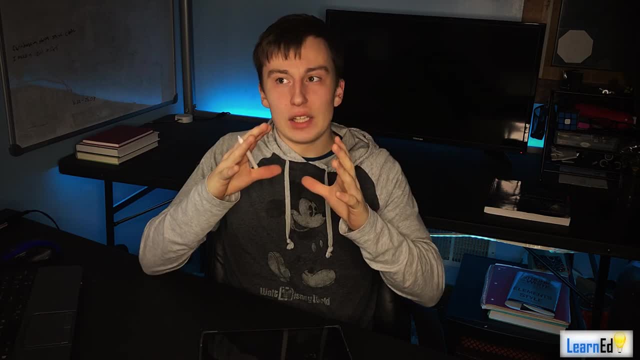 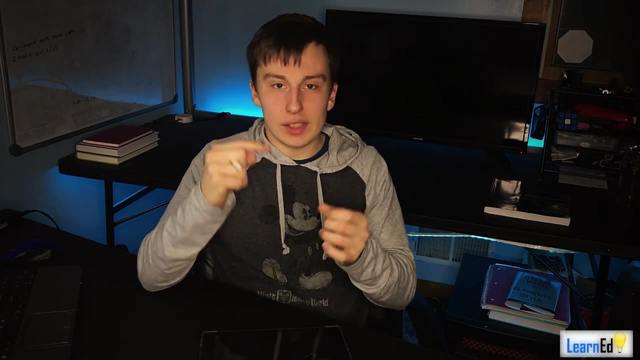 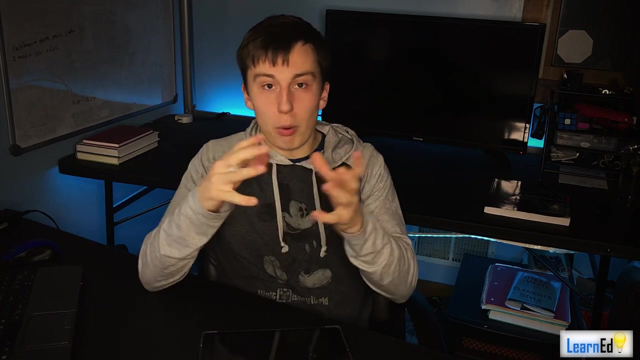 three dimensions. okay, just picture it. okay, and you're taking a partial derivative with respect to x, all you're doing is finding the slope in the x direction, in the, in, in a certain direction, right, the, the x direction. for any point that you're at on that surface, you're able to find the slope in. 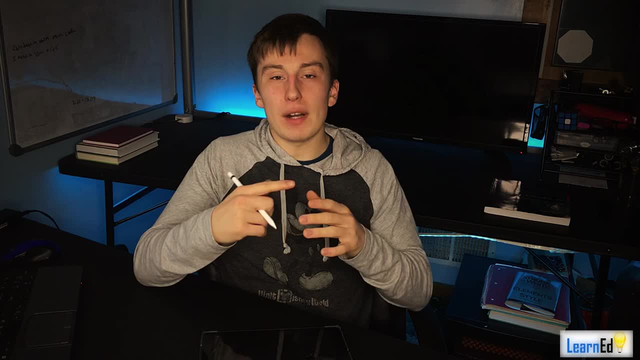 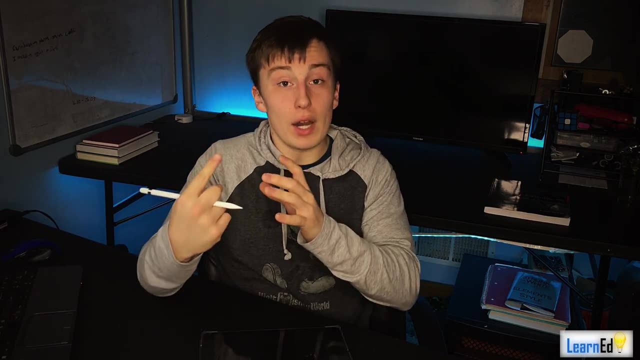 the x direction. you're finding a partial derivative with respect to y. you're finding the slope in the y direction. okay, because there's you know infinite many directions on the surface. you're finding it in the y direction at any point. okay, when we get into directional derivatives, it's a little bit. 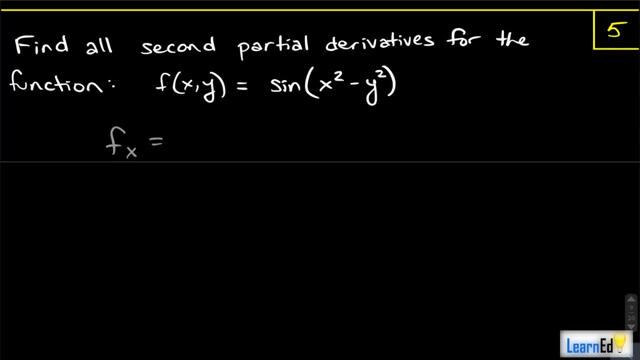 different. okay, so you know, then it's any direction. but anyways, for now those are partial derivatives, so we're finding the slope in the x direction for this, this surface that we have here. okay, we have the partial derivative, uh, with respect to x here, where we know that the inside 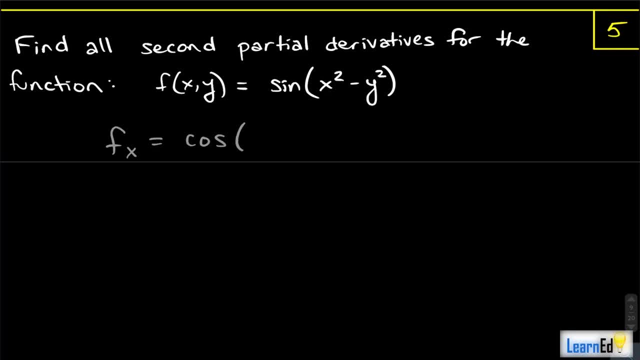 of this is just going to change, or sorry, the. the outside of this is just going to change to cosine of x squared minus y squared and the derivative of the inside with respect to x. so we're going to: the y squared goes away, we just have a 2x, so i can actually just move that out front. 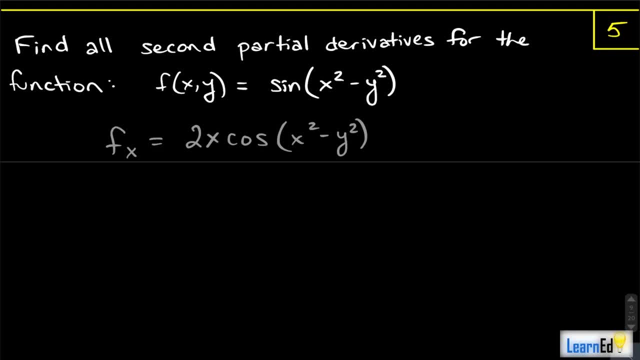 and we have 2x cosine of x squared minus y squared. now for the partial with respect to y. we have. well, we have again. we're going to have cosine of x squared minus y squared, but the derivative of the inside is now negative to y. okay, 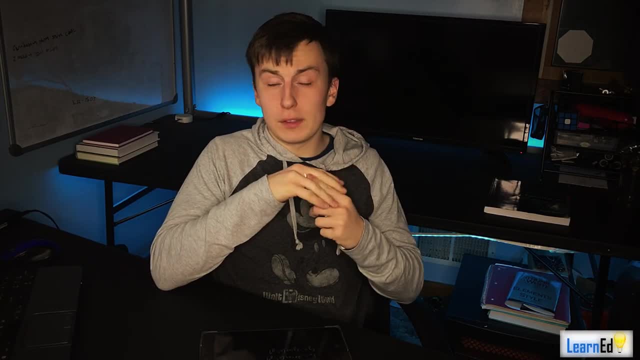 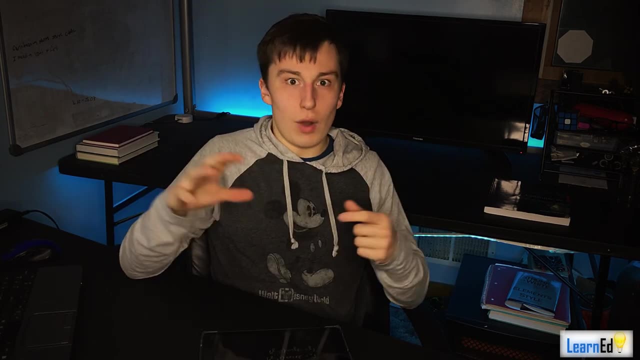 okay, and that's the whole thing with partial derivatives. right, if you're taking a partial with respect to x, you're treating y as a constant. so when we were taking the derivative of that inside, with x squared minus y squared, the y's just just treated like a constant. so it's like 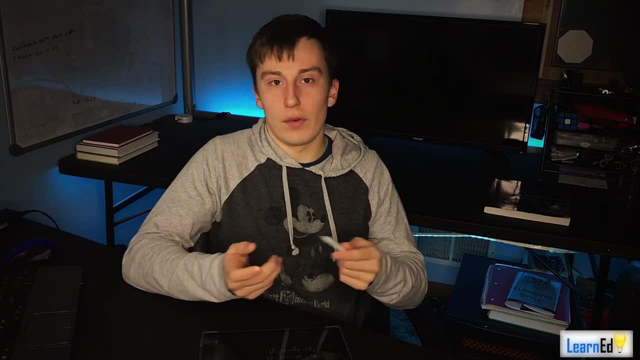 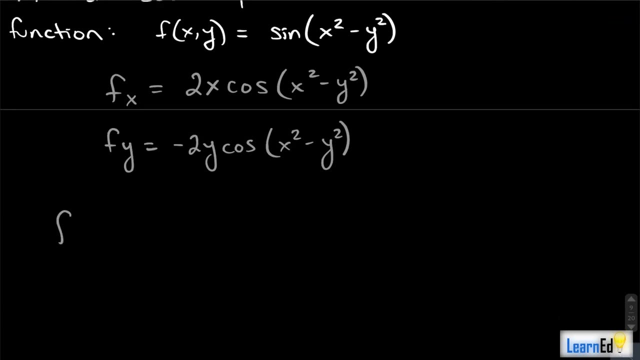 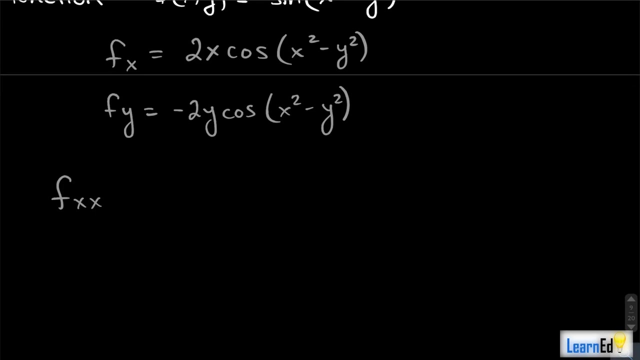 x squared plus two, the two goes away. all right, it doesn't matter, worthless, okay. so that's the first derivatives. now we got to find the second derivatives, which, If you remember, our Fxx, Fxy, Fyx and Fyy. So, first off for the partial derivative, so the second partial derivative, actually, I'm not sure how to say this. 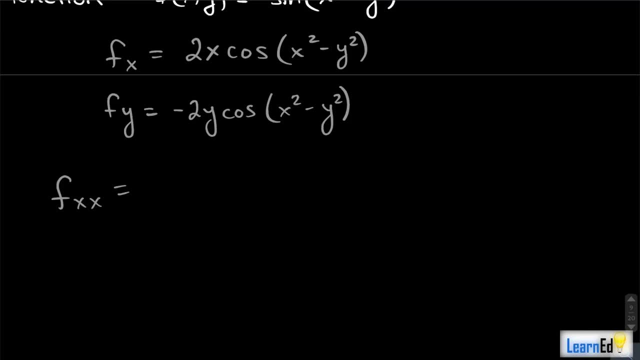 Let's just go Fxx, alright, So to find that we just take another derivative of this with respect to x, And what that is going to be is some product rules. So first we're going to start off by taking the derivative of this, 2x, and dragging along the cosines. 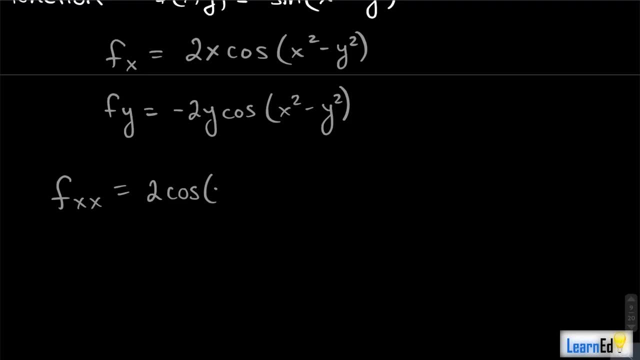 So we get a 2cosx²-y² And then we're going to have the derivative of this cosx²-y² times 2x. So the derivative of cosx²-y² is going to be negative, Negative 2x. sine of x²-y² right. 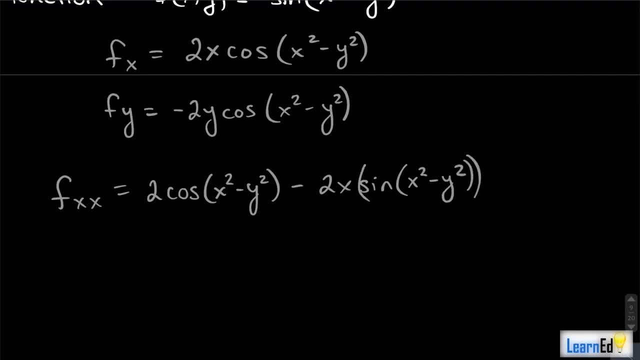 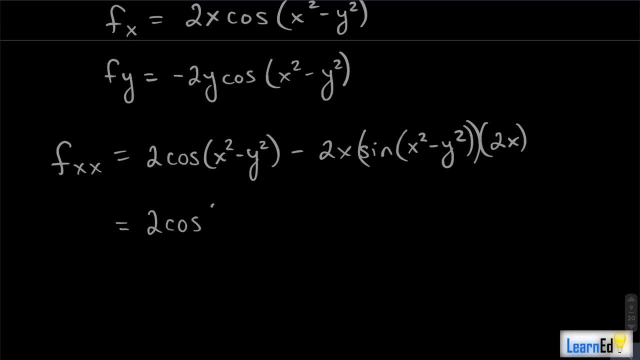 The negative comes from the cosine converting to a sine, And we're going to multiply that by the 2x that straggles along, So simplifying that we get 2cosx²-y² minus 4x² sine of x²-y², right. 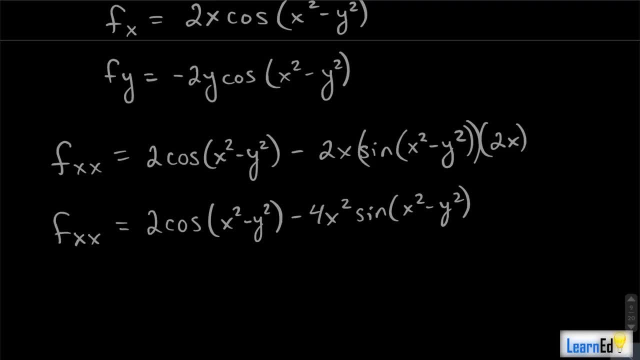 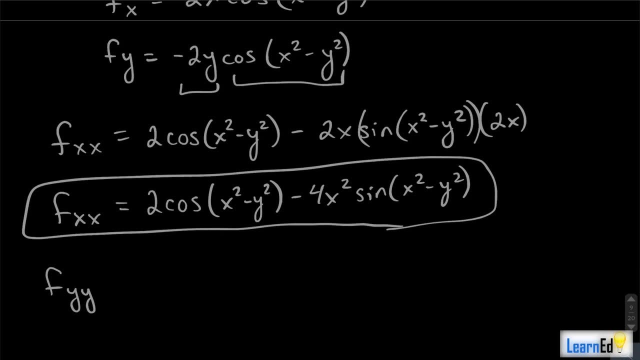 That's your partial derivative, But your second partial derivative of x. Now for the partial derivative, the second partial derivative of y. what we are going to do is just take another partial with respect to y, of fy. So we take a derivative of cosine, of, actually. no, let's do that. 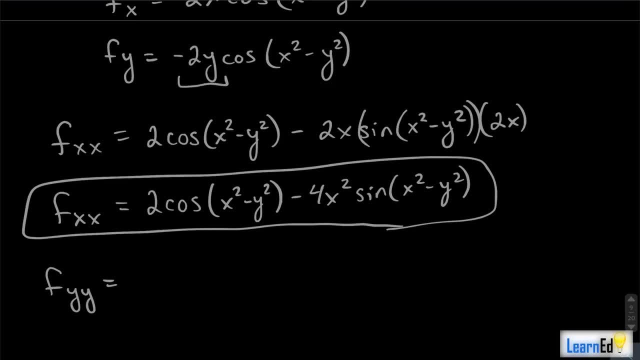 Let's keep the consistency here. We'll take a derivative of negative 2y first And we'll get a negative 2 times cosine of x²-y². okay, And we're going to add on the derivative of cosine of x²-y². 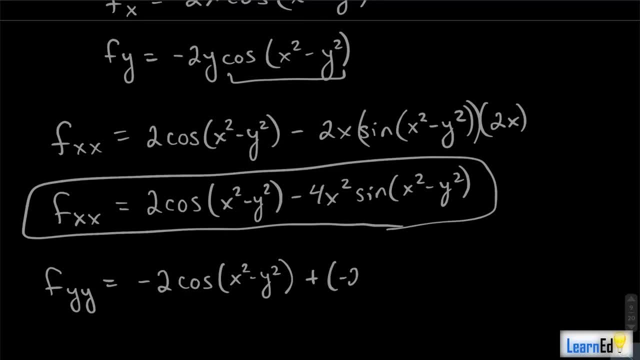 which is going to be first off. we'll have a negative 2y, which is the derivative of the inside times negative sine of x²-y², And then we have it all multiplied by a negative 2y. Okay, 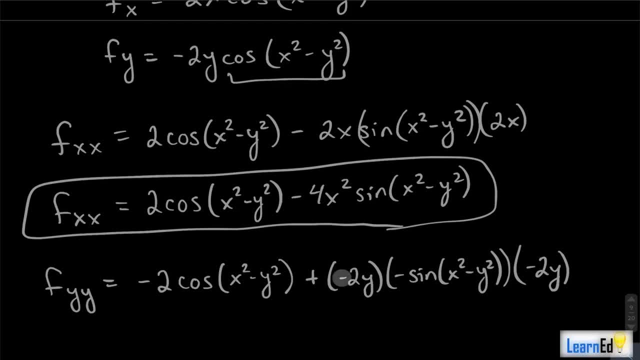 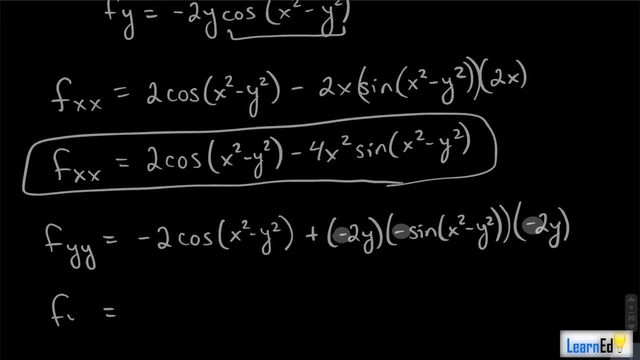 Okay, We have three negatives here: one here, here and here. okay, And so that is going to give us. when we simplify this, we get negative 2cosx²-y² minus a 4y² sine of x²-y². 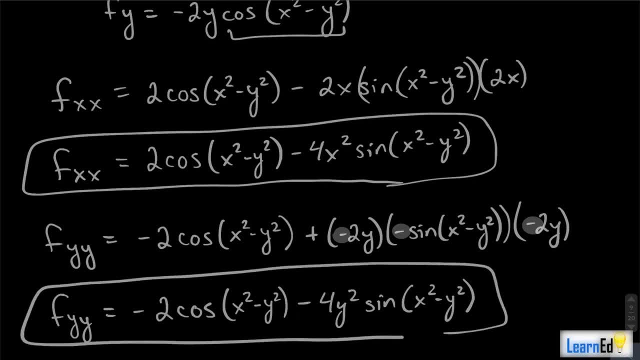 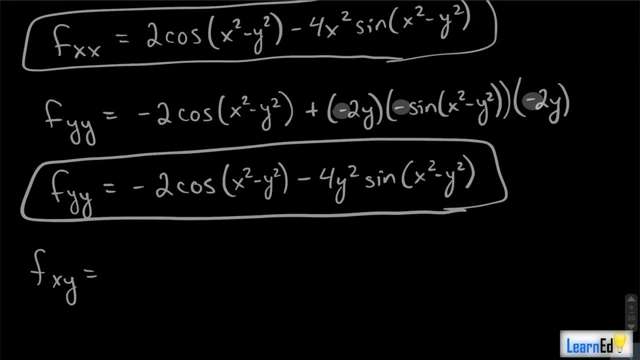 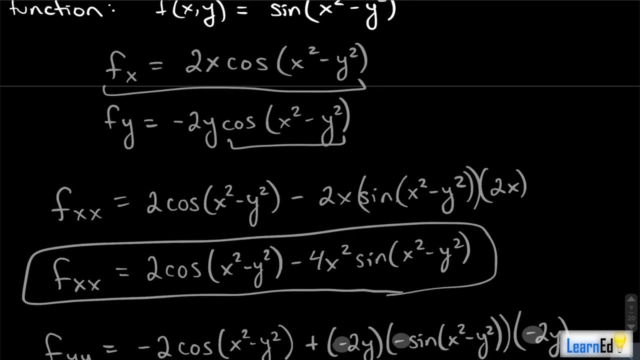 And that is fyy. Now for fxy, all we have to do is take a partial of fx- this guy over here with respect to y, okay, So all that's going to happen is: since this, we don't have to do product rule, because this 2x gets treated like a constant. 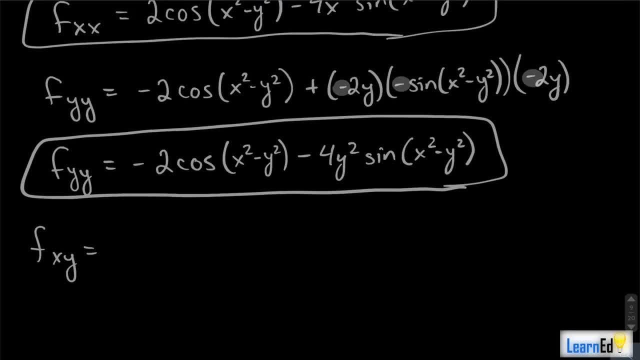 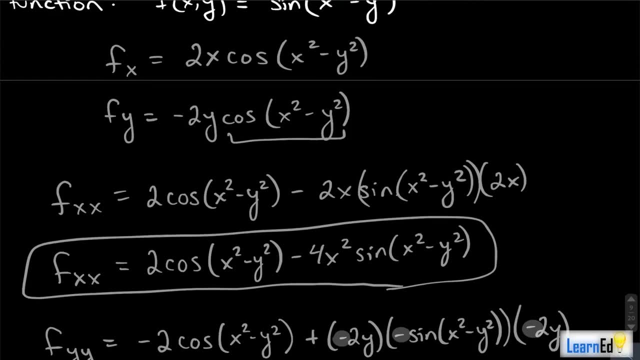 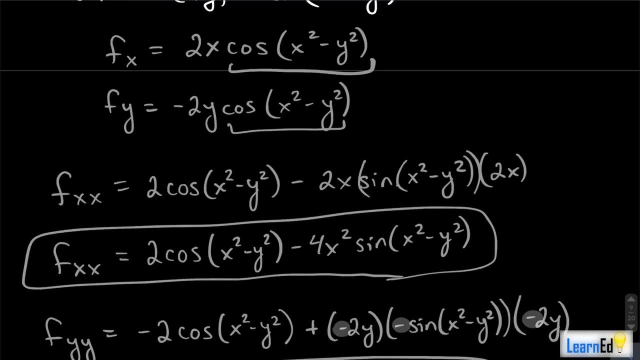 And what we're just going to have is 2x times the derivative of negative y². the inside function is negative 2x. So we're going to have negative 2y. so I'll bring that out And then we'll convert this whole cosine of x²-y² to negative sine of x²-y². 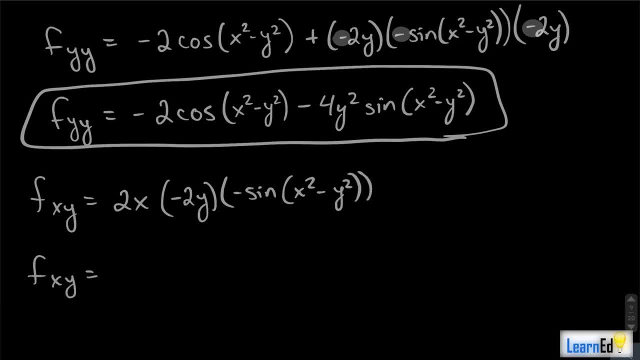 So we get our fxy is equal to negative 4xy, And actually, since there's two negatives here, we're just going to make this a positive. So we'll have 4xy sine of x²-y², All right. 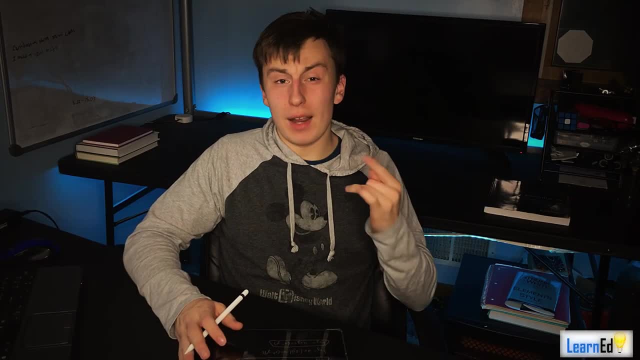 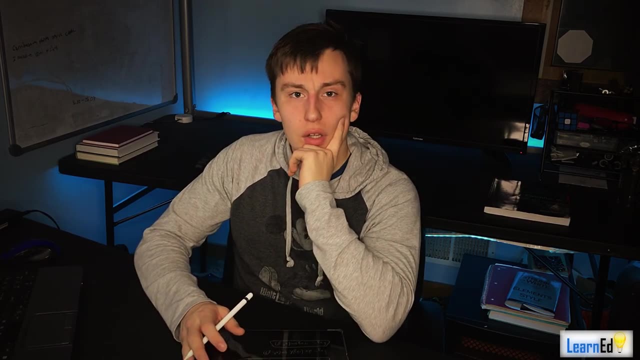 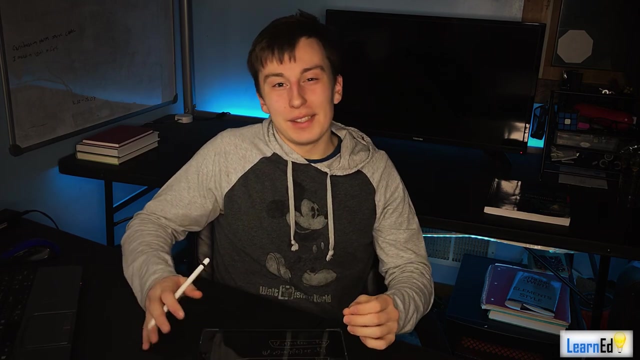 Now for the last partial derivative. fyx, we actually already have it. And well, how do we already have it? Well, there's this thing called- well, I'm not really sure. I hope I don't butcher this name too hard- but Clareau's theorem, okay. 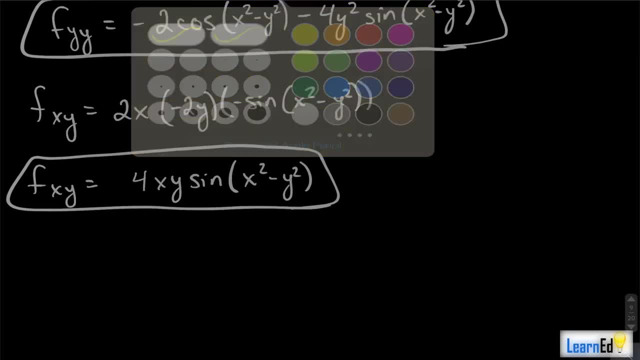 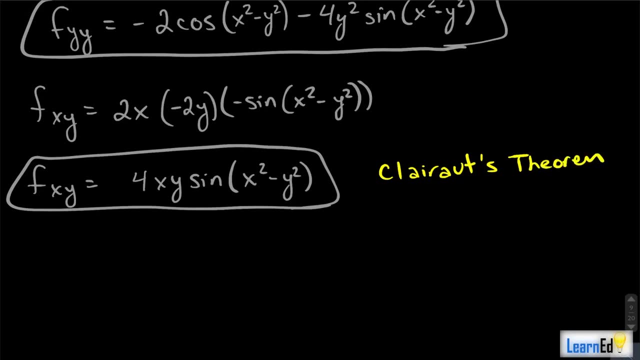 And I'll write that So you can all see exactly what I'm talking about and maybe the name. But looking at it will jog your memory a little bit more than hearing me say it. Clareau's theorem is that fxy equals fyx. 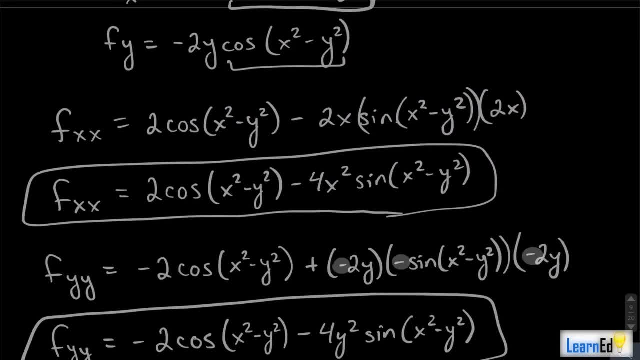 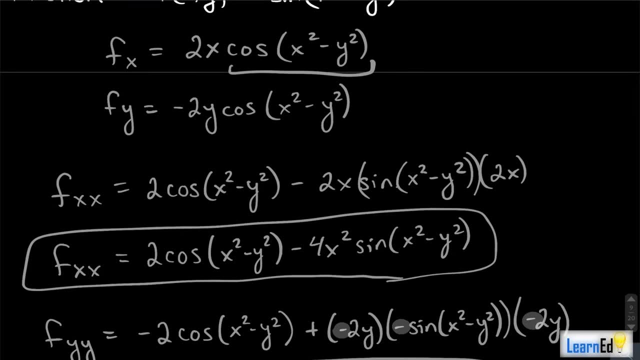 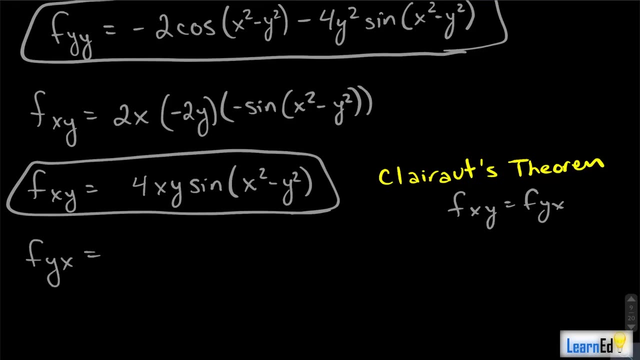 So, sure enough, we took a derivative of a partial derivative of fy With respect to x. we would get the same thing. But we don't have to do that all work, because we can just cite Clareau's theorem and get that fyx equals fxy. 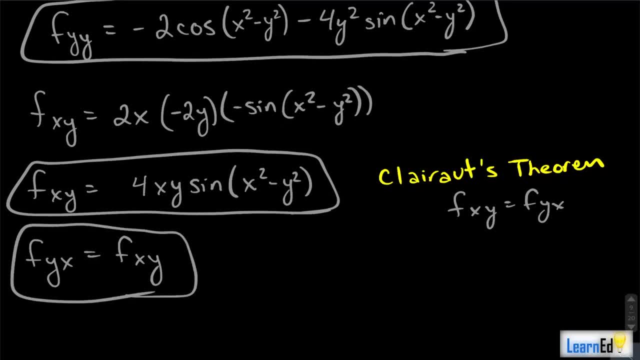 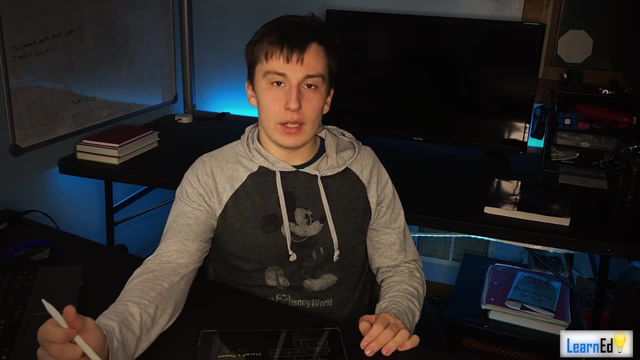 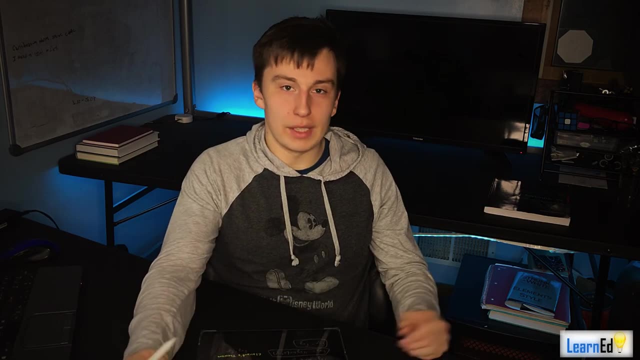 And there you go, Okay, And you can say via Clareau's theorem, right? So I would make sure to note that, because you don't want to get a point taken off because you didn't state a theorem or something like that. So, honestly, I would just write it down, rather be safe than sorry. 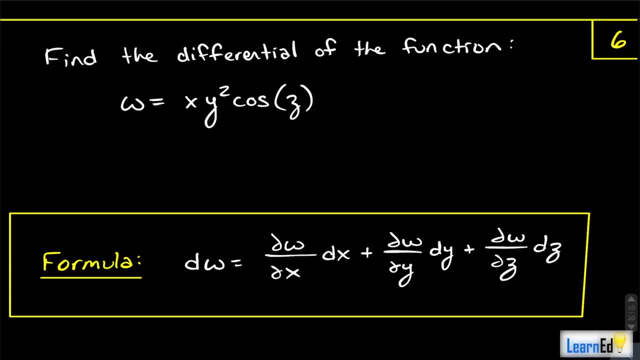 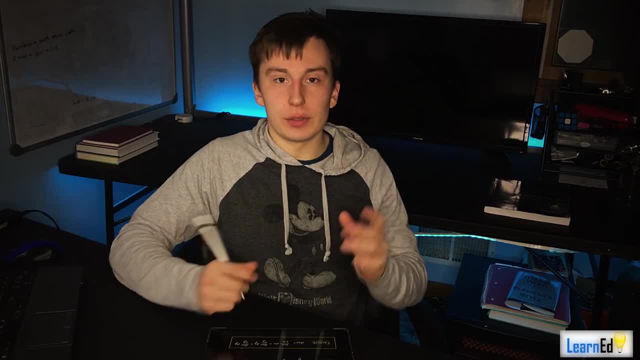 So for number 6, we want to find the differential of the function. w equals xy squared cosine z. Now what I want you to do is I want you to understand about differentials. okay, Because this is, while this was a small topic in Calc 3,. 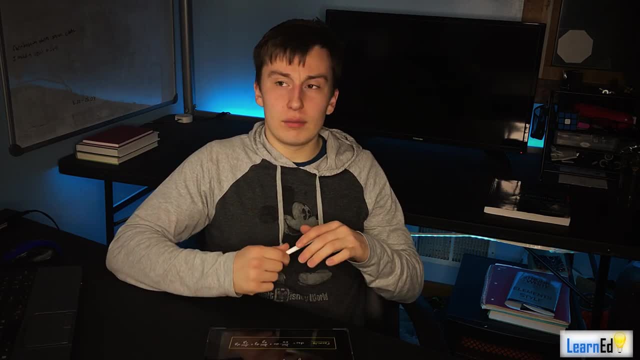 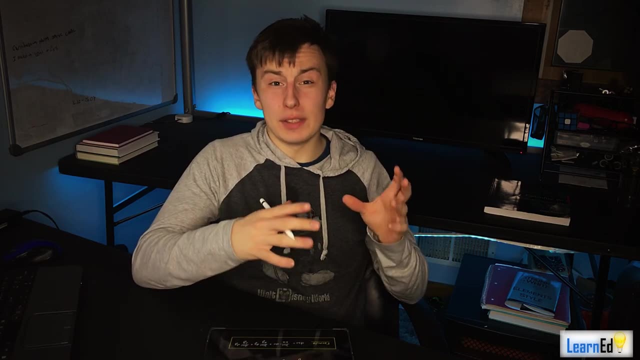 it was. you know it was covered with tangent planes, approximations, things like that. So you know, approximating something. this is a lot of applications in, like physics, things like that, So you know, and probably chemistry as well. 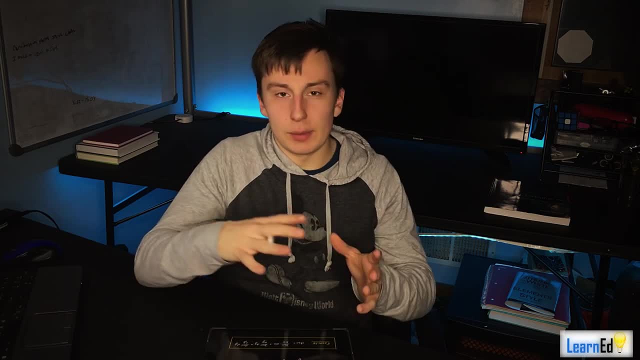 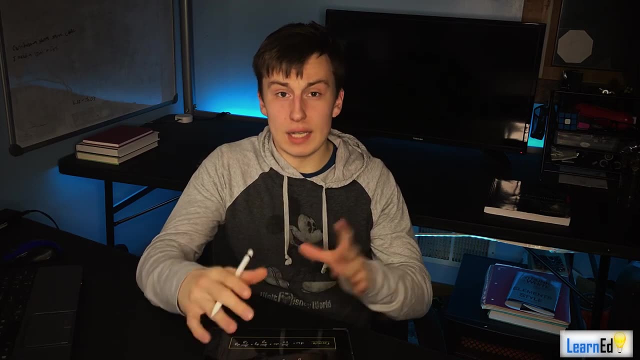 I don't know too much in the chemistry field So I'm a physics major myself, So you know it's something to I definitely go over. It's one of it's a good concept that you can take from Calc 3.. 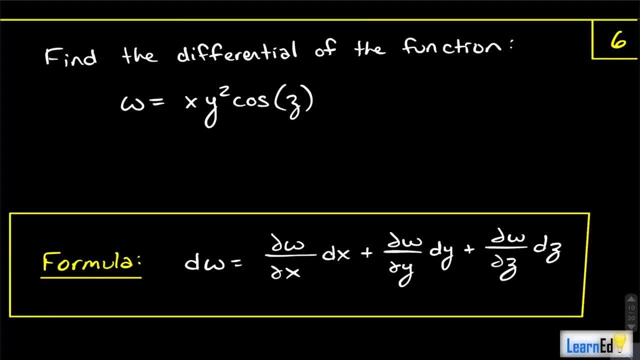 So I really want to go over differentials here. Now, the thing about differentials: okay, This is something that should be actually familiar to you, because it kind of is like a use of. in a way, the formula makes sense, Because if let's just take x's- okay. 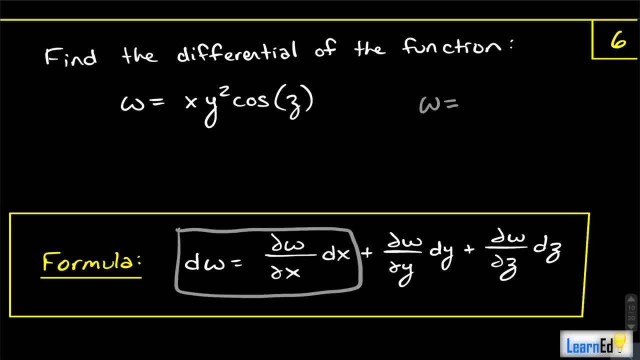 If you have w equals. if you make a u sub, let's say instead of w we write u: u equals 2x, then du equals 2dx. right, How did we find du? Well, it was equal to the derivative with respect to x of 2x. 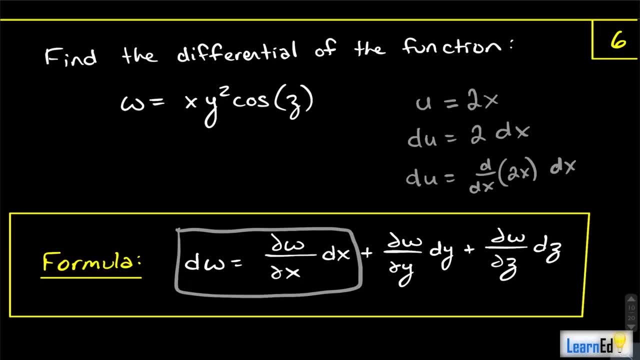 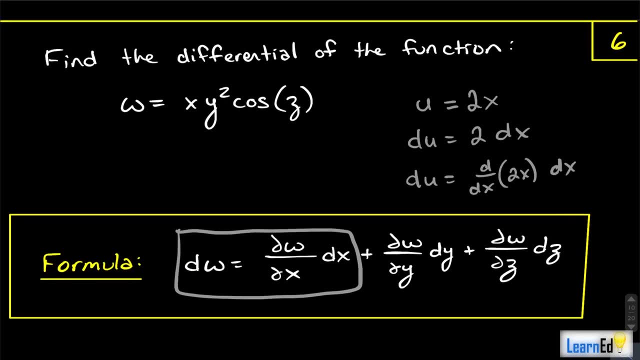 And then we added dx on the end. Okay, That's what this thing is saying. It's saying that d, instead of every time you see a w, just say u du equals partial, and we do partials now because we have multiple variables. 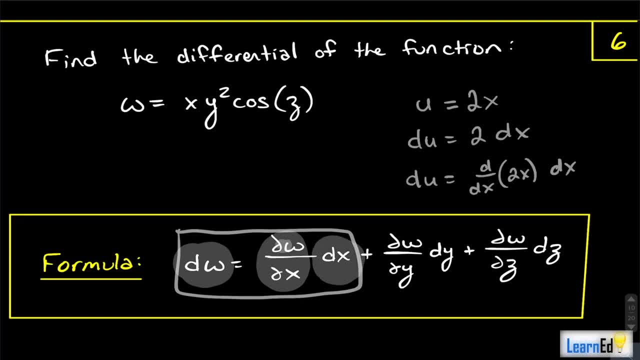 partial u over partial x, and then you have the dx on the end. So that's where, like, all that is coming from. But, and that should make sense, but now we're kind of adding on those extra variables. So what happens to the differential? 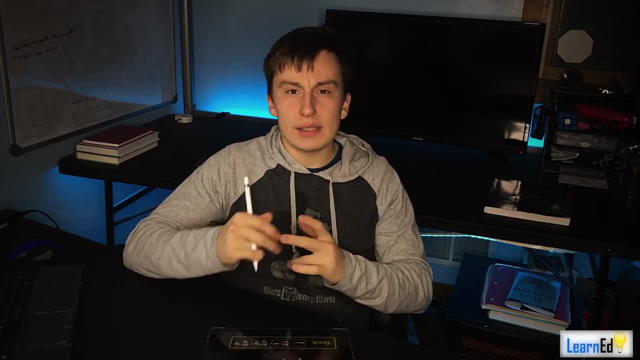 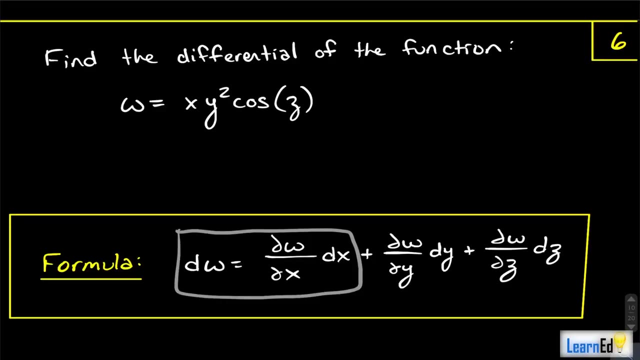 when you do certain things like this, right? So that's the whole idea of what you guys kind of covered with differentials. okay, Let's get into the problem. This should be a fairly simplistic problem. I just wanted to make sure I go over it. 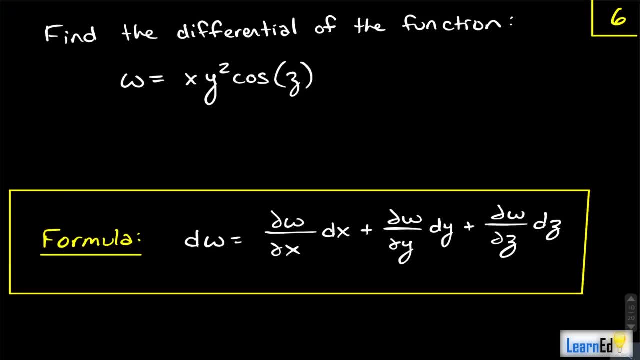 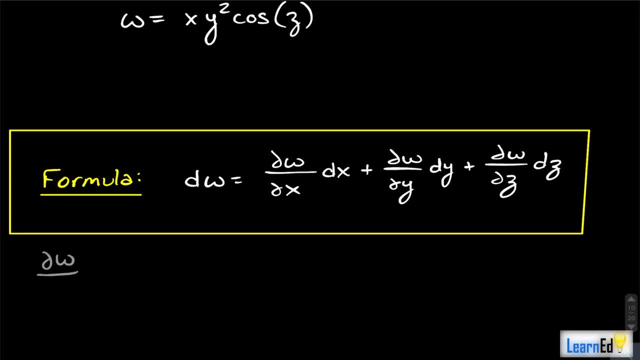 because this should be a good takeaway from Calc 3, I think. And yeah, let's just find the partial derivatives. We have: partial w over partial x equals. well, this just is, I mean, the y squared cosine z is a constant and the x goes away. 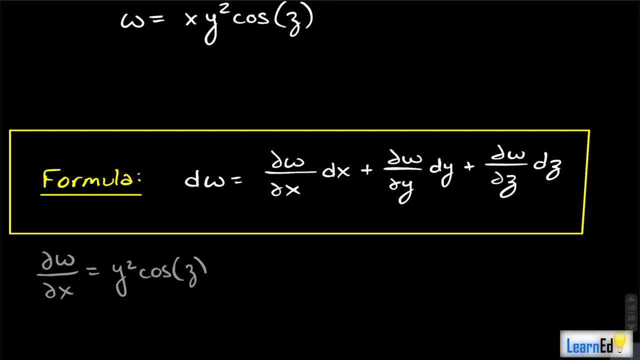 So you just have y squared cosine z. Partial w partial y equals this: y squared becomes a two y, So you have two xy cosine z. And lastly, you have partial w. partial z, which gives you cosine z becomes a negative sine z. 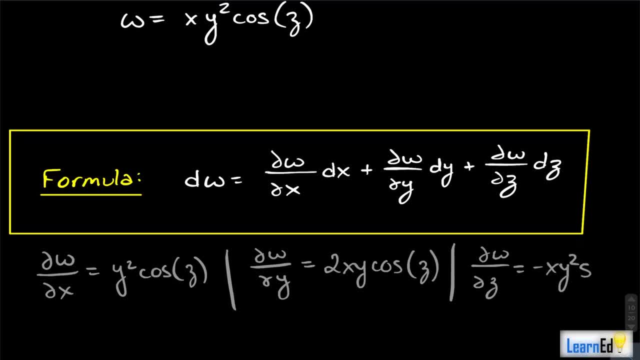 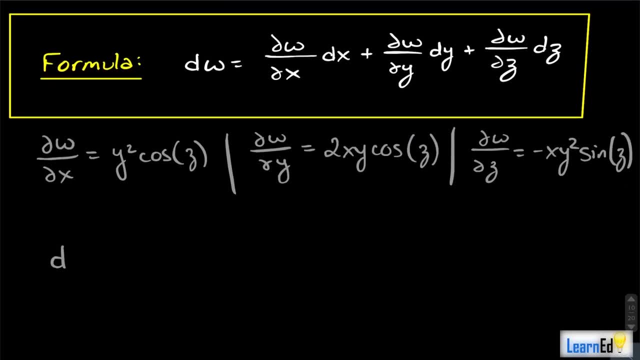 So you get negative x squared, no, sorry, negative xy squared, sine of z. There you go. Now, put it all together, get the partial, or sorry, get the differential Partial of w. So partial w, partial x is y squared, cosine z. 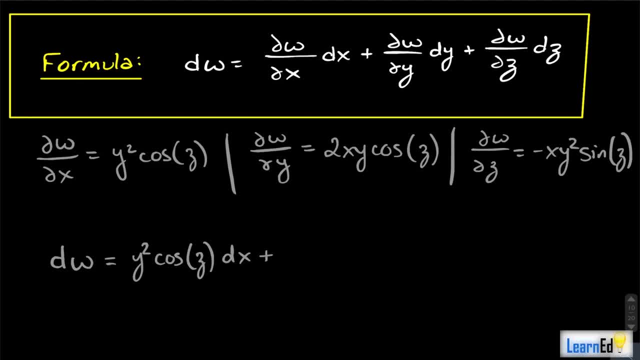 And we put a dx on the end: Plus two. xy cosine z, dy, plus, not plus. we're gonna have a minus, not two. don't know where that came from. What am I doing? xy squared sine of z And that right. there is your differential. 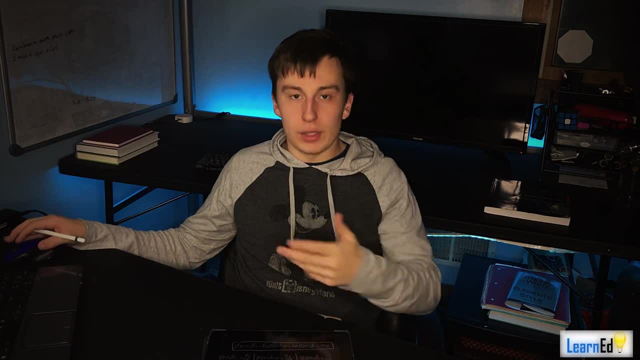 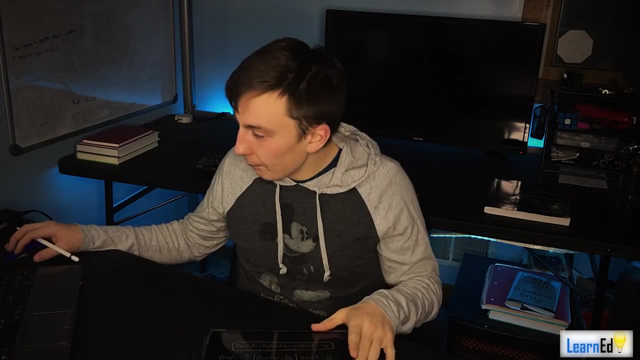 Again, not too rigorous. I just wanted to go over. you know what a differential is because, like I said, it has a lot of applications later on. So you know I wanted to make sure everybody is okay with that concept. 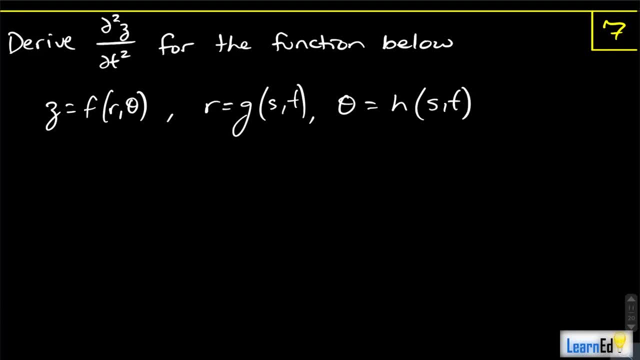 Moving on to number seven, we are asked to derive the second partial derivative with respect to t for the function below We have. z is a function of r and theta, and these r and thetas have individual functions themselves with respect to other variables. 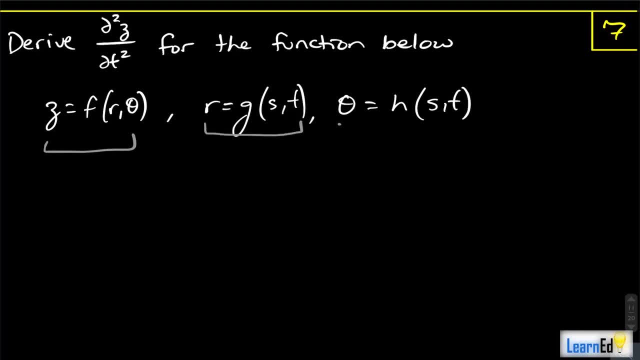 So r is a function g with respect to s and t, Theta is a function h with respect to s and t. okay, So now we have to use some kind of rule. What rule is that? Well, that's chain rule, okay. 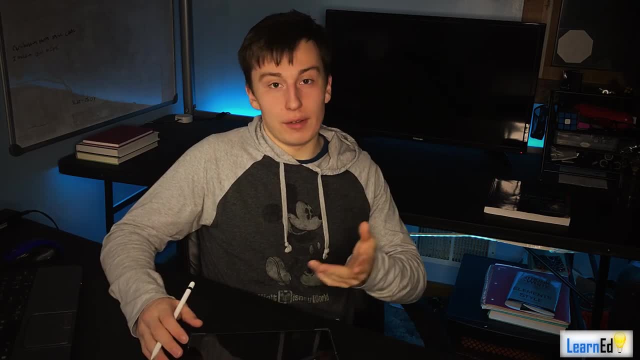 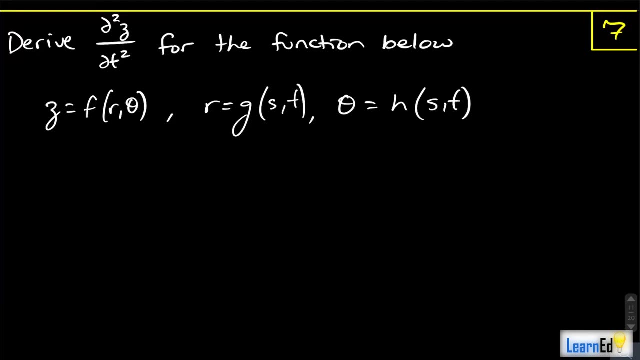 Now, chain rule is pretty easy for you know: first derivatives, okay, But then second derivatives. it might get a little more complex. so you know, you know the the derivation is going to be a little bit tougher, okay, so let's start off with the, the first derivative. okay, so for chain rule. 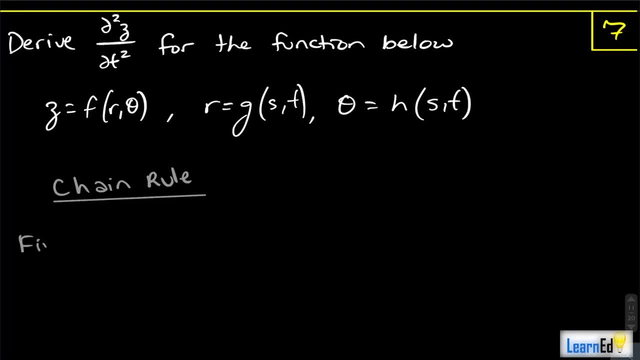 we are going to set up the first derivative now. the first derivative is going to be dz over dt. okay, so this guy is equal to. first off, we have z is a function of r and theta. okay, so r is a function of s and t. so to to get the to extract. 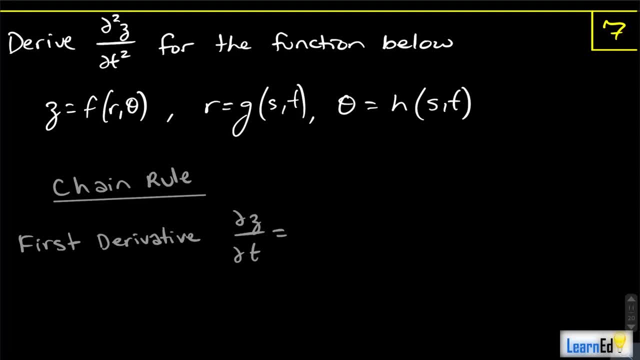 the t. what we have to do is first go through. we have to go through this r and we also have to go through theta. so our terms: we're going to have d, z over dr, so we're going to take a partial with respect to r, okay, and then for the r equation, we're going to take a partial with respect to t, and you see the. 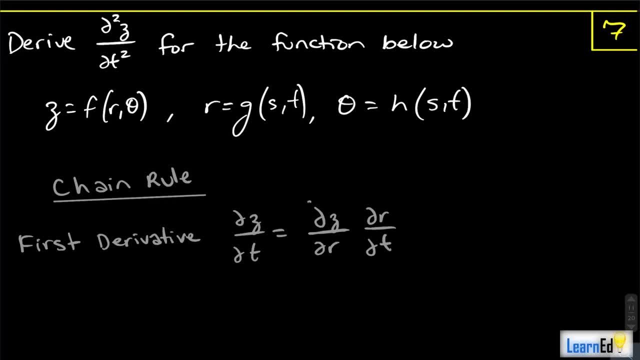 drs cancel out. we just get dz over dt, right, so that works out. and then we do the same thing with the theta equation: a partial derivative with respect to theta, and that's not added, then we have d, theta over dt, and there you go. okay, so that's chain rule for the first derivative, right. that's pretty. 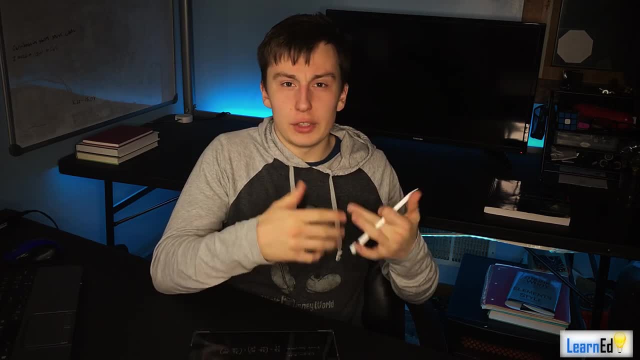 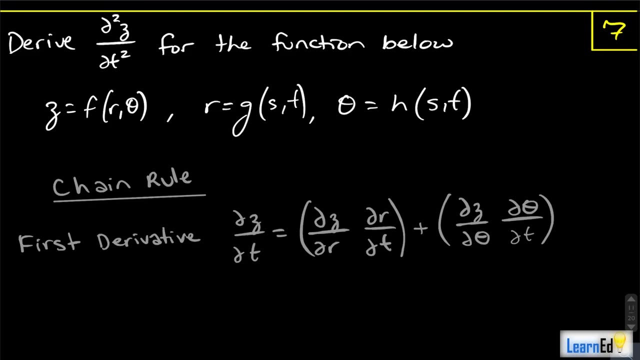 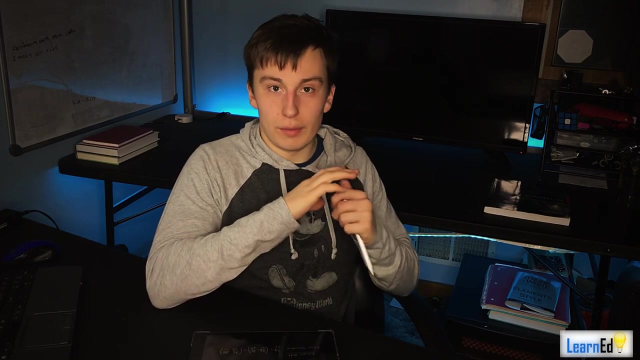 simple. that's, you know, kind of intuitive, right, it makes sense, okay. and also another thing to remember is that these are all going to have the curly d's. okay, because they're partial derivatives. okay, they're when you you're having a function of multiple variables. okay, so you have to have 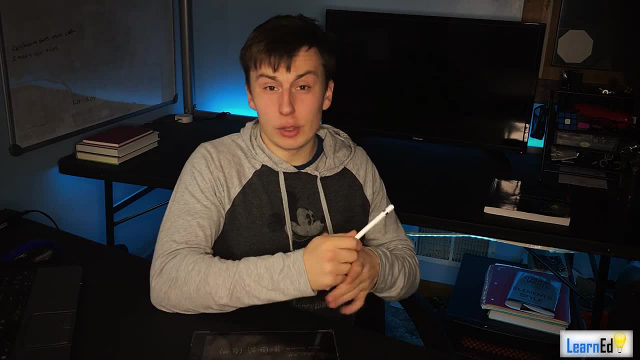 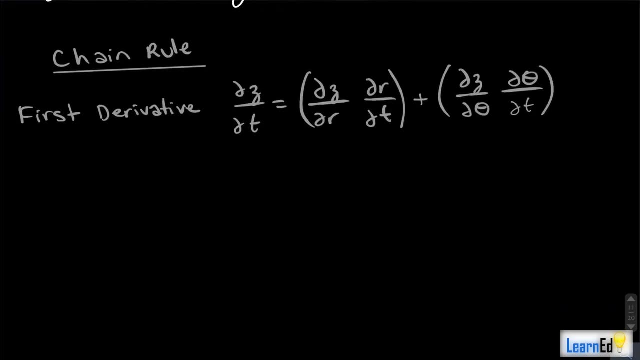 the curly d's when you take a derivative. okay, because you're only going to be taking a derivative with respect to one of those multiple variables. okay, that's the chain rule for the first derivative. now we have to move on to the second derivative, which is going to get a little more complex. so 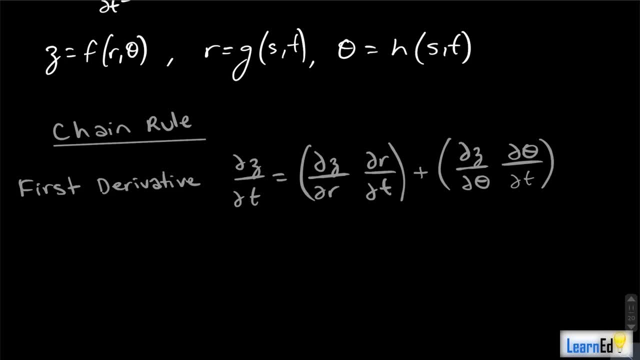 what we're going to have to do is take a derivative of both of on both of these sides. okay, so we're going to take a derivative, a partial derivative with respect to time of each side. okay, so we can go through with that. you have d over dt of this huge thing, and i'm just going to copy this below: 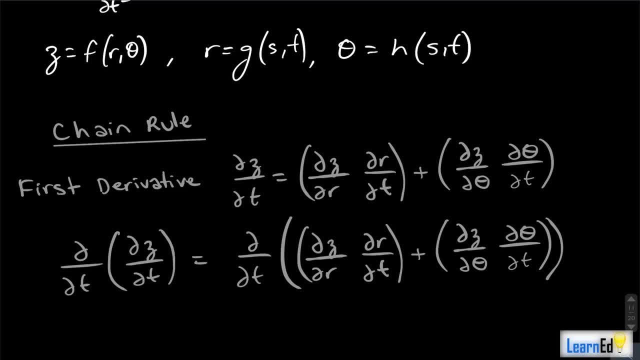 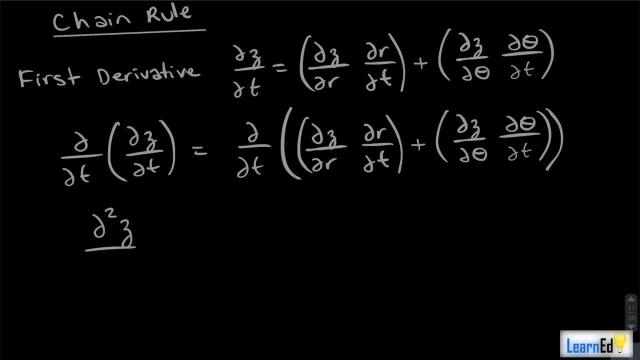 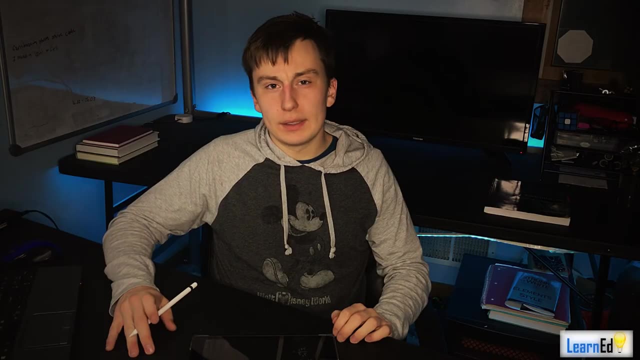 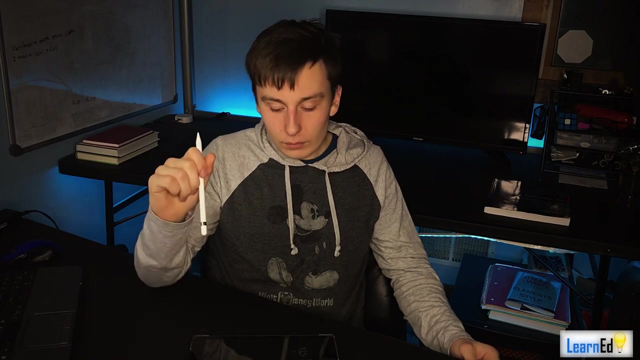 okay. so in taking a partial with respect to time, on both sides, we have, you know, the, the d squared, z over dt squared, okay, and how are we taking a partial with respect to t of this, this huge mess that we have going on in the right-hand side? what we're going to have to do is use some, some. 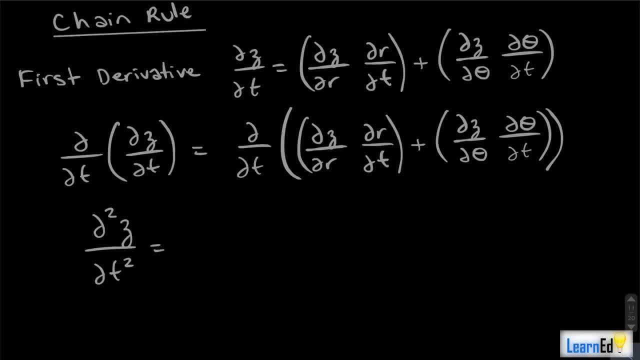 some product rule here, okay. so the reason why is, first off, these are two separate terms. this thing and this thing are two separate terms, okay. so it's kind of like having like 2x plus 2 and taking a derivative with respect to x. okay, that's just 2 plus 0, right, so it's 2, you can take the derivative. 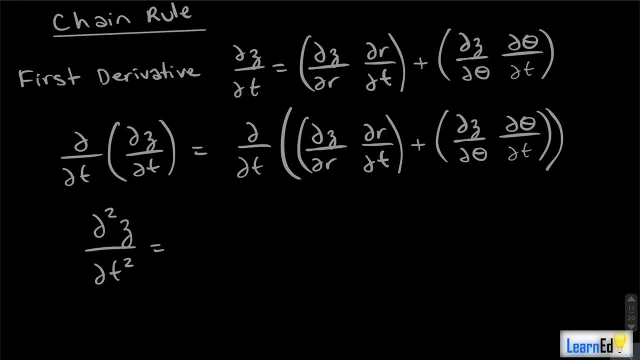 separately of each term, but what i'm talking about here. but from using product rules, we have to use product rule inside here, because we have two things being multiplied together. okay, so we're gonna have to use product rule here and product rule here, so we have two cases of 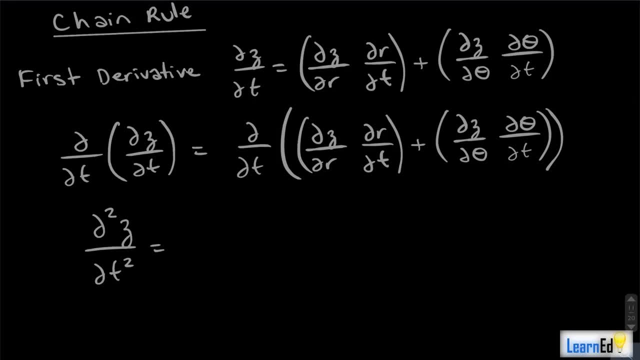 product rule to deal with. okay, so if we're trying to find, if we're trying to use product rule for the, the first pair, okay, let's use product rule for this piece right here. what we have to do? first let's take a partial derivative with respect to time of dz dr. okay, so we'll do partial of dz dr, and then we're gonna have to multiply dr- dt. 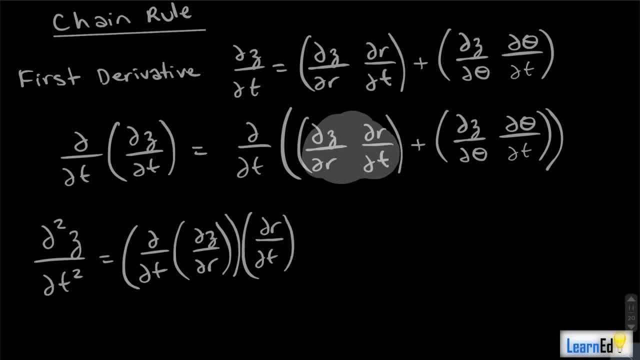 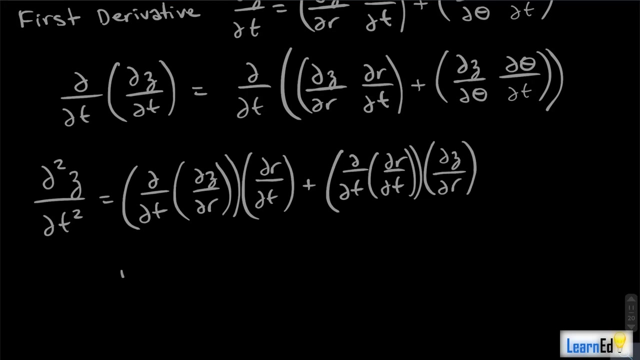 and we don't take a derivative of that. okay, then we're gonna add that to. we're gonna do the opposite. we're gonna take a partial derivative with respect to time of dr dt and we're gonna leave dz dr alone. okay, and then, since we did the first piece now, we're just gonna add on to the second piece the. 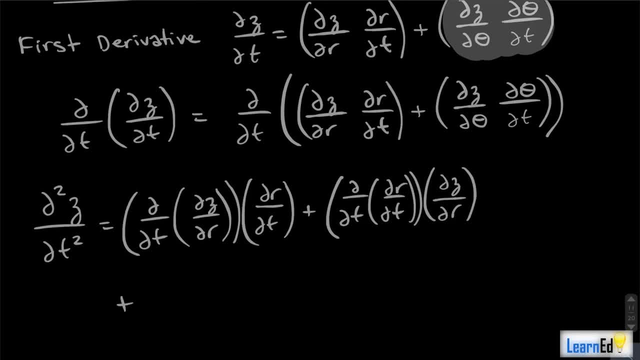 dz d theta d theta dt. we're gonna take a derivative with respect to time of dz d theta, okay, and then we're going to multiply that by d theta dt, which we're going to leave alone. and then we're going to add that to the partial with respect to time of d theta dt and we're going to multiply that by dz d. 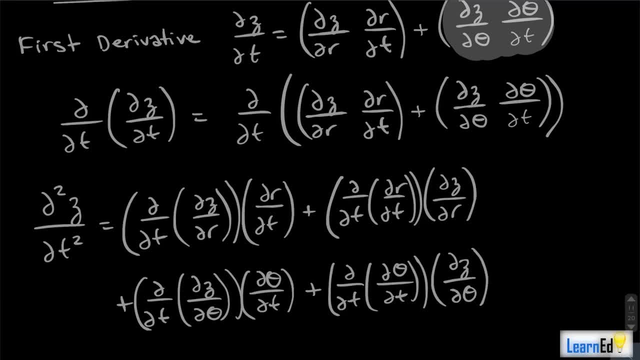 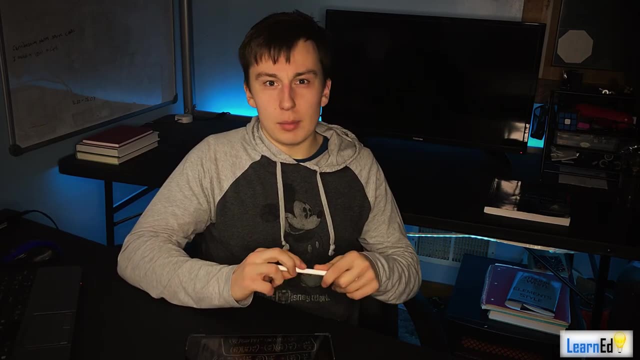 theta, which we left alone. okay, in this whole thing is your second partial derivative with respect to time. okay, so you have to do quite a few things to actually get through to, you know, that that time. so it is a little or short to that, to that, to that uh t variable, and i believe i just referred to that. 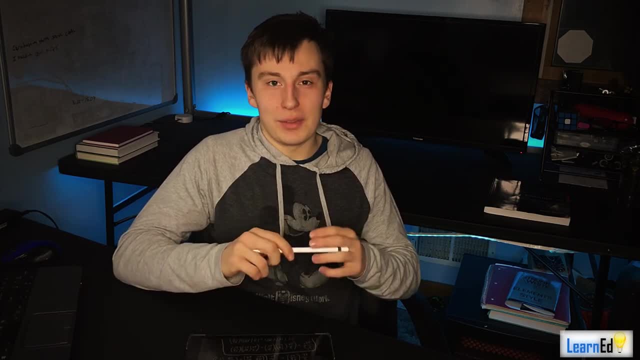 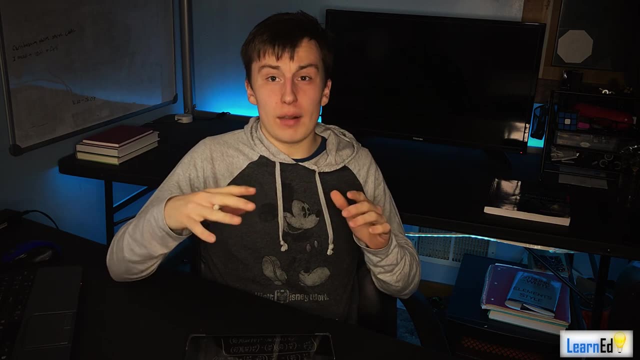 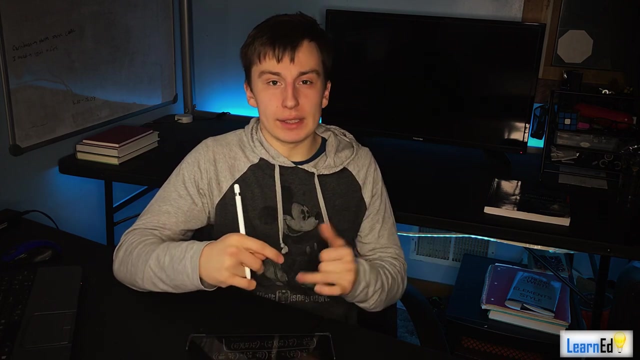 as time throughout the whole problem. i don't know, but you understood i what i what i meant there. anyways, yeah, so chain rule can be really really messy, especially with this. if you, if i gave you um, all like the, the functions and everything, and i, like you know, like real functions and i didn't 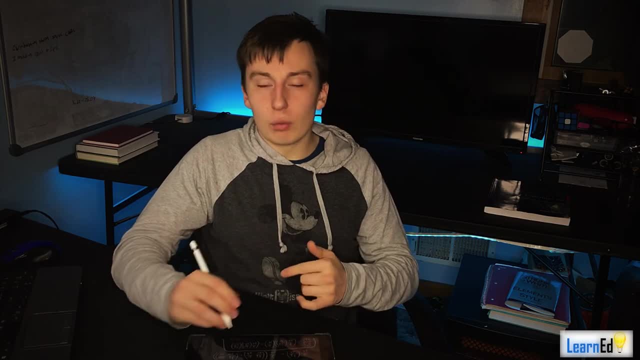 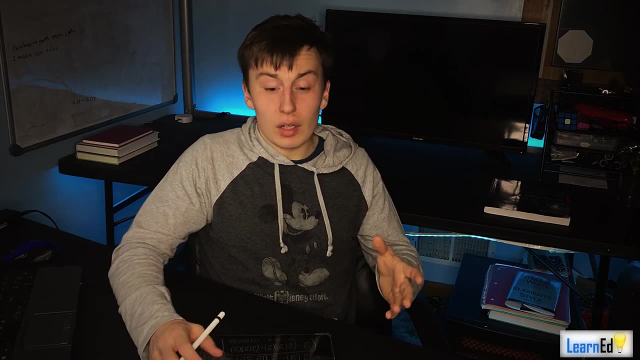 just make this like a general problem. this would be really really messy to go and compute all of these different things, and, yeah, i wasn't going to do that to y'all, so, um, anyways, that's how you work with chain rule, okay, so i the. the whole purpose of this problem was to get you to really 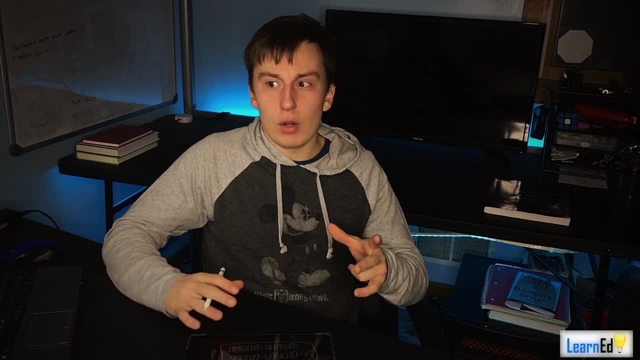 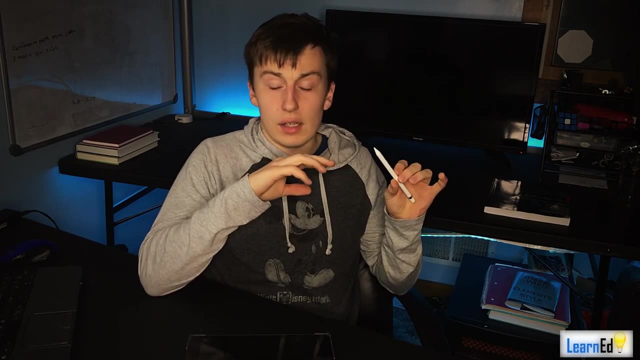 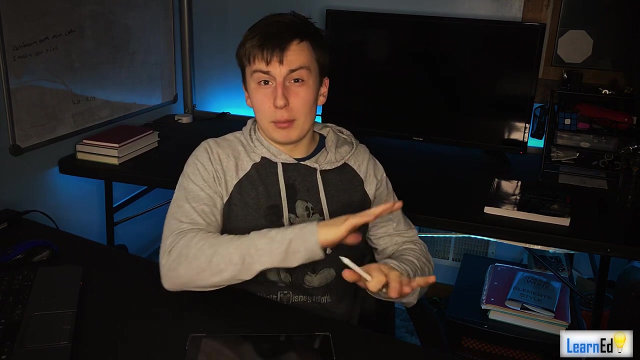 understand how chain rule works. okay, and how we can find the second derivative with chain rule. okay, we're about to get into like maximins and lagrange multipliers and like, uh, you know some some kind of um, you know, and some gradient stuff as well. so if you want to take a break before we 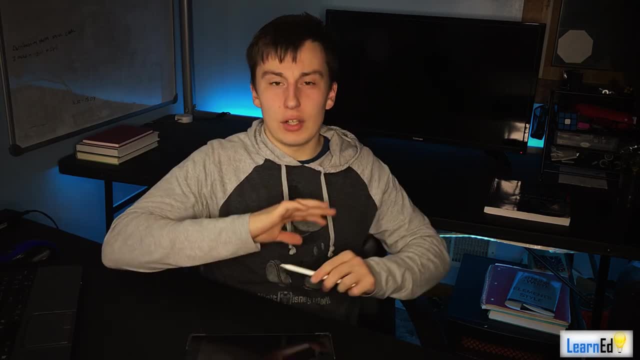 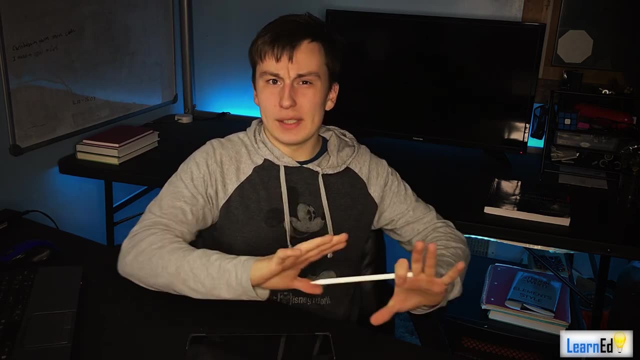 get into that, feel free, you know, take a five minute break quick, just kind of go over everything that we did. it was not not the the worst stuff in the world, okay. so hopefully that all makes sense to you. so for number eight, we want to find the maximum rate of change of f at the given point. 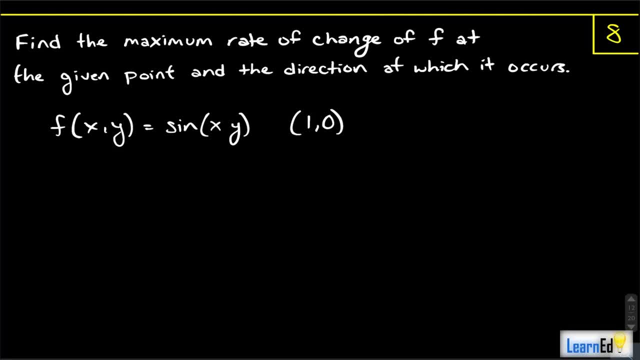 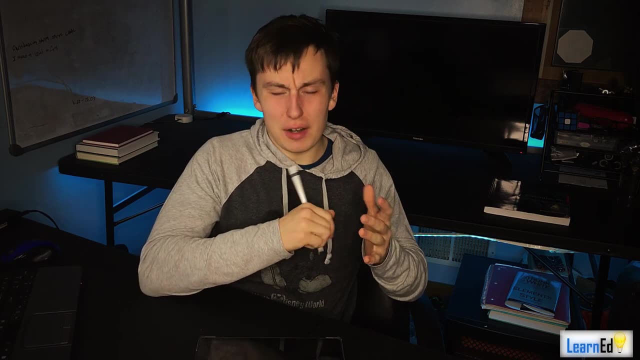 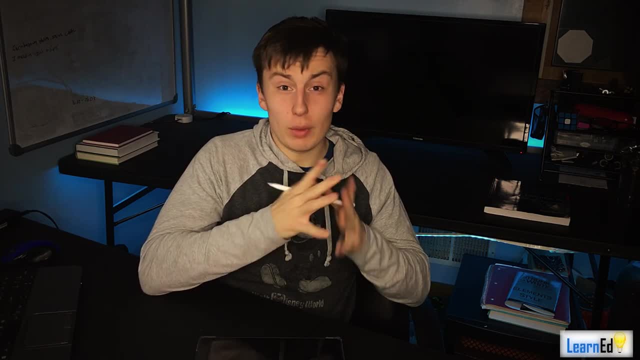 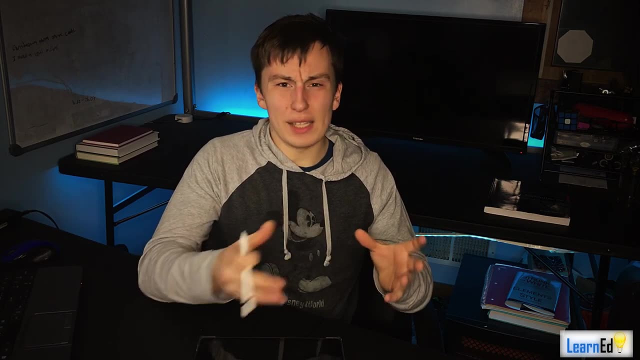 looking for then. so what, what's that? what's that value called? it's the gradient. okay, the gradient. so you know, when i was in calc three i would have been like, okay, why is the gradient the maximum rate of change? right, i was. i was very confused as to why that is, so i want to explain that to you. so 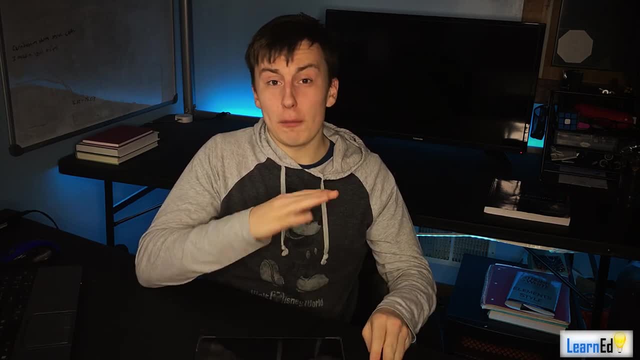 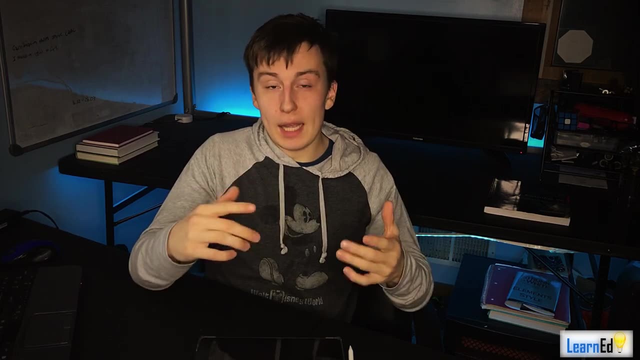 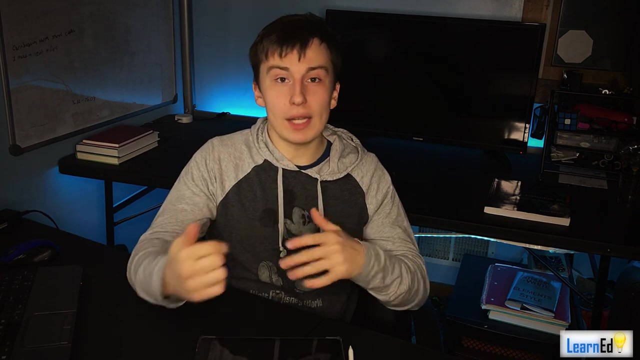 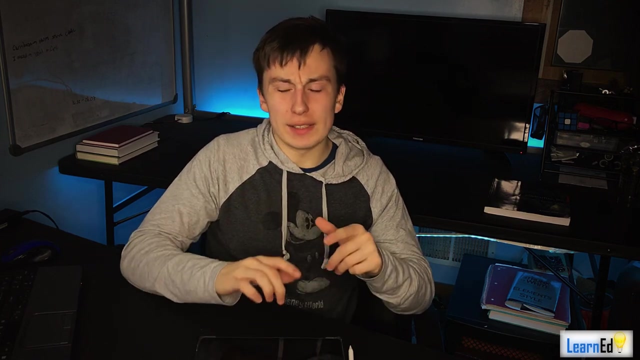 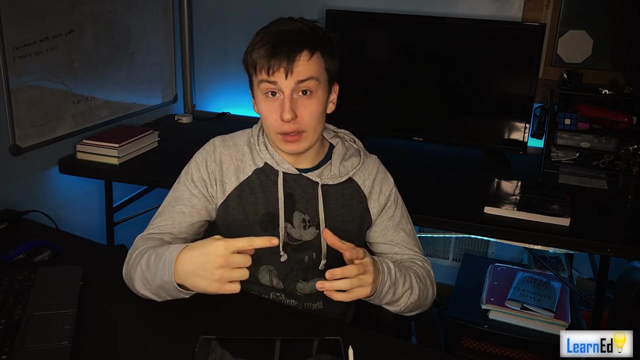 you actually understand it right, and that's all going to start out with partial derivatives. okay, i talked about what partial derivatives were and i'm going to talk about what partial derivatives were earlier, when we were covering it. a partial derivative with respect to x is the, the, the slope in the x direction at any point on a surface. the partial derivative with respect to y is the same thing: just slope in the y direction at any point on the surface. okay, a directional derivative which gets covered with gradients is the slope in any direction that you you want, but you have to specify it with a unit vector. okay, so you can't just find the slope in every single direction, you have to use a unit vector. 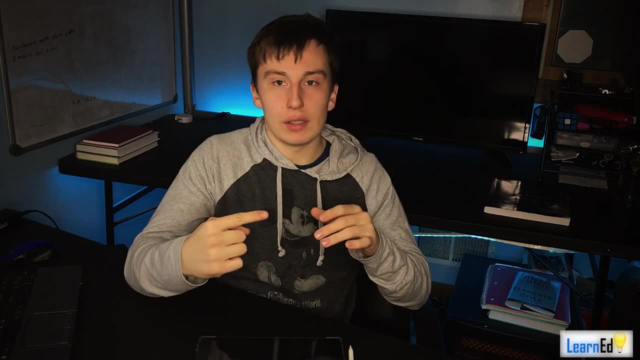 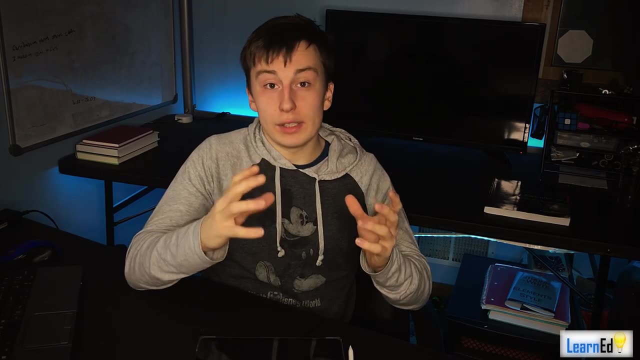 okay, so you can't just find the slope in every single direction. you have to use a unit vector. okay, so you, you know you only um get to find the slope in a single direction. all right. so now that you understand directional derivatives, we have to use an equation that we know to figure out. 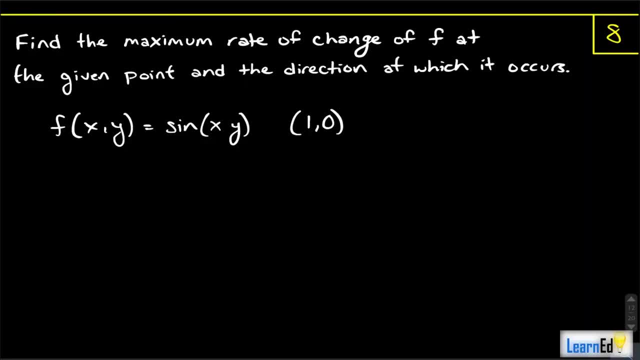 what the meaning of the gradient is. okay, we know that the directional derivative of f equals del f, so the gradient of f dot u. okay, so, since this is you know, since this is an equation that we know and you know, if you want to understand why we're able to do this equation, you can look in in your textbook or something like that. i don't. 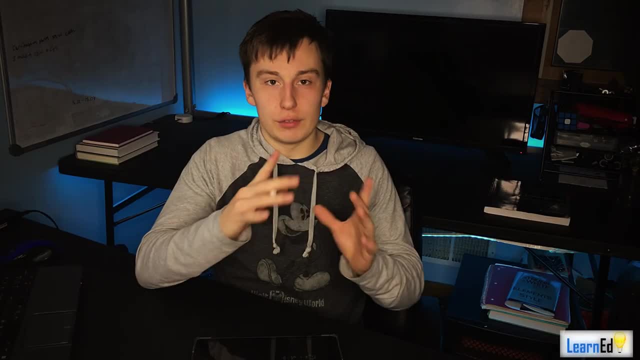 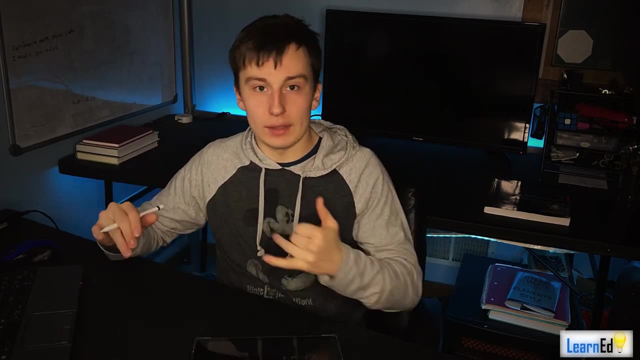 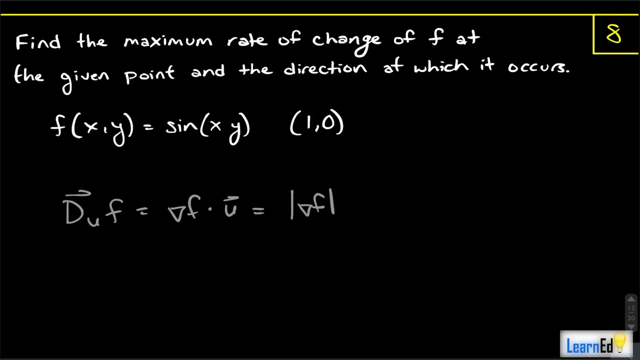 want to spend too much time on this, but when you take the dot product of two things, you can just, you know, have the magnitude of those things times cosine theta. right, so a dot b equals a b cosine theta. so we can rewrite this as the magnitude of del f. del f is a vector. it usually doesn't have a. 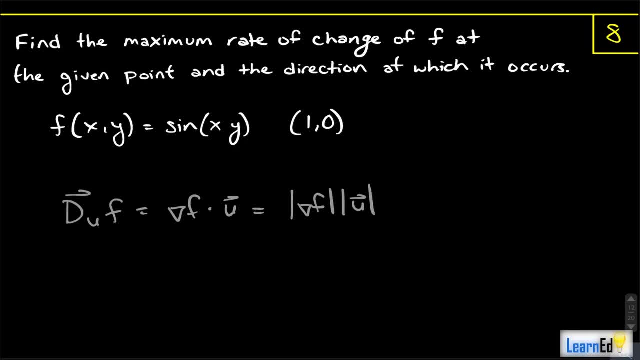 vector sign over it. uh, how, when i see it? so i think it's kind of just implied, but it's equal to that. so when will this directional derivative be a maximum? well, the unit vector, the magnitude of the unit vector, is always going to be one. okay, and cosine theta: what's the max that cosine theta can? 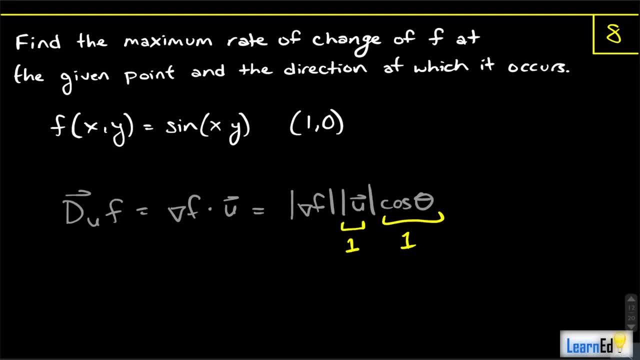 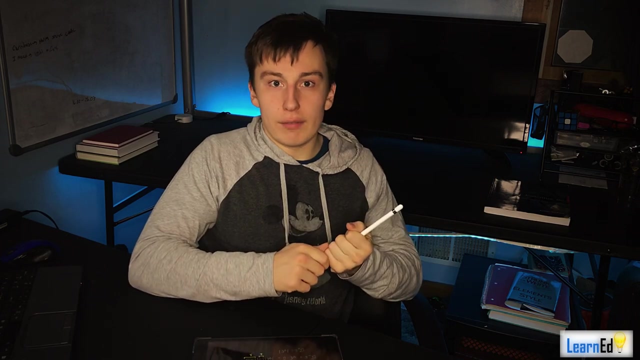 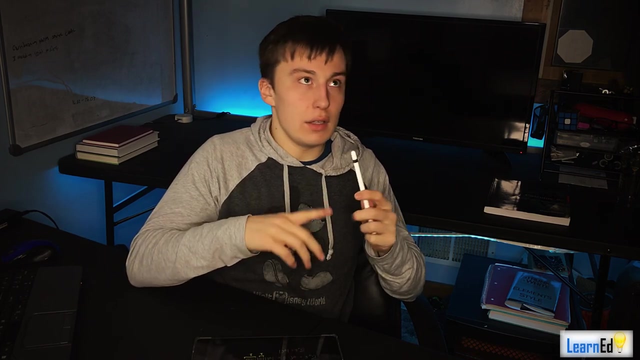 be well one. okay, so at the max um, the, the max slope of the directional derivative of f is equal to the magnitude of the gradient vector. okay, so the direction of the steepest slope: right is the gradient vector and the magnitude of the gradient vector is the value of the, the steepest slope right. so it's. it's telling you what the steepest slope is. 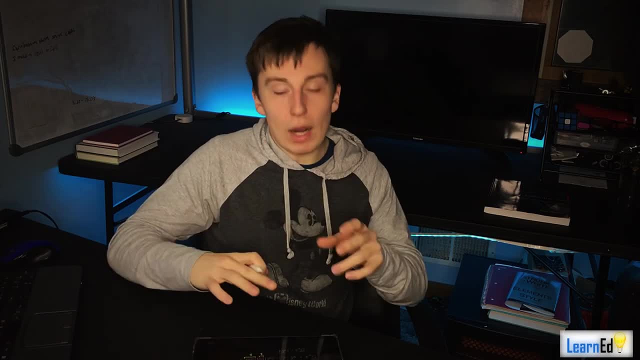 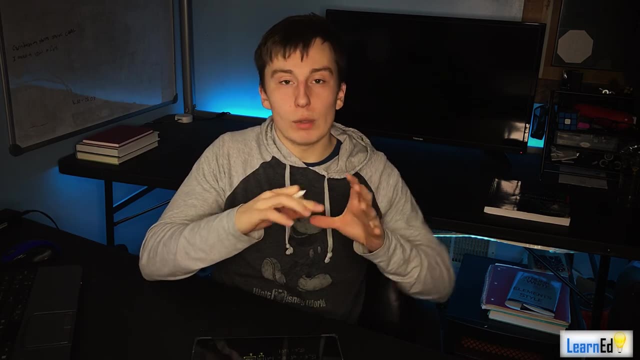 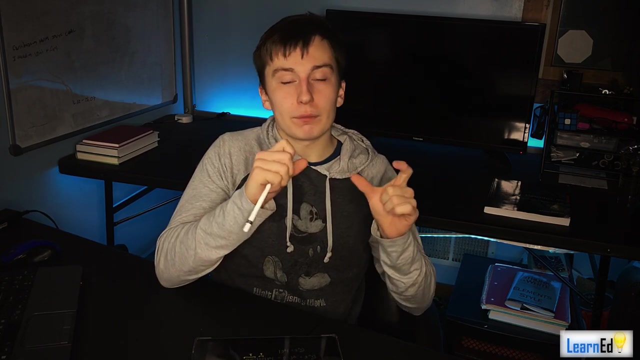 from that point. okay, that's why, though? okay, because we know we have that equation for the directional derivative- if we're trying to find the max- what's the maximum value that that directional derivative could be- it's going to be the point where the angle between that unit vector and the 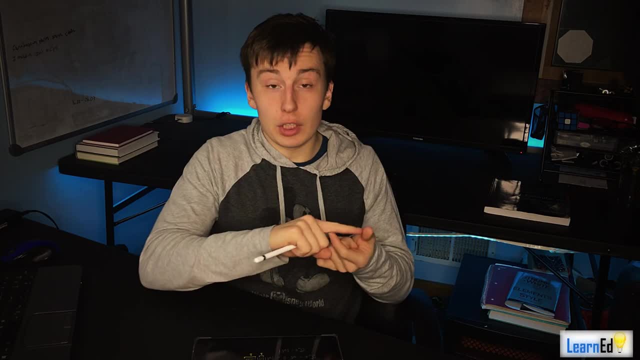 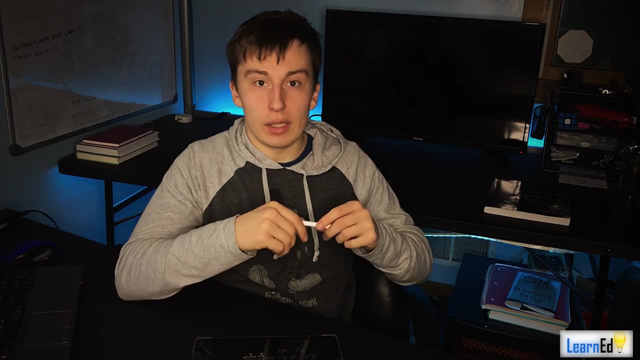 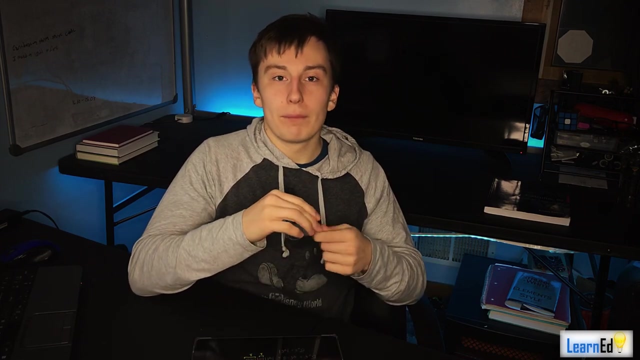 directional derivative are the same, meaning that the direction you're going in is the direction of the gradient vector. okay, because if they're parallel, then you end up with cosine of zero, right? there's zero degrees between those two angles, so that's one, all right. so your unit. 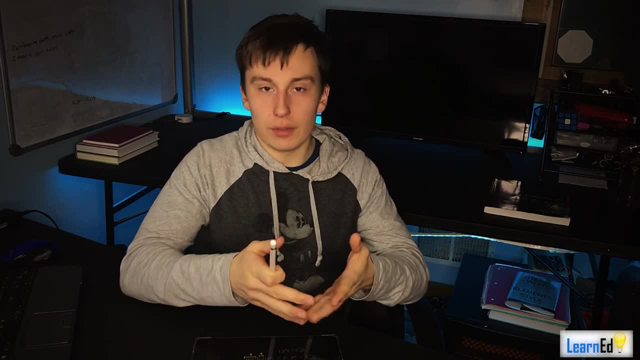 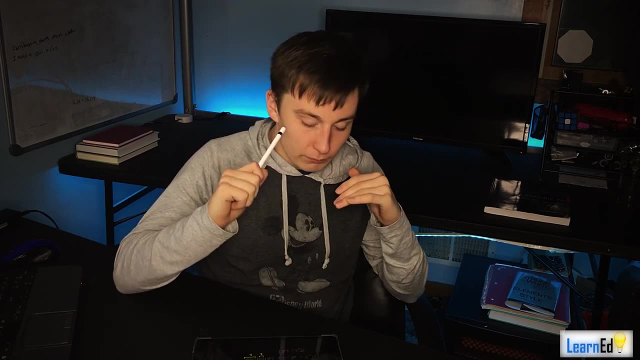 vector right. your direction of the steepest slope is the direction of the gradient vector. that's the whole point i'm getting at. that's why the gradient vector is the direction of the steepest slope, all right. so if you understand that, now we can kind of begin this problem. we want to find the maximum. 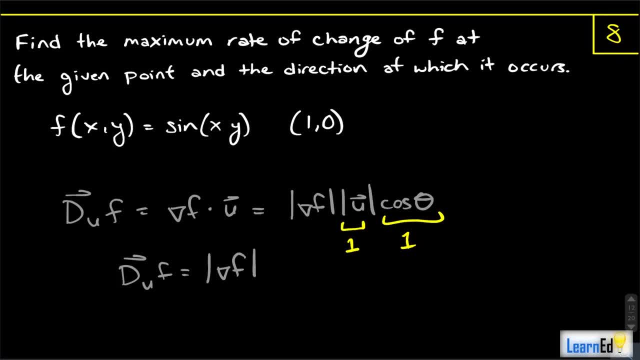 rate of change at f. i'll repeat the problem. we want to find the maximum rate of change of f, so we want to find the magnitude of the gradient vector at the given point and the direction at which it occurs. so we want to also find the direction, which is just the. 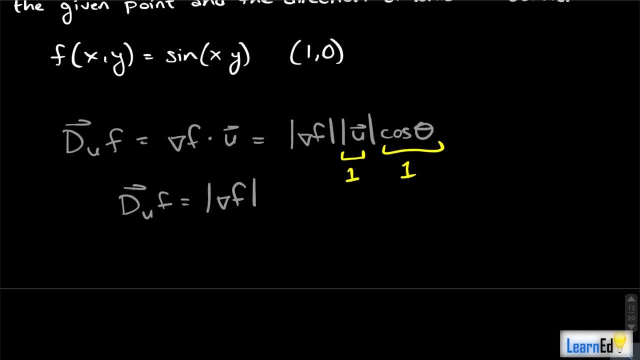 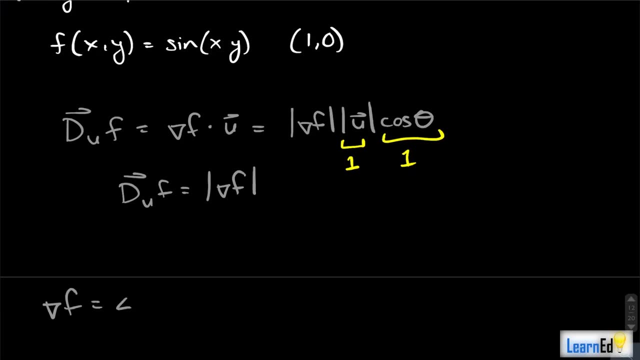 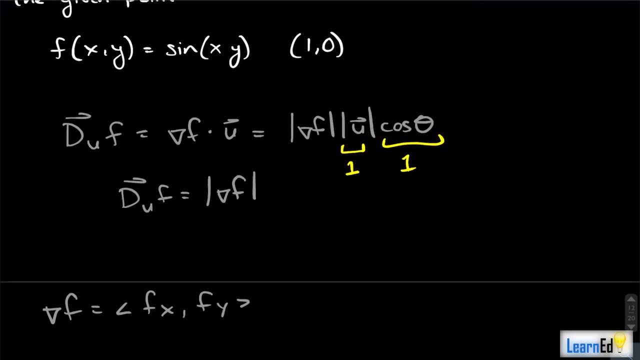 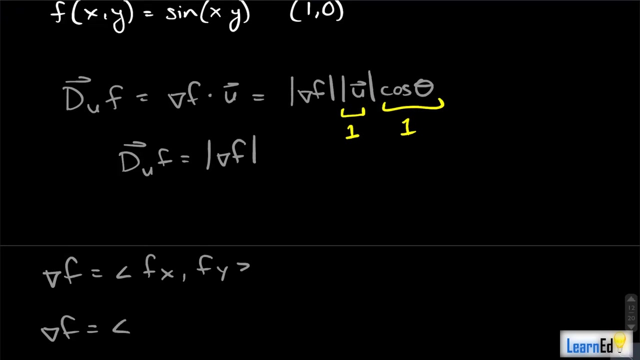 gradient vector itself. okay, so let's get to that now. the gradient vector is just the, in this case just going to be the partial of x and the partial of y in two separate entries. okay, that's our equation for the gradient vector, now the partial, with respect to x, of sine x, y. 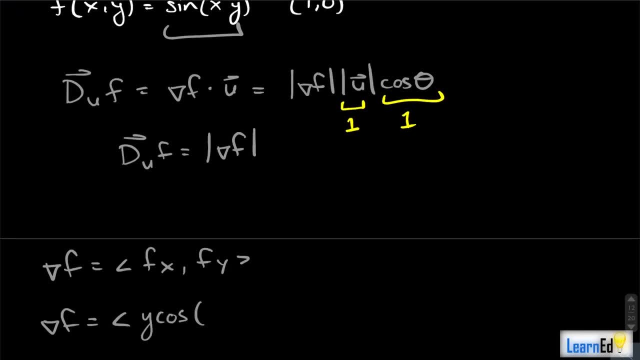 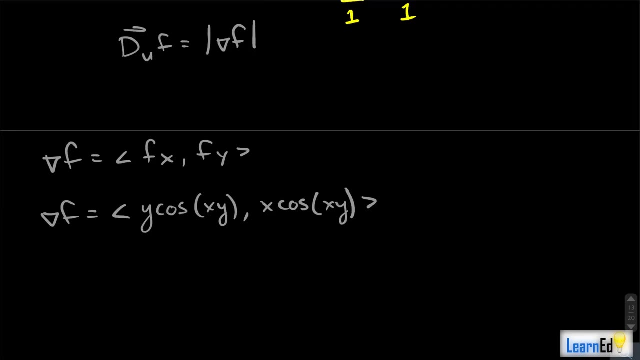 is just going to be y cosine of x- y, and the partial with respect to y is going to be x cosine of x- y. okay, so now we can just plug in our point. our point is: one zero delta, uh, del f at one zero equals. well, our first entry is just going to be zero, because we 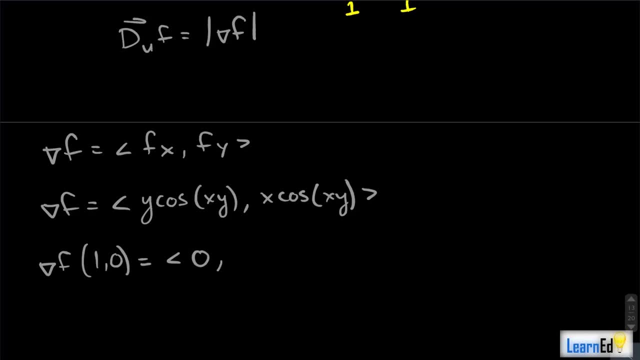 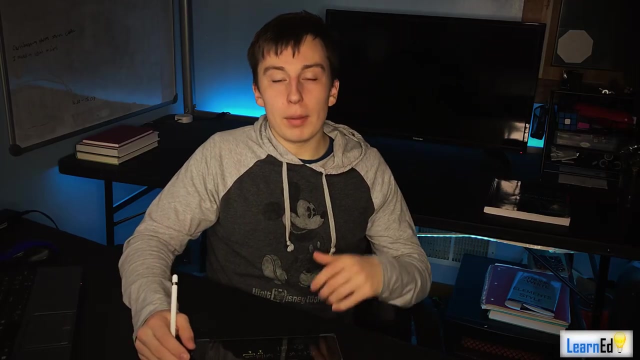 know that y is zero and our second entry is well going to be one times cosine of zero, which, remember we said cosine of zero is one. so we just get zero one and this is the direction of the maximum rate of change. okay, but that's not the whole entire. 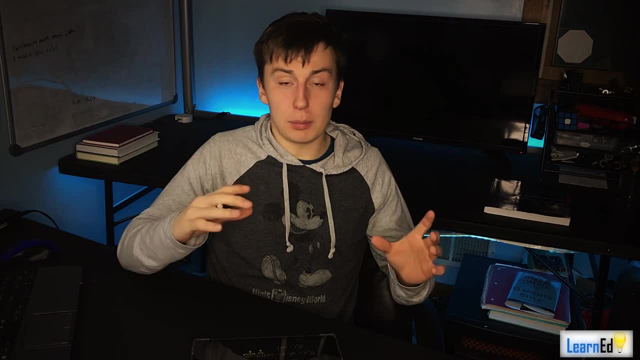 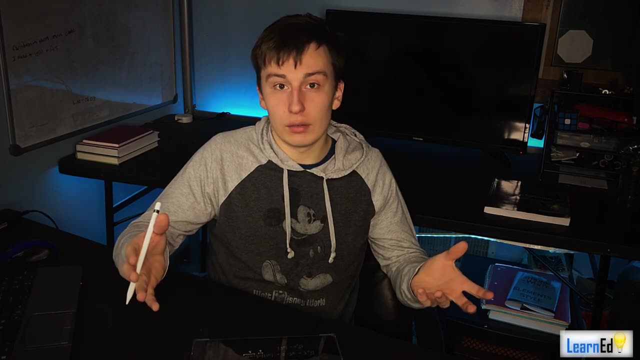 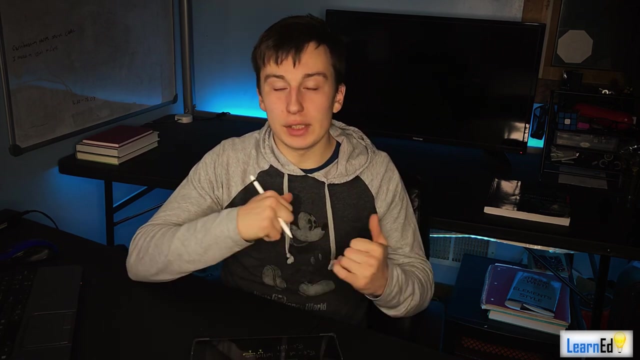 problem right, the initial, you know, the initial problem was asking us to also find the maximum rate of change. so we just have to find the magnitude of the gradient vector. okay, and, and, and, and. remember, i just showed you the the whole reason why the maximum rate of change is the. 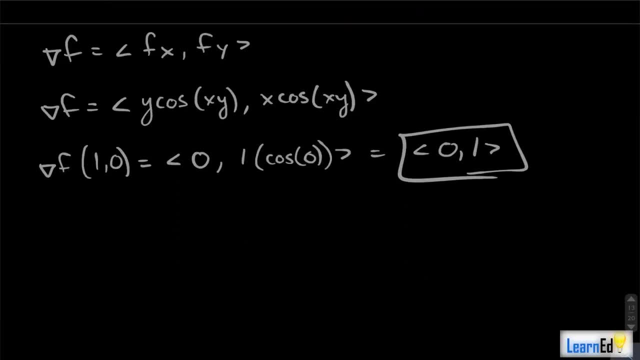 the magnitude of the gradient vector. if we find the magnitude of the gradient vector, okay, magnitude of this is equal to the magnitude of zero one and there. so it's equal to square. root of the sum of the squares is zero squared plus one squared. uh, this is equal to just one. you can. 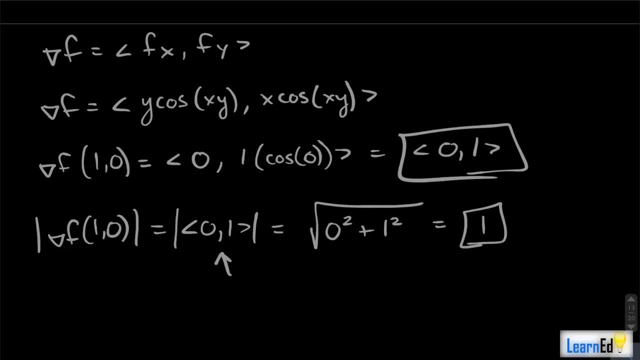 already tell that this has a magnitude of one, because it's just, basically, j hat okay, so you don't really need to. you know, do the whole square root thing if you don't want to. but yeah, that's, that's literally number eight right there. okay, that's just finding the gradient vector now you. 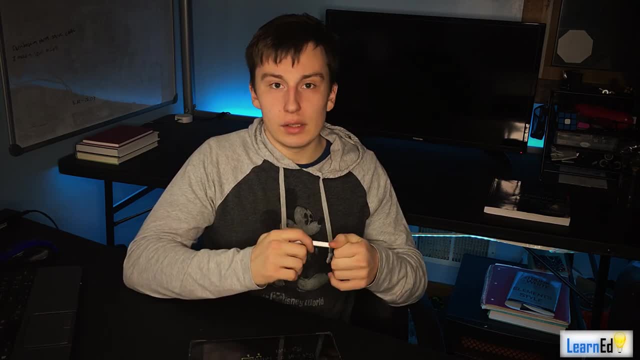 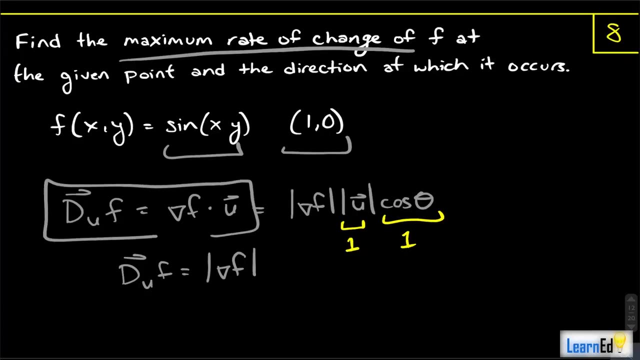 may be asked to find the directional derivative, in which case, you know, maybe they give you direction, you find a unit vector for it and you use the exact formula that i just showed you here. okay, so the only other thing you could be asked to do is, like i said, find this directional derivative. okay, so you what they would do. 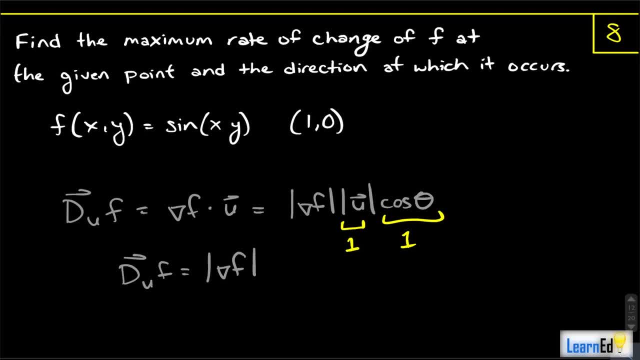 is, they would give you a direction. excuse me, they would give you a direction. you find a unit vector that's in that direction. so you just, you just um, normalize the direction that they gave you, dot it with the gradient vector and there you go, you have your directional derivative, okay, so actually, it's, it's. it's a pretty simple. 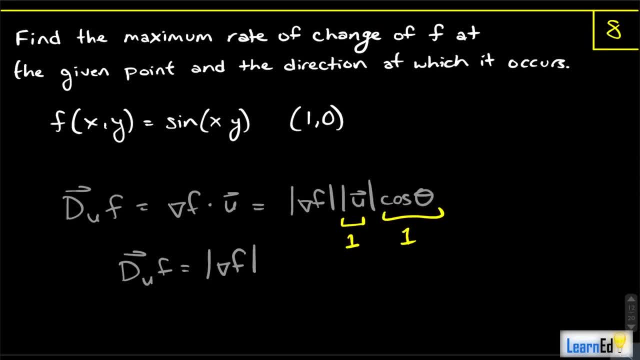 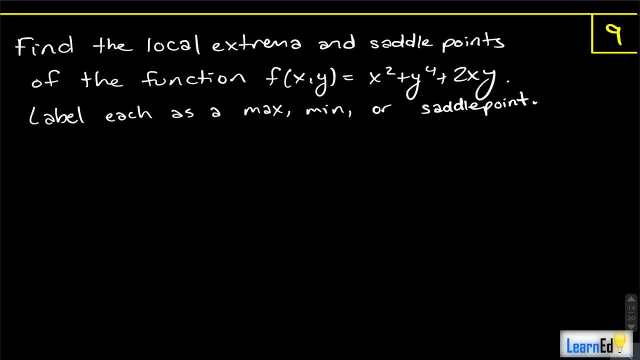 problem if you understand the whole idea of what the gradient vector actually is, what a directional derivative is and what a partial derivative is. okay, so on to number nine. all right, number nine. we want to find the local extrema and saddle points of the function. uh, there's a function f of x and y. 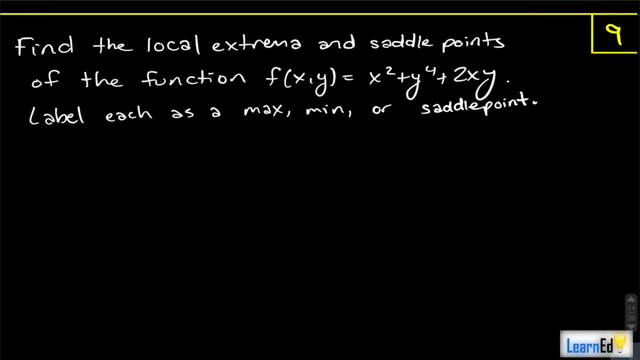 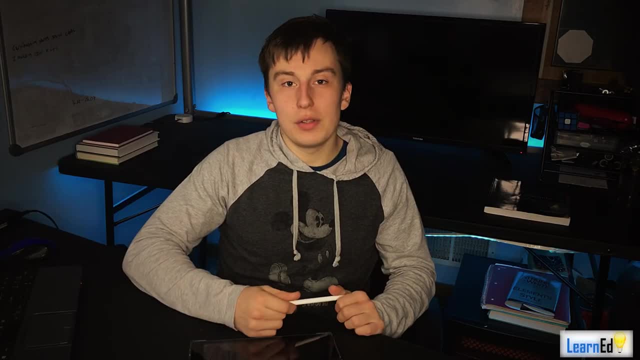 equals x squared plus y to the fourth, plus two x, y. and we're going to label each extrema as a max, a min or a saddle point. okay, how do we do the, the extrema stuff, like we, we know how to do that in calc one right, we just, you know, we use, we use a bunch. 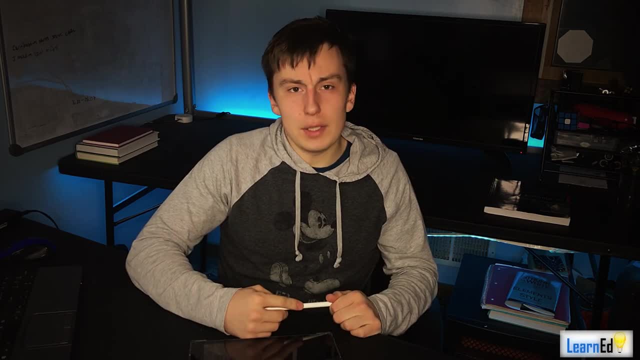 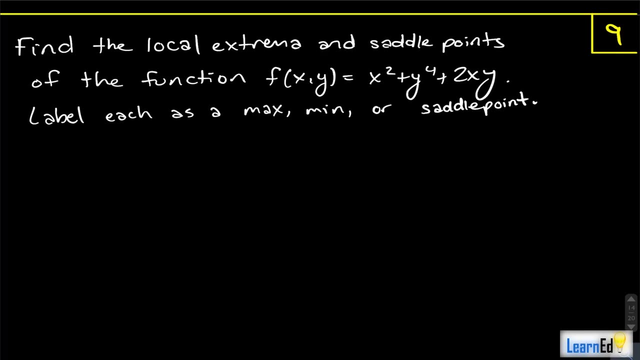 of derivatives. but how are we going to do that in three dimensions? well, if you remember, this is going to involve some partial derivatives, okay, and it's going to involve that d. right, it's going to involve seeing if that that d thing is greater than zero or if it's less than zero. 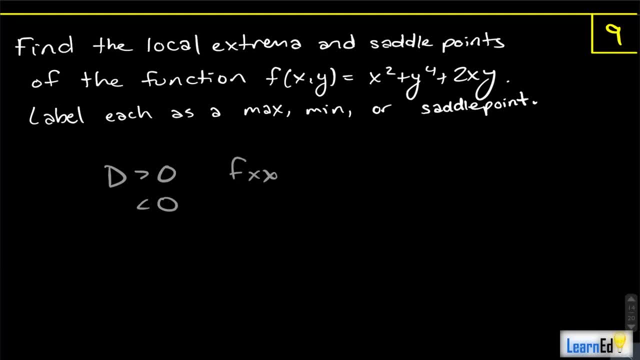 and then you're going to have to look at the partial with respect to x or the double partial derivative or whatever it's. it's a process. okay, it's definitely a longer process than it was in. uh, in calc one, i'm gonna switch over to the white. honestly, i don't. i don't like the gray as much. 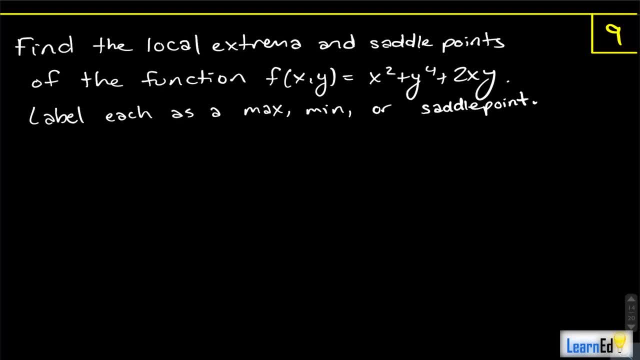 honestly, i'm not. i'm not a big fan anymore. i was the beginning of this video. now i'm like, nah, yeah, so i hated maximins when i was in calc 3. it was. it was a long process, but don't worry, this isn't. 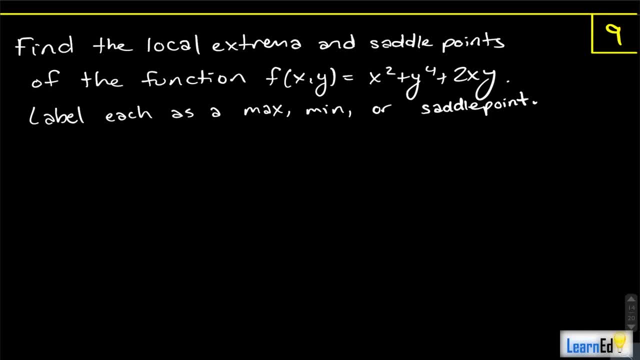 as bad as the next problem we're going to do. the whole idea of this is, if you have a point a, comma b, okay, it's going to be called a critical point of your function f, if your, if all of your partial derivatives, so all of your, you know, first, partial derivatives. 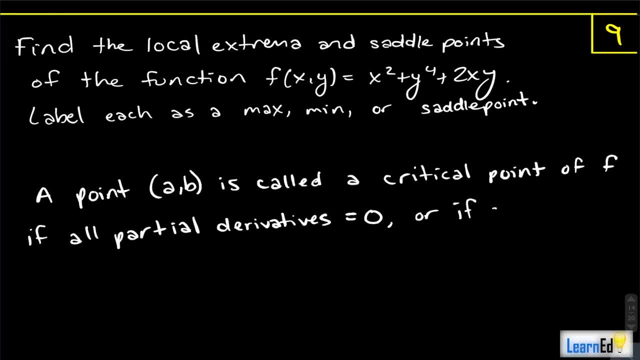 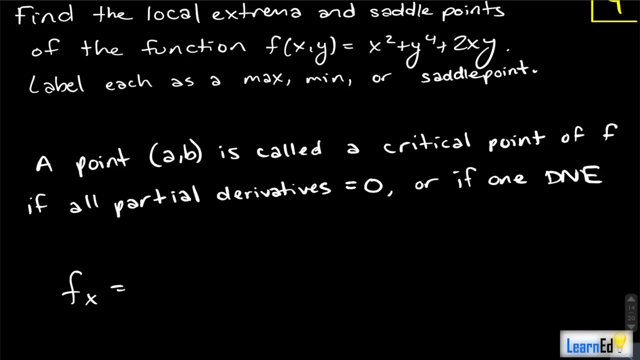 equals zero or if one of them doesn't exist. okay, so the first step is to find- no, i'm not switching back to that. um, first step is to find the partial with respect to x. partial with respect to x of this guy is just going to be 2x. 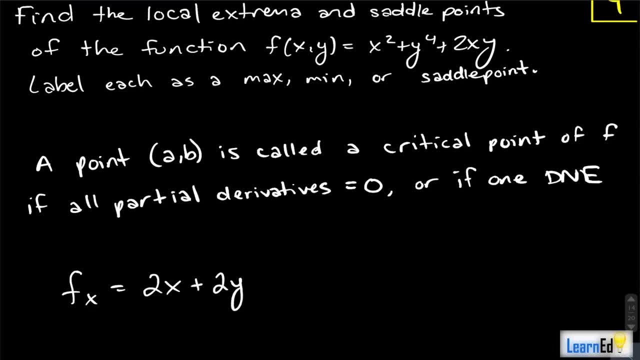 plus 2 y, and the partial with respect to y is just going to be 4y cubed plus 2x. okay, if we set these both equal to zero, we find out what values of x and y are going to make this thing". q. 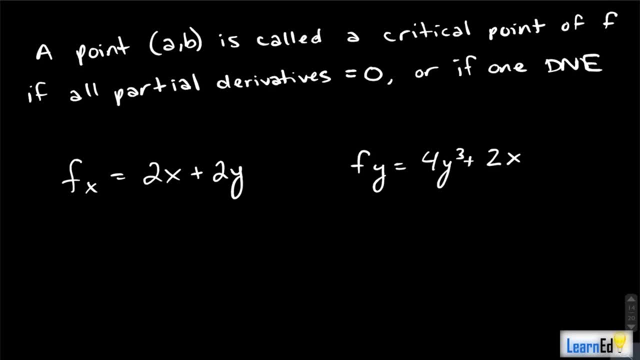 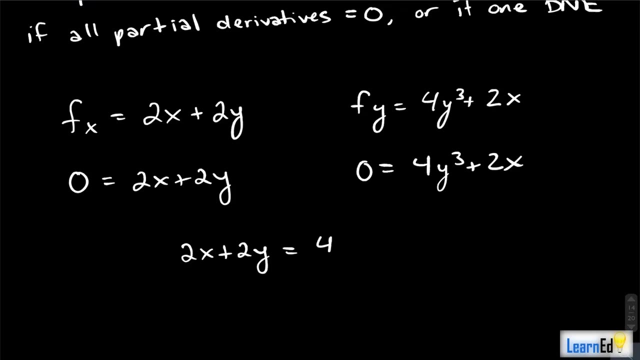 zero. all we have to do is just combine these two equations. okay, so we get 2x plus 2y, and the partial with respect to y is just going to be 4y cubed plus 2x. okay, so we find that low. okay, so we get: 2x plus 2y equals 4y cubed plus 2x. all right, so you know the. 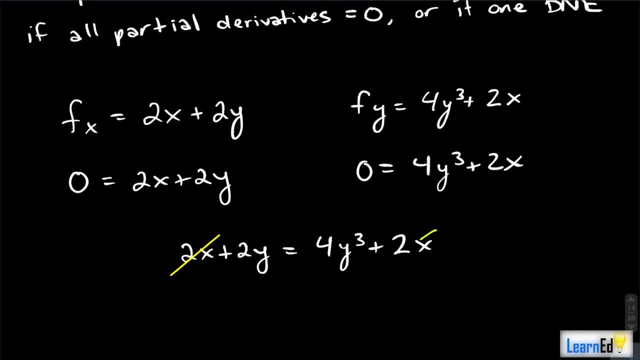 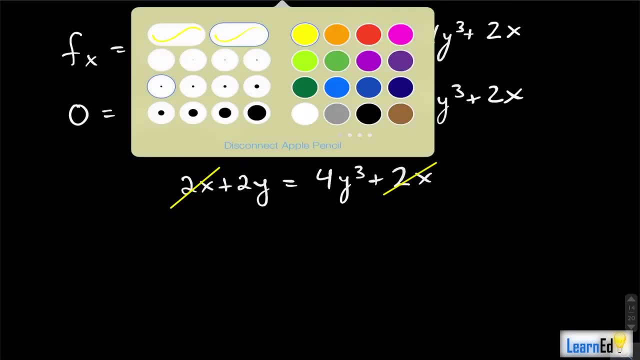 two X's just end up canceling off. right, there's two X's on each side, so these go away and you're left with- and actually the one that you're gonna have a Y cancel off and this will become a squared. but be careful when you cross. 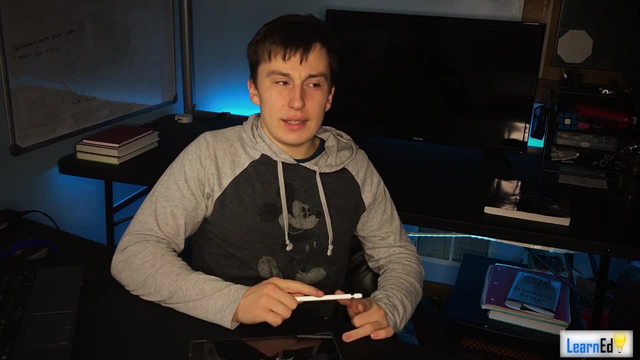 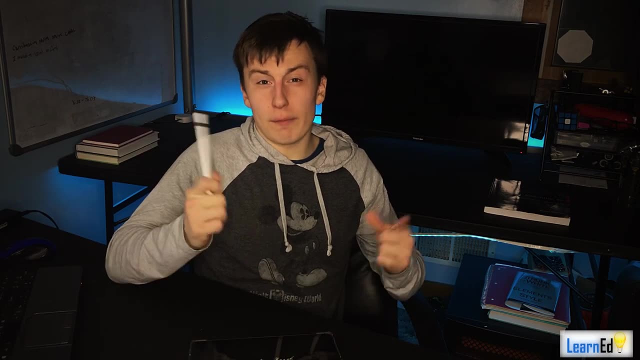 off the Y's like that: okay, it you're going to have Y can can be zero, right? so Y equals zero is a possible solution to that equation. but when you cancel off the Y's, it doesn't seem like it's any longer a solution, okay, so I want to make 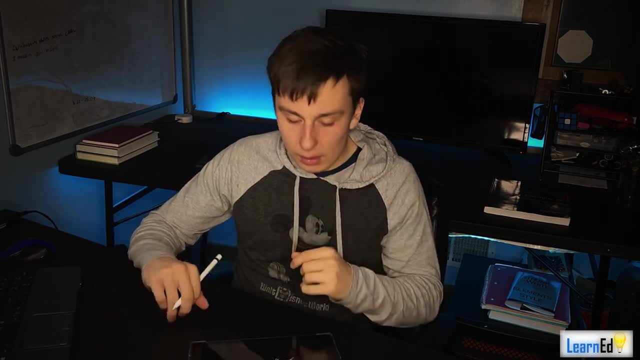 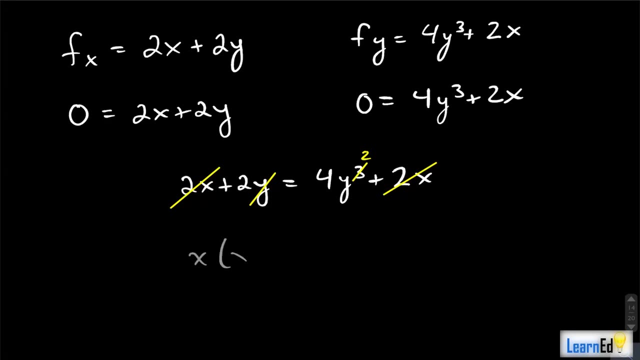 sure that you get that and let me show you an example of where that did matter. um, when you guys were like factoring and stuff and finding zeros when you were in algebra, if you have like an X times X minus 2 equals 0, you know you. 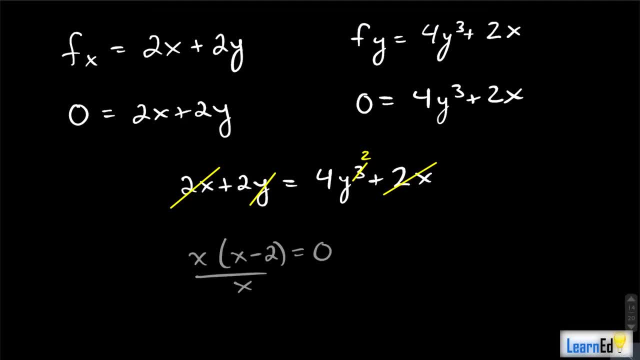 could have just divided that X right over and you could have just got X minus 2 equals 0, but then you lose one of your zeros. okay, so, um, you know, one of your your zeros is X equals 0, the others X equals 2, so when we cancel off one of 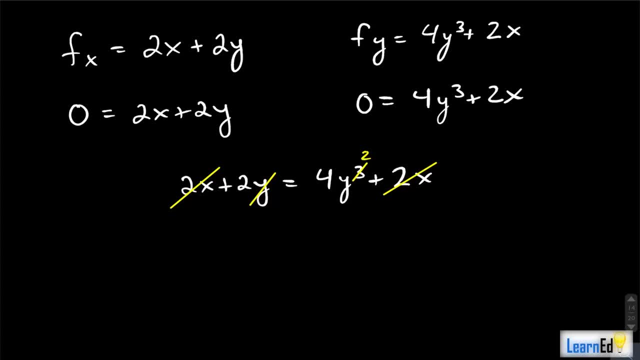 these Y's here. okay, one of our. we're losing one of our zeros, which is Y equals 0. so Y equals 0 is the solution, and we also, you know, now end up with this. 2 is also going to cancel off. actually, with this force, this becomes a 2, so we have 1 equals 2, Y squared, so we 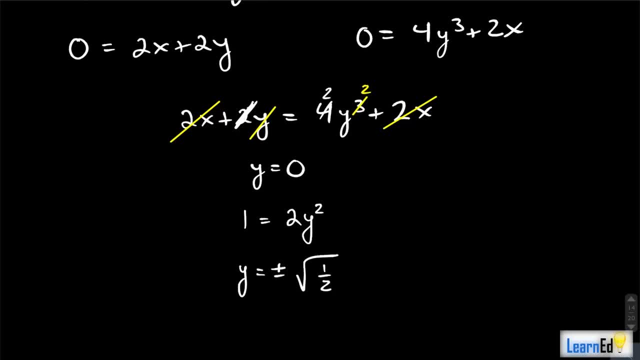 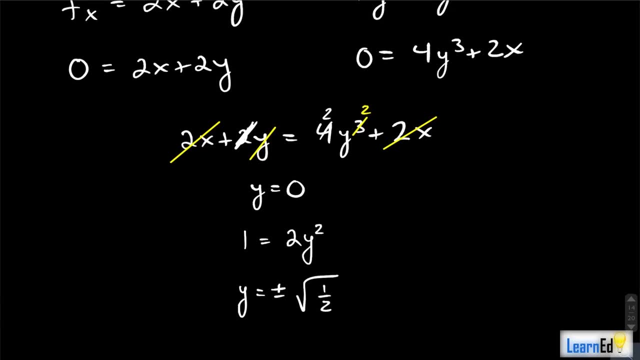 get, Y is equal to plus or minus, the square root of 1 half. okay, so if Y is equal to square root of plus or minus 1 half, then what does X have to be? well, it's kind of pretty easy to see with this equation right here: 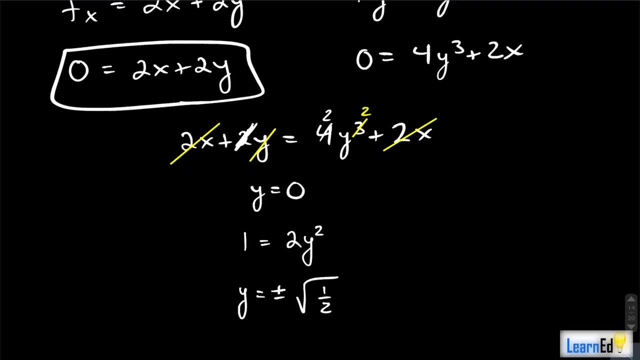 because basically X just has to be the opposite of whatever Y is okay to get 0. so if Y is this, then X would have to be minus plus the square root of 1 half. now if you're not familiar with that whole minus plus notation, like that was: 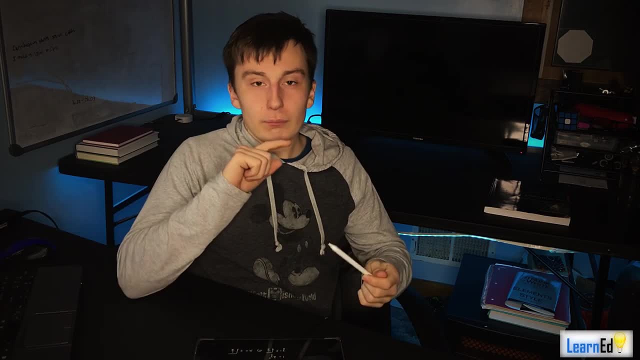 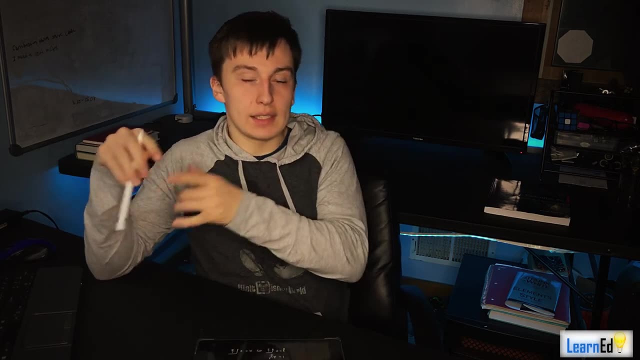 something that was introduced to me in calc 3, but you know if you're not comfortable with it. here's what it means. whenever Y is positive, the reason why we have minus plus for X is because X is going to be negative when Y is positive. okay, it has to be, though those two 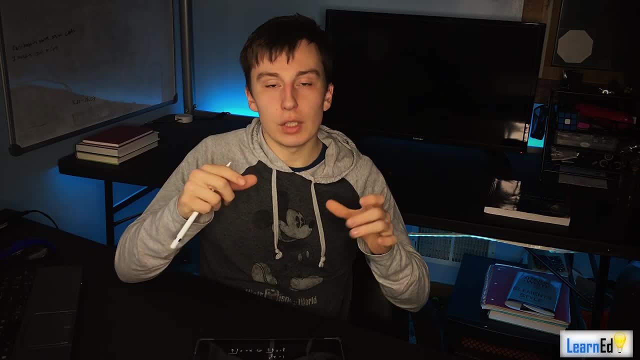 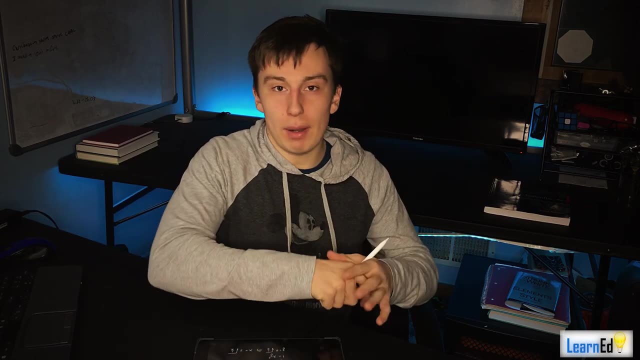 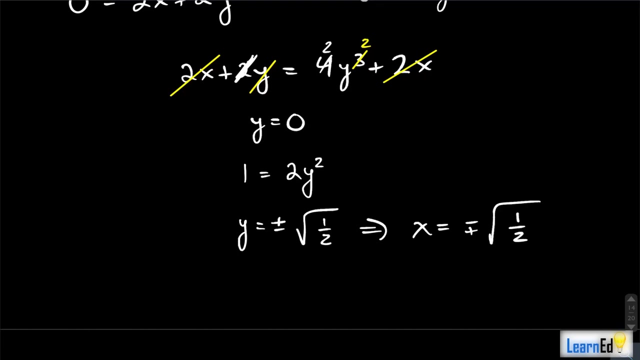 things are bound together, right so? and whenever Y is negative, X has to be positive. so that's why we flip the signs like that: it denotes that X is going to be dependent on the sign of Y. okay, so that's the idea. now, moving on, what we 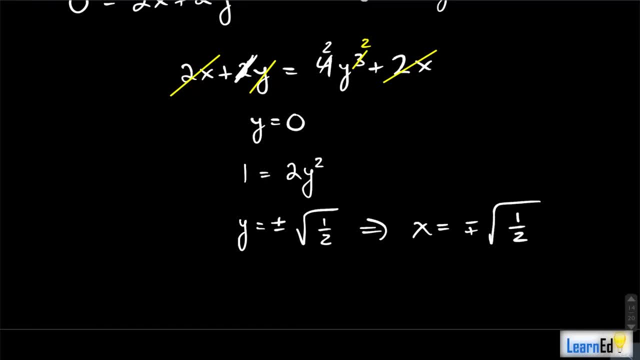 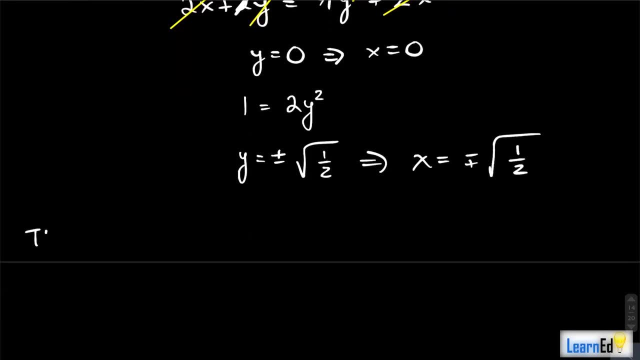 can do here. we have our roots and, by the way, when Y is equal to zero, X is equal to 0. so we have our, our three extrema and we can write those down. we have 0- 0. we have rad 1, half, negative, rad 1 half. we have negative. 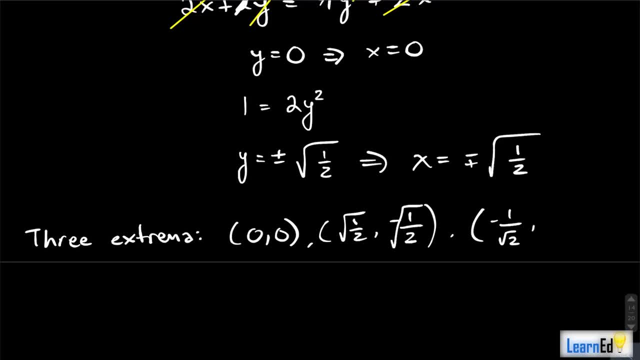 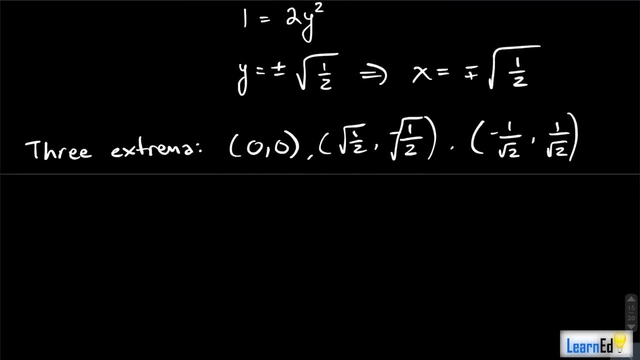 rad behalf half negative rad 1 half. so we have zero zero, we have minus whichóg, We have about学, we have abouteg of one half and then we have positive red one half. okay, and just so this doesn't confuse you guys, this is the same thing. i just wrote the same thing. these you know, the square root of one is one. 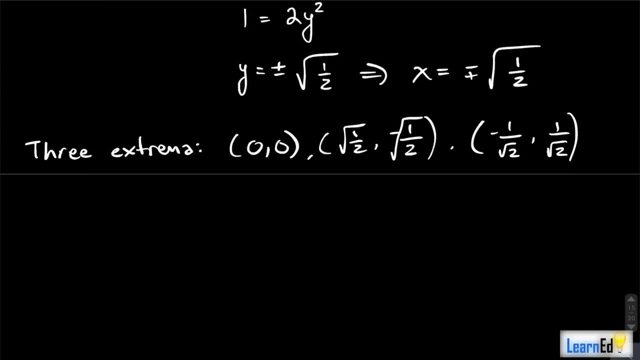 so, um, i don't know, i just felt like writing it that way. all right, so moving on, here we now, we have that, we have our extrema, we have to deal with that d thing. okay, and the basically the whole idea of d. okay, if you guys remember what the whole d thing was, 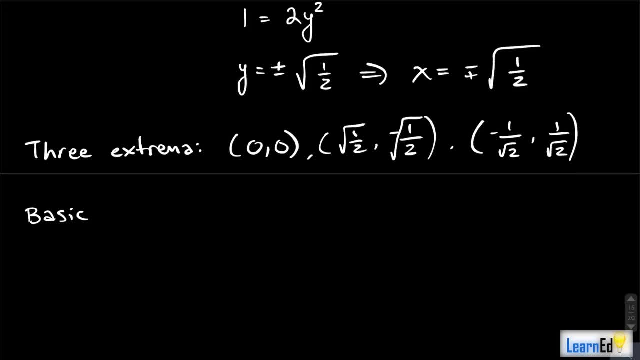 since we have the extrema, the d is going to tell us what is a max, what's a min, what's a saddle point? okay, and saddle point just means it's neither a max or a min. okay, so we have the whole idea of d, okay, and the whole idea of d is going to tell us: 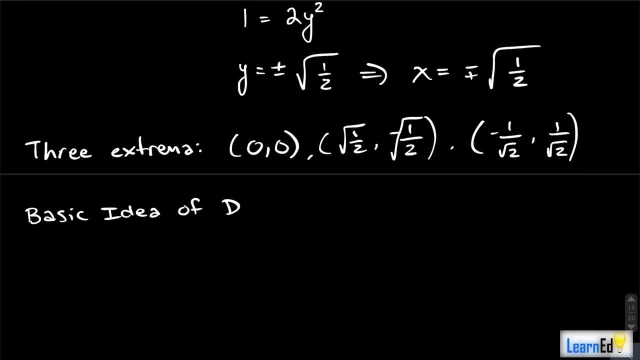 so the basic idea of d is that by analyzing all your second derivatives, you can figure out if this you know, if a certain extrema, so i'll say that instead. if a certain extrema is a max min, or you know neither, if it's a saddle point, okay, so the formula for d, all right. the 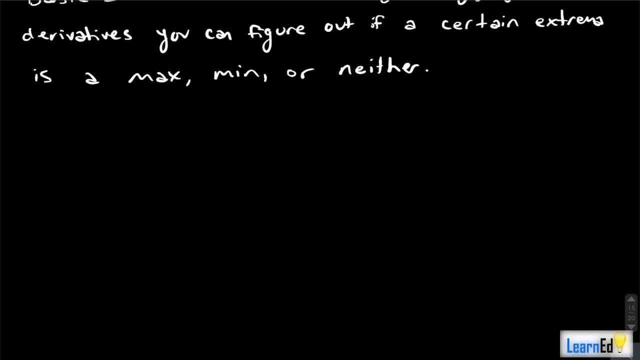 formula for d is just going to be a matrix of partial derivatives, of second partial derivatives. so d equals f x x, f y x, f xy, f y, y, and when you compute the determinant of this, you get f x x times f y y minus, and you can just write this as f x y squared, remember? uh, this is just some. 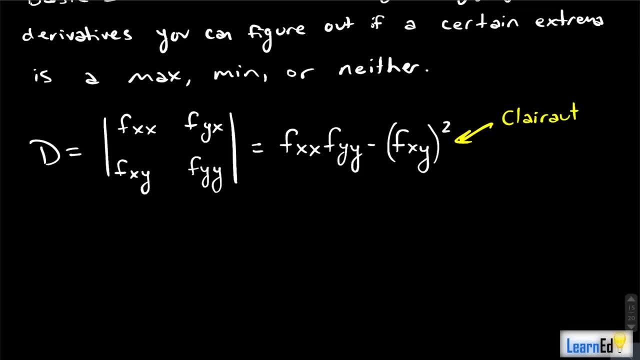 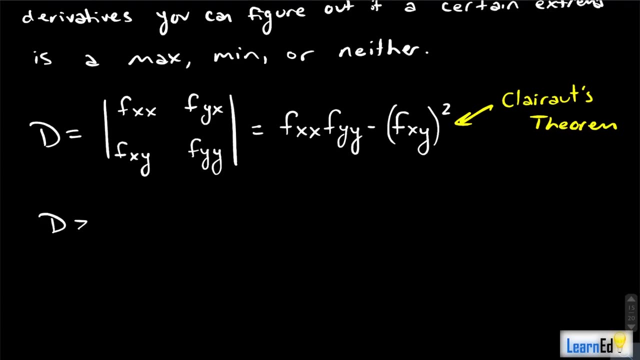 uh, this is just all from claro's theorem. really hope i'm not butchering this guy's name. i don't know. let me know if i'm in the comments. if i'm butchering this name, I feel bad, but it's all good. so, and then the rules with this is that if D is 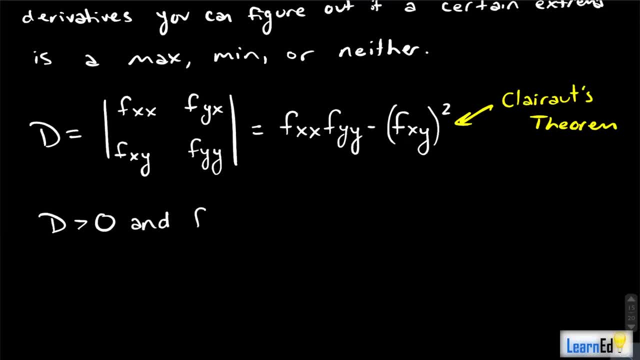 greater than zero and the double X derivative of. I'm gonna call this thing a different thing every time. if FX X is greater than zero, it's a min. okay. so if they're both positive, it's a min. if you have D is greater than zero and your 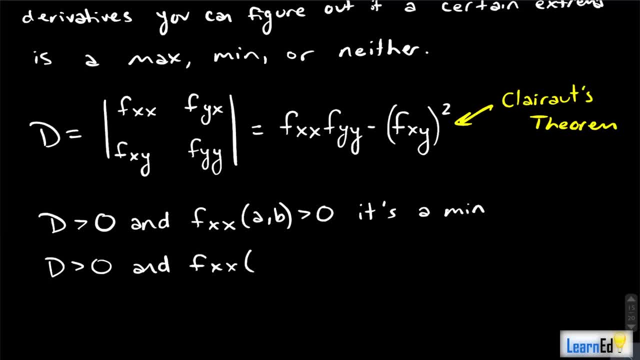 partial derivative with respect to X is your second partial derivative with respect to X. I don't know what to call it. this has been like my number one battle this whole video. I was not ready for that. and D, unless if D is less than zero, it's a saddle point. so those are the conditions we have to meet and you. 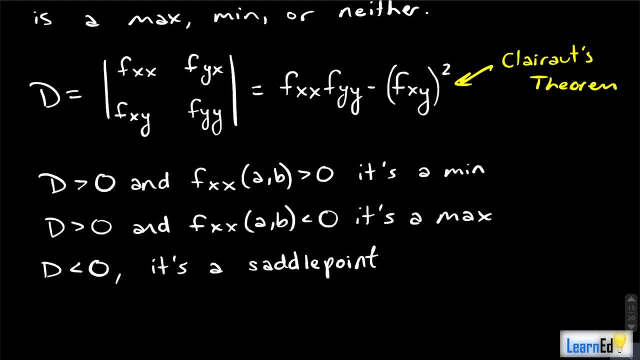 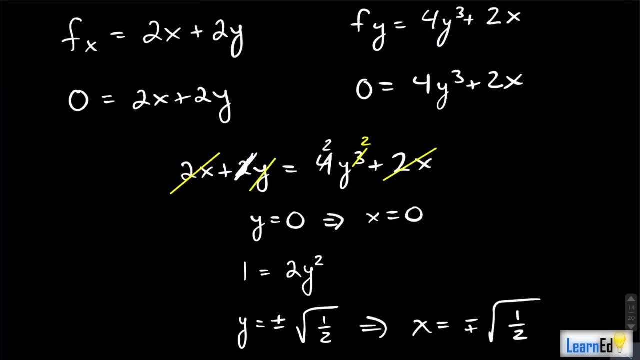 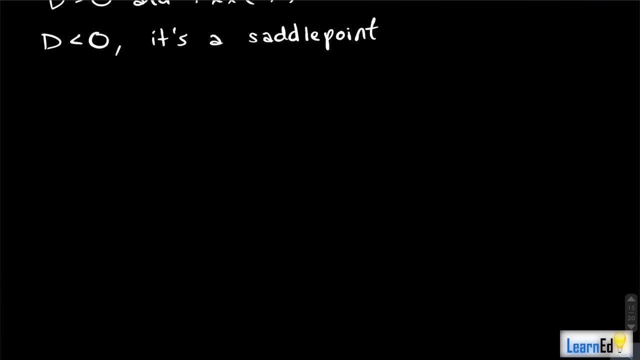 probably already have these in your notes, but I just kind of want to go over that again because this is very important. so let's bring down our partial derivatives and then we're gonna find the second partial derivatives. okay, and whoa, what am i doing? that was weird. 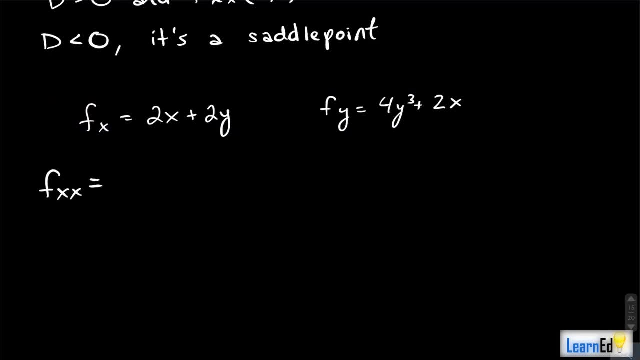 our partial, our second partial derivative with respect to X. X is just going to be to. our second partial derivative with respect to Y is going to be just twelve y squared, and our partial with respect to x and y is going to be: well, we, we just go with. 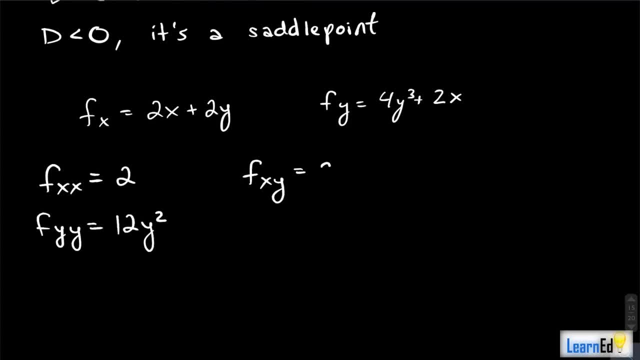 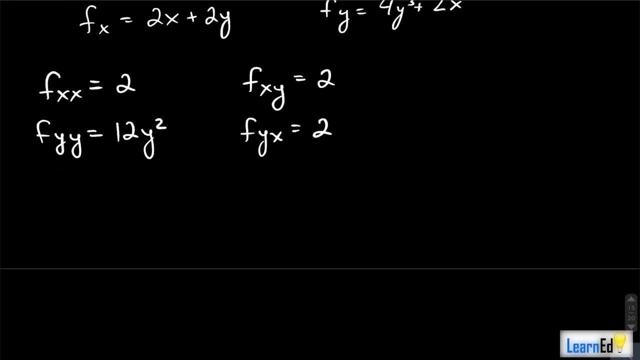 that this is just gonna be to again. so you know that means that that's also going to be F of Y, X. but we're gonna make our matrix now: 2: 2, that's not 2, that's 12 y squared, put in the exact. 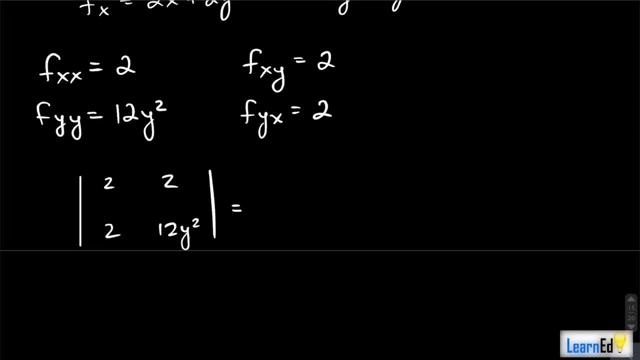 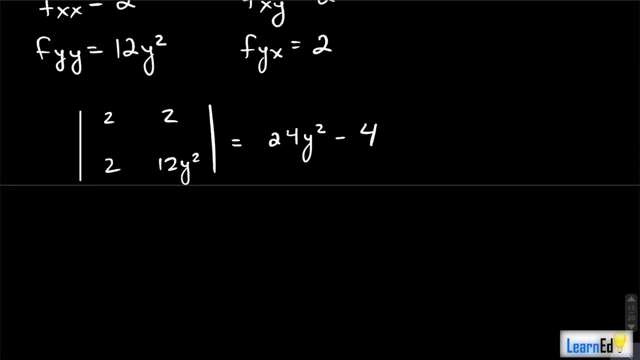 wrong place, you guys. you guys can tell that I'm getting tired out in my videos, I swear. alright, so we got 2 times 12 y squared, which is 24 y squared, and then you have subtraction 4: okay, and now we have our, our function for D. okay, we have. 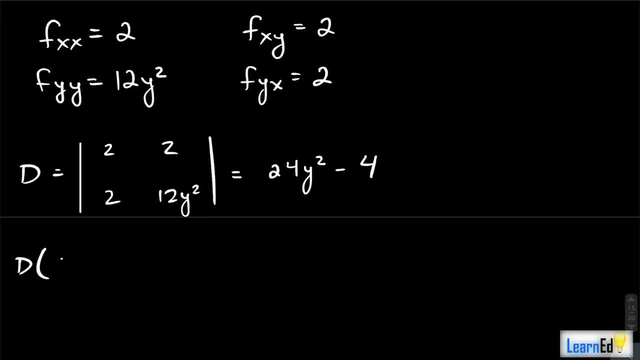 our function for D. so now we have to analyze D at each of our extrema. first, we're going to analyze it as 0 comma 0. as 0 comma 0, this is just going to be negative 4, which means that that extrema is going to be a saddle point. 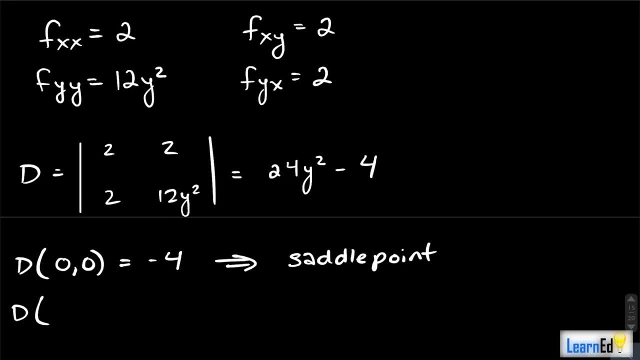 okay, D at 1 over rad 2: square root of 1 half: same thing. negative square root of 1 half is going to be equal to well, we just end up this Y squared. I mean it's gonna. it doesn't matter if this is negative or positive, so this is going to. 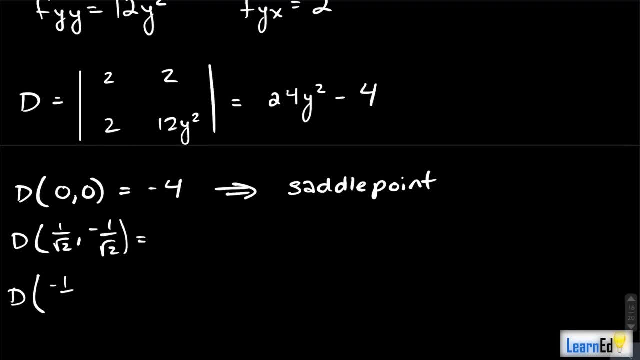 be the same for both this extrema and the next, which is this guy. okay, and you, basically, that'll just end up being 1 half when you square it, and so you'll get 8 and 8. so now you have to look at your partial, your second partial. 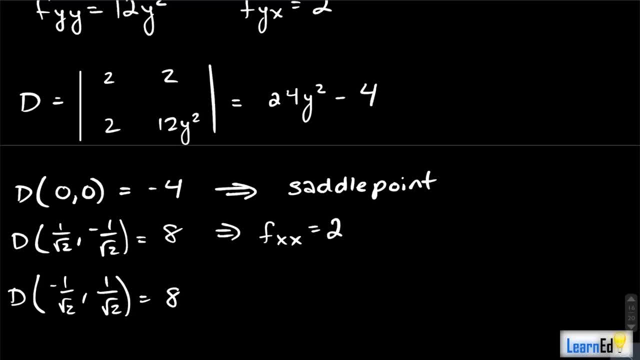 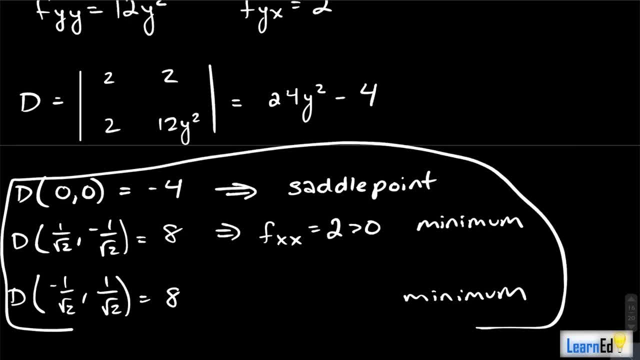 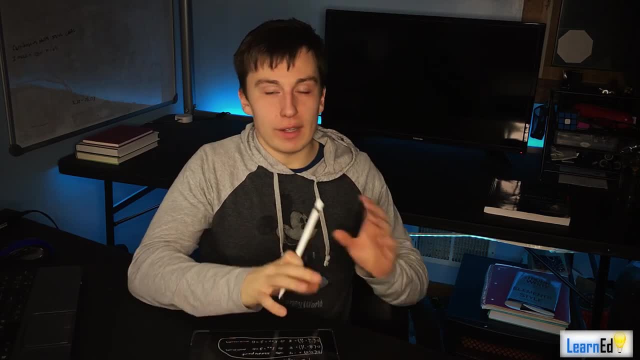 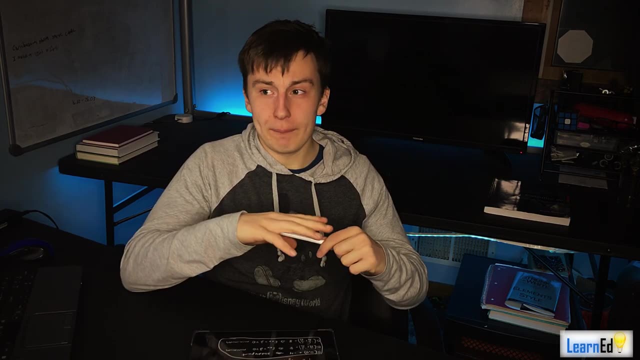 partial derivatives, seeing when they're equal to 0, what values of X and Y can make them 0. and then you're going to proceed with calculating that D function okay, and that is just the determinant of partial of second order. if you just live by this. 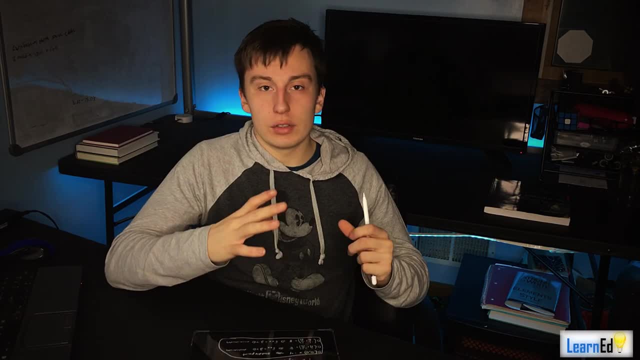 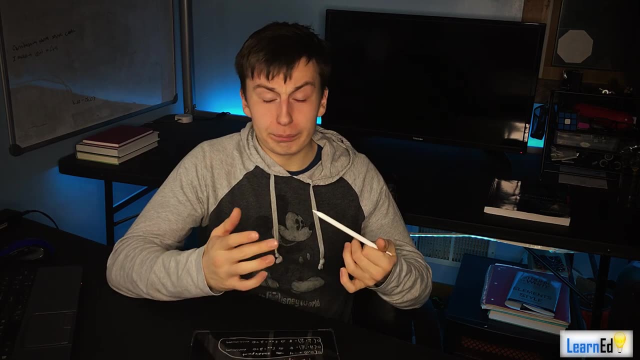 partial derivatives. so you're using those second partial derivatives to analyze whether these things are a max or a min. okay, and you know that's pretty much exactly how it works for uh, calc, one or one of the ways that you can see if it's a max or a min. right, you're analyzing the. 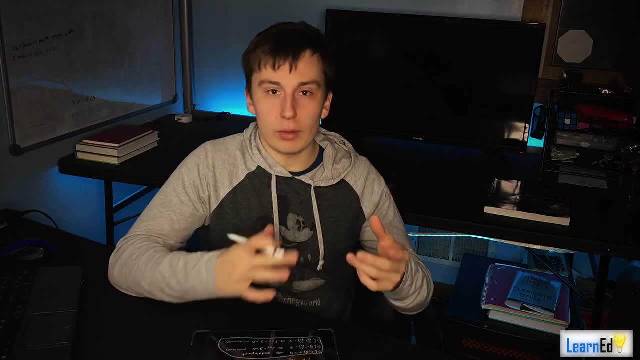 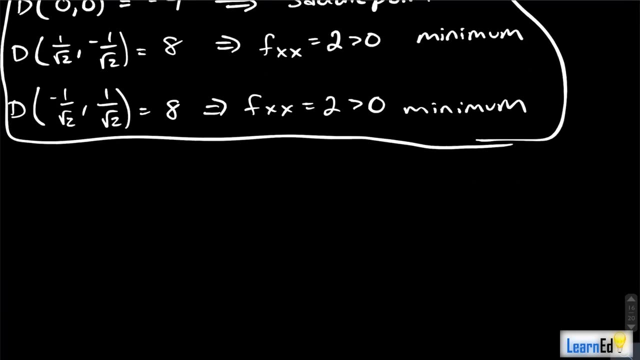 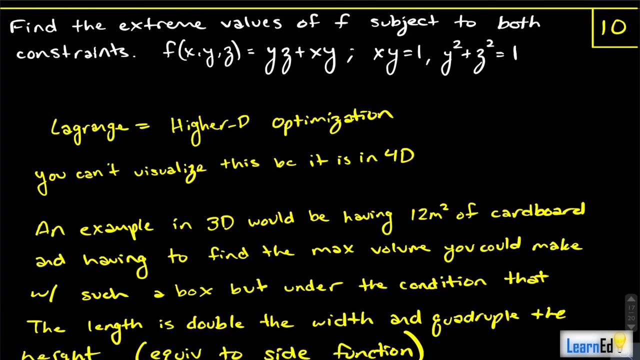 second derivative, okay, but now you have multiple second derivatives, so that's why there's a matrix of it. okay, that's the the gist of it. so now we're going to get into our last problem, and this is going to be a lagrange multiplier problem. okay, which everybody loves. this is everybody's favorite. 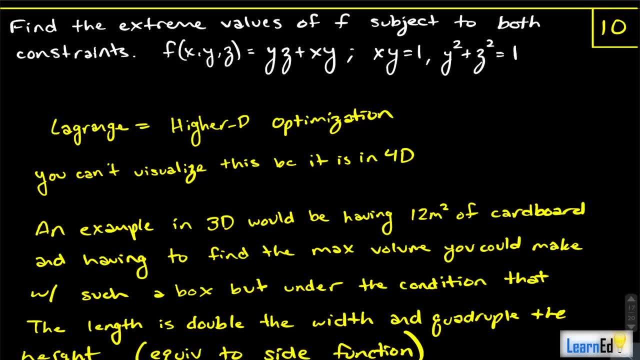 topic in calc 3, aka nobody's favorite. so basically the the question here is: we need to find the extreme values of f, subject to both constraints, and our function is of x, y and z, and it's y, z plus x, y, and our two constraints are x, y equals one and y squared plus z squared equals one. 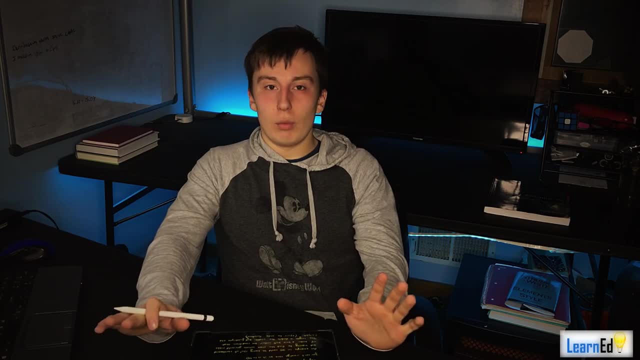 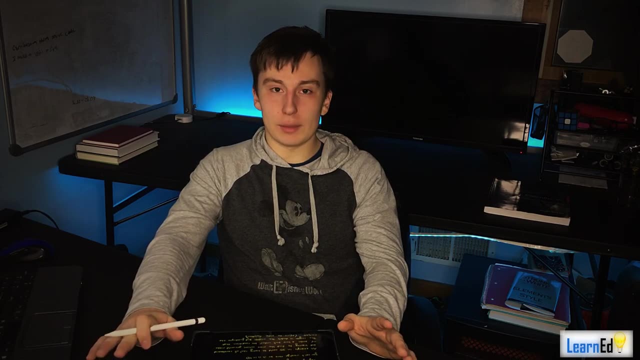 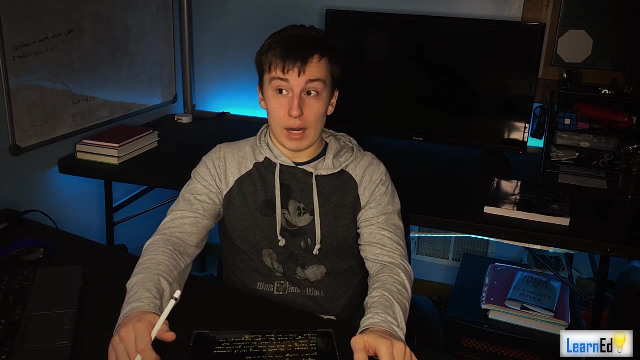 now, first off, hold up. what's a lagrange multiplier problem? okay, seriously, i guarantee you that most of you have no idea what lagrange multipliers are actually doing, and if i said that i knew what lagrange multipliers were like two hours ago, i would be a complete liar, like i had no. 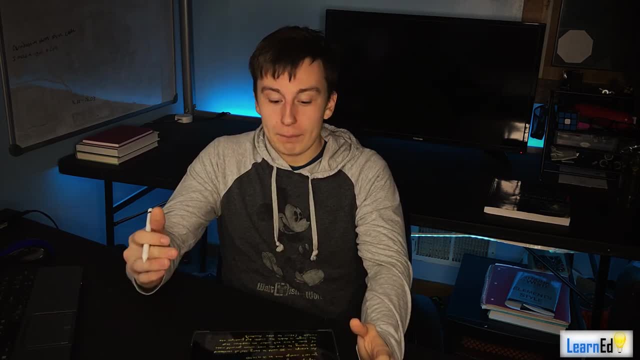 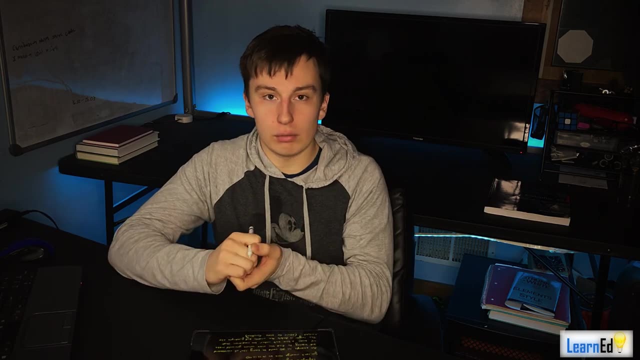 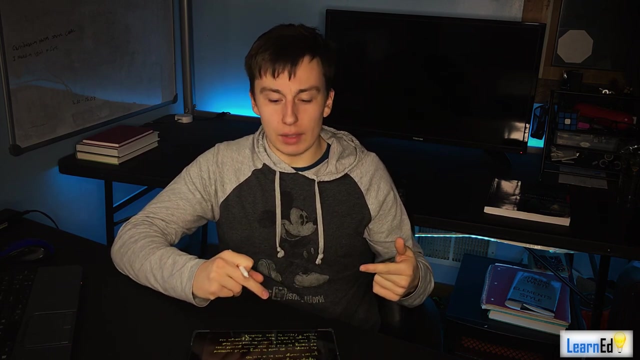 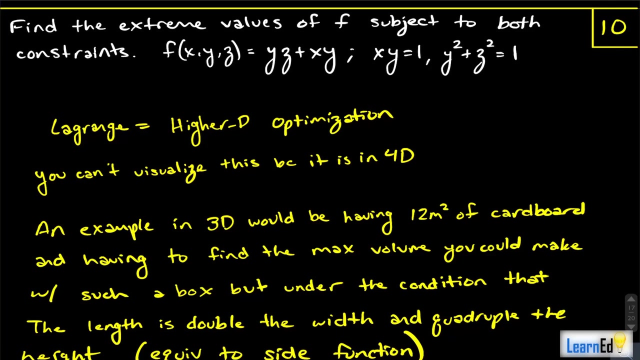 idea what they were actually doing. i just knew how to do them right. basically, what lagrange multipliers are, without getting into too too much depth, is their their higher dimensional optimization problems? and let me give you an example of like a way that this could actually be applied in real life. okay, um, but i can't use this example as uh an example, because, uh, you're. 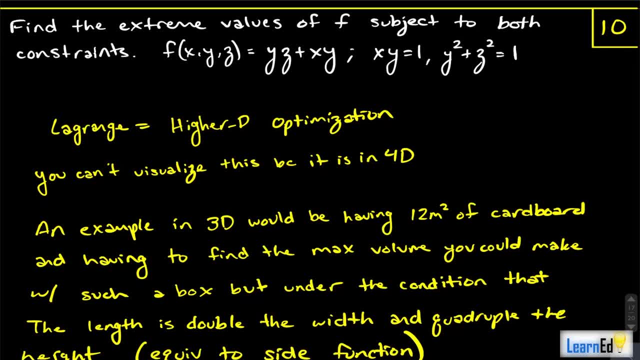 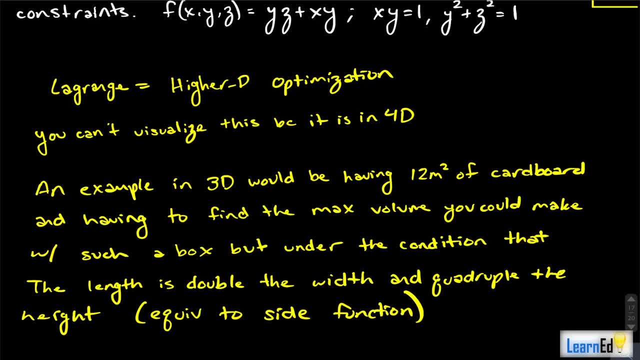 not going to be able to visualize it because it's in 4d. i could probably talk about, like mass density, but that's not something i'm ever going to do, uh, because i don't want to so and it's confusing. so here's kind of an example. 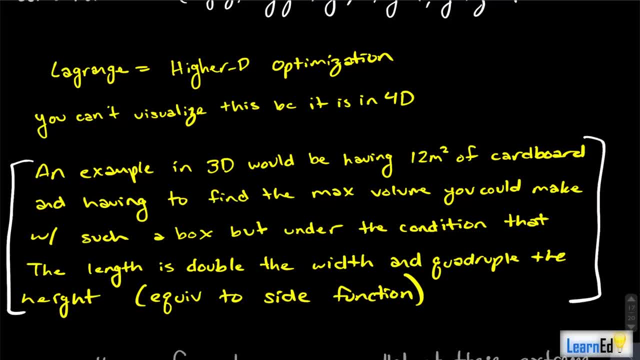 right here. an example in 3d would be having 12 meters squared of cardboard okay. so you got 12 square meters of cardboard and you have to find the max volume that you could make with such a box, but it's under a condition, okay, and that's kind of the whole. this is kind of like the. 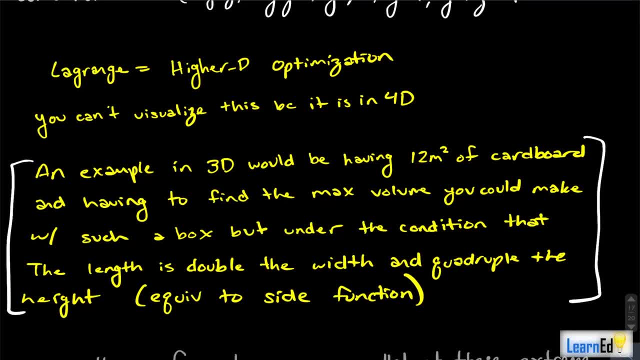 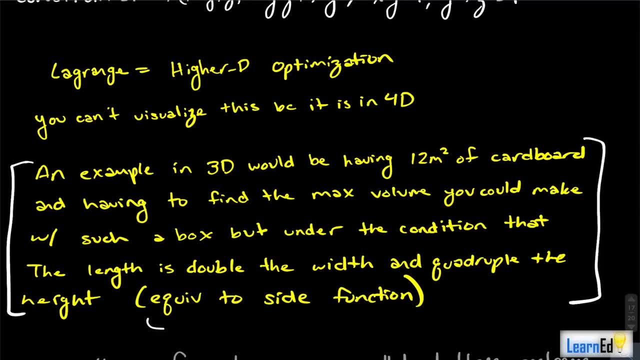 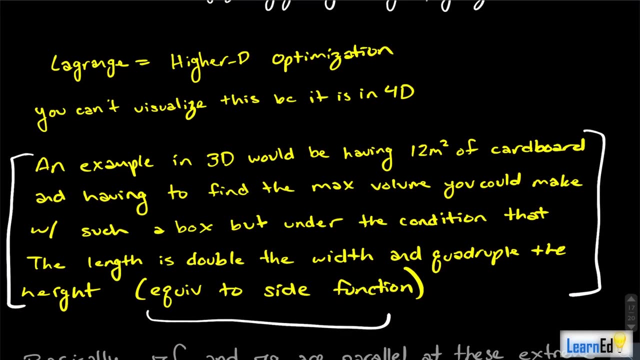 whole calc 1 optimization stuff. okay, it's under the condition that the length has to be double the width and quadruple the height. okay, this is the equivalent to a side function. in this case, we have kind of two of these side functions right here. okay, so we have two constraints, all right. so these are just optimization problems and we all know how. 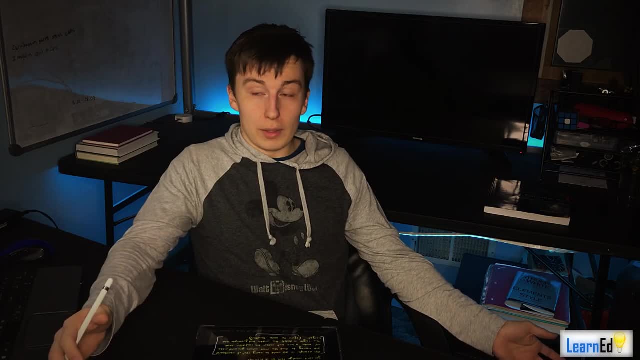 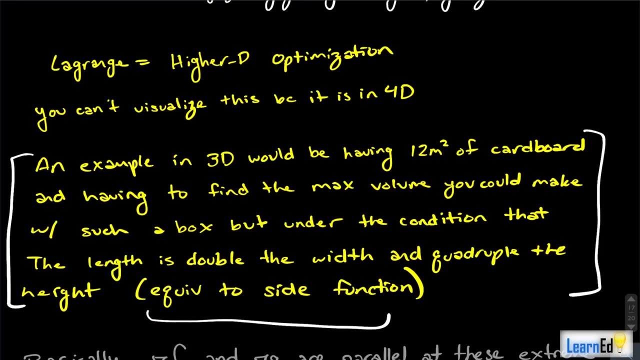 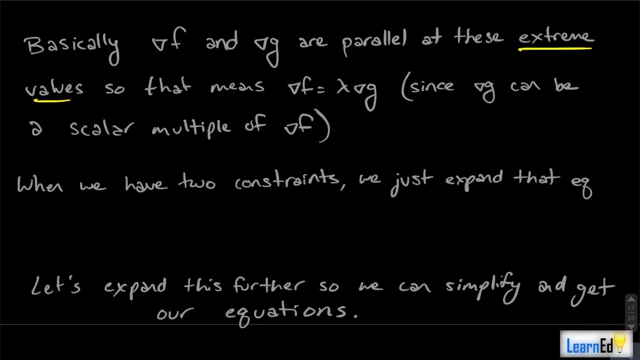 many people loved optimization in calc 1- nobody. so how do you think it's going to go over for lagrange? honestly, like it's. i mean sucks, like i didn't like doing it and here i am teaching it so cool. so the idea now and kind of getting into the application of this stuff, 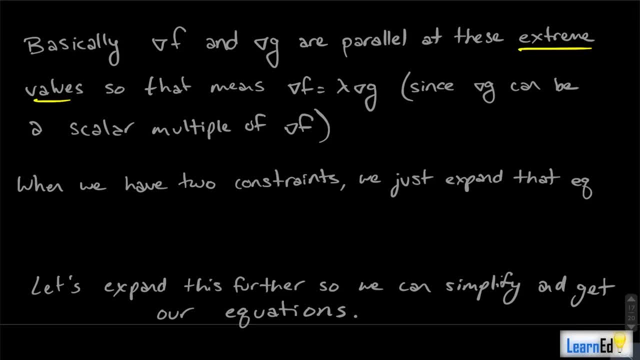 and uh. so i'm not gonna again, i'm not gonna go into too much depth here, uh at all. basically, let's say you only have one constraint, and your constraint is um a function g okay, and your regular function is f, del f and del g are parallel. so the gradients of these two things of your 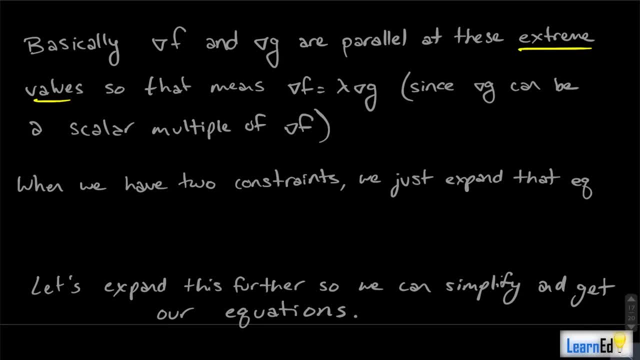 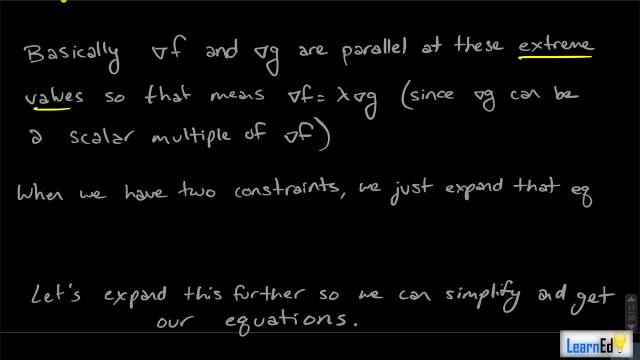 regular function and your constraint are going to be parallel at these extreme values that you're looking for. right, you're finding extreme values. so that means that basically, del f can be a scalar multiple of del g. okay, so we put a lambda there to denote that it's scalar multiple, right? if these things are parallel, they don't. 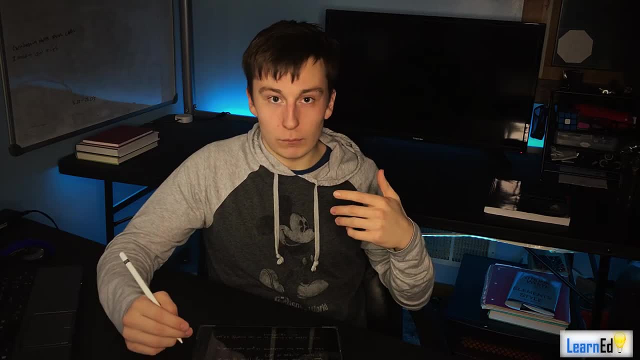 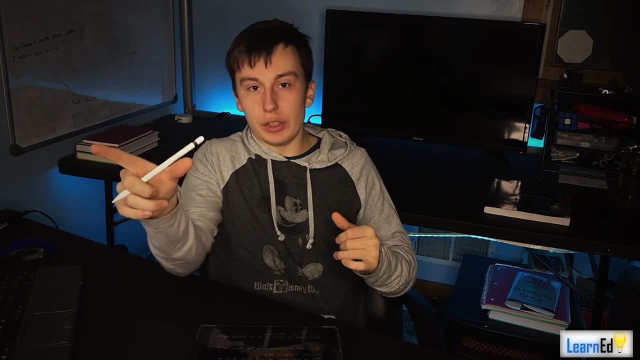 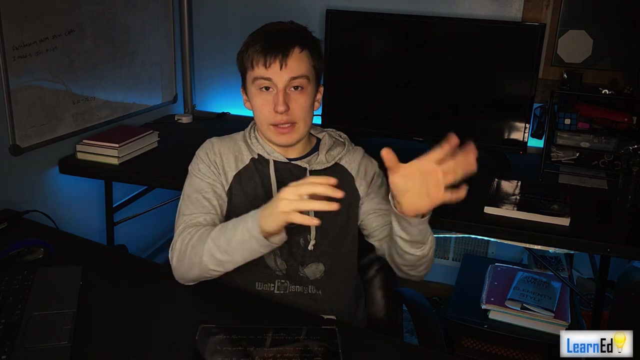 have to equal each other. they can just be a scalar multiple of each other. right, like it's saying. it's like saying it's the same thing as saying, like a unit vector, like, let's say, like one, two is equal to some scalar times two, four. right, this one on the on the right hand side right here is just double. 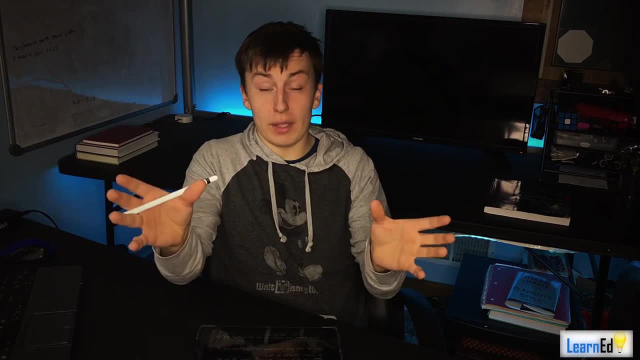 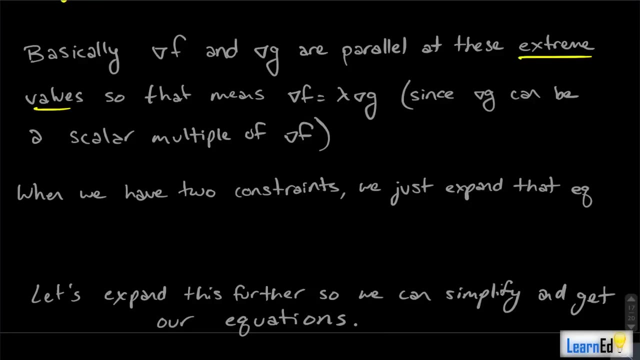 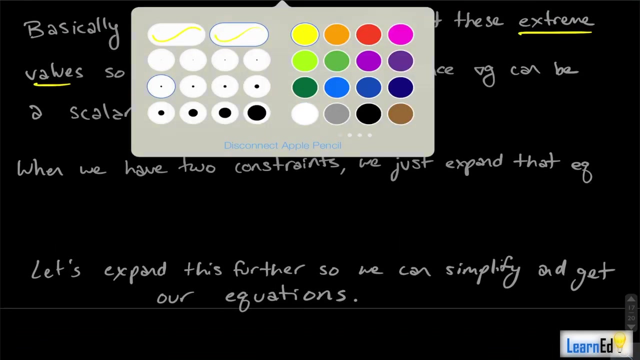 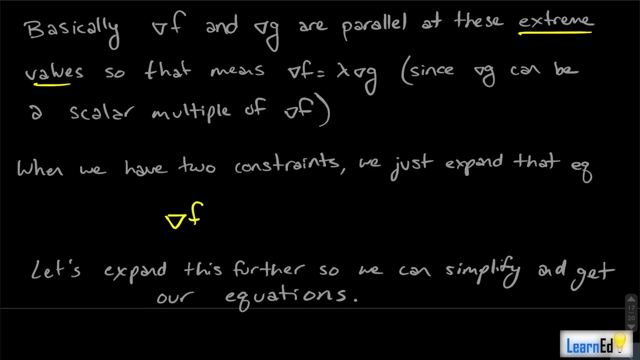 the other one. okay, so these two things are parallel, right, they're both pointing in the same exact direction, but they have different magnitudes, and that can happen, okay. so when we have two constraints, we can just expand that equation. so what we get is that f equals lambda del g plus and our second scalar is going to be mu. okay, this is what most people 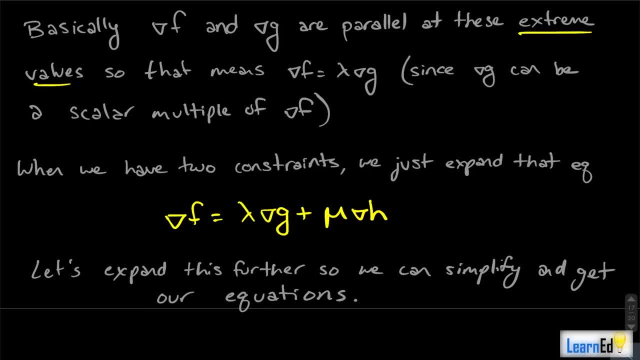 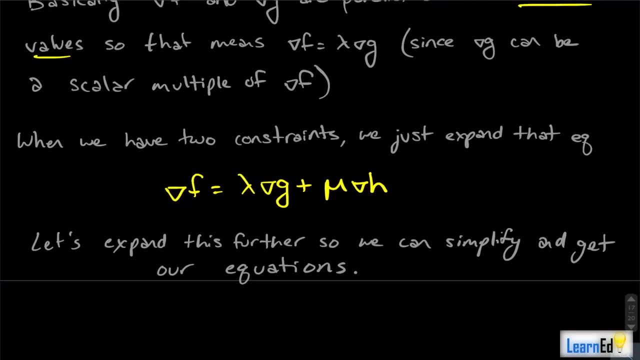 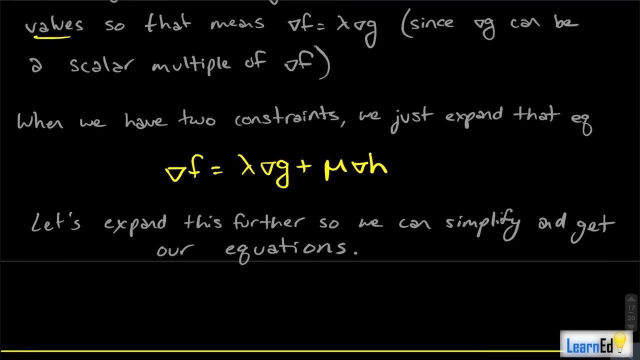 use and we're going to have del h. okay, and we're going to expand this further so that we can simplify and end up getting our equations okay. so, expanding this out, we get that. the gradient is just well. the gradient of f is just this, right, our partial x, partial y, partial z. 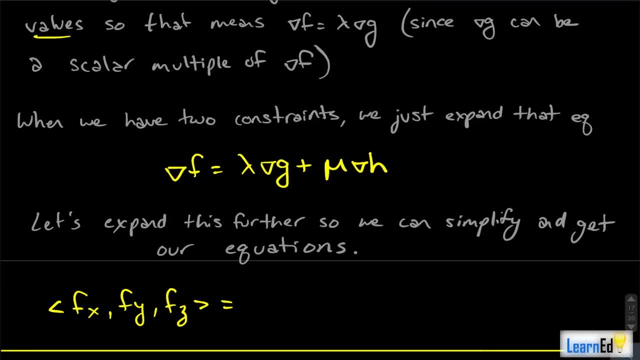 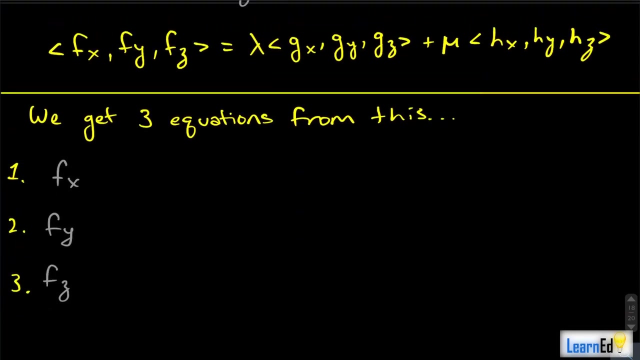 and that's equal to lambda times the gradient of g, which is just g x, g, y, g, z. okay, plus mu times h x, h, y, h, z. okay, so now You can get three equations from that. okay, You can say that, okay, well. 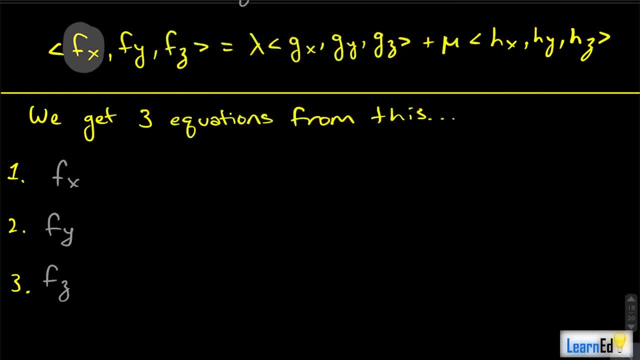 you can do this component-wise in essence. So fx is gonna be equal to lambda gx times mu hx. Okay, that's your first equation. So fx equals- I'll do this in gray- fx equals lambda gx plus mu times hx. 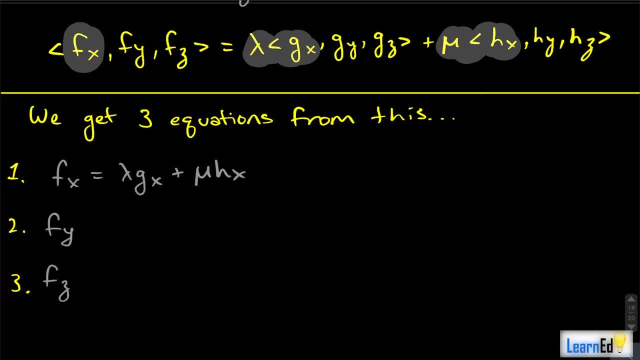 All right, so that's your first equation. Your second equation is just going to be fy equals lambda gy plus mu hy, right? So the mu, just the scalars are just getting distributed, if you haven't already figured that one out. 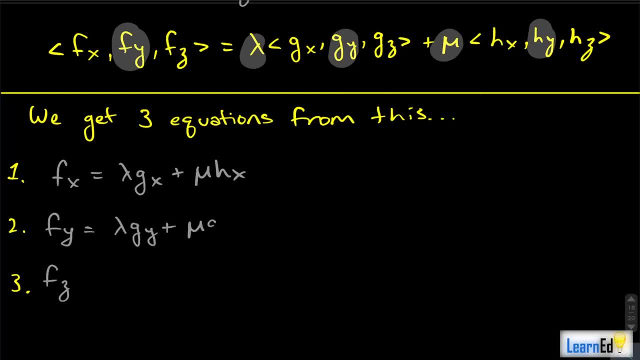 This is equal to just lambda gy plus mu hy, And fz is equal to lambda gz plus mu hy. Okay, so that's how you get your different equations. You just do this thing component-wise and you're fine. Okay, so we can get our equations. 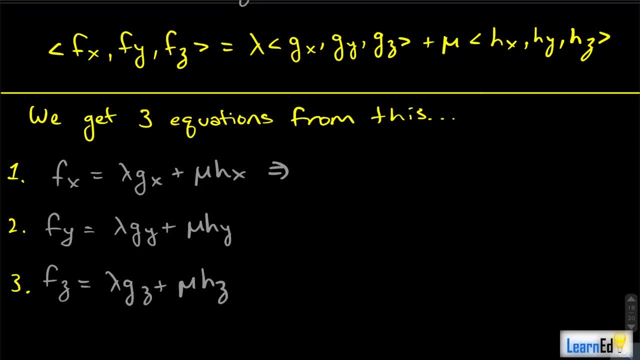 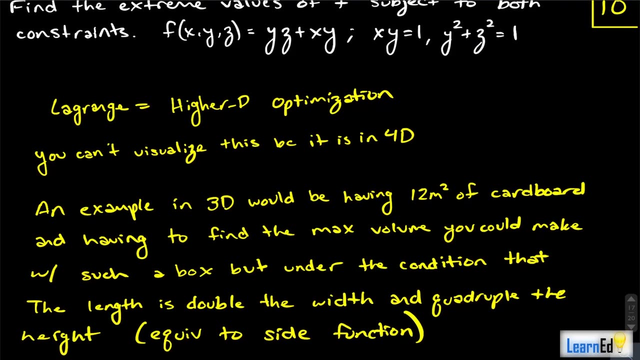 for all our we can actually do out our equations now. So what is our partial with respect to x of f? Well, what Actually? let's? here's what I'm gonna do, because I'm not scrolling up every time. 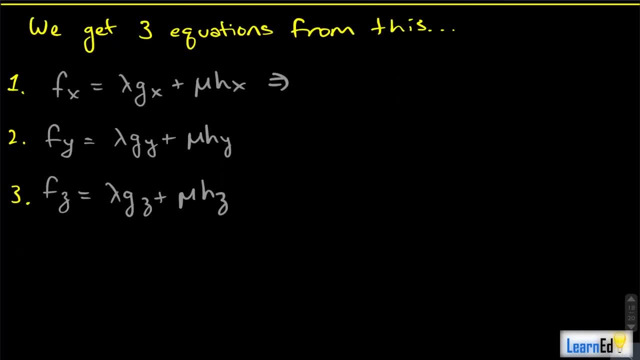 I'm just gonna bring these guys down, So I'll bring this down right here. Okay, so now we have our different constraints And what I'm gonna do, so I'm actually gonna break this up a little bit, because we gotta figure out. 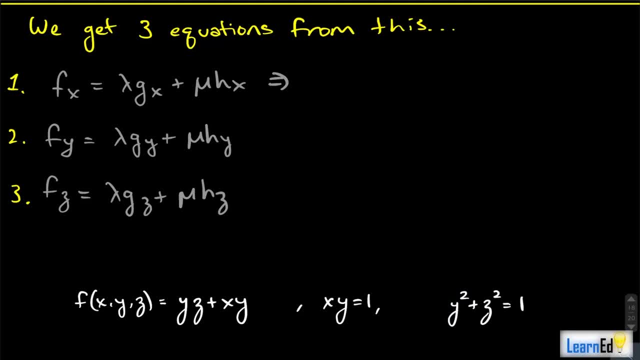 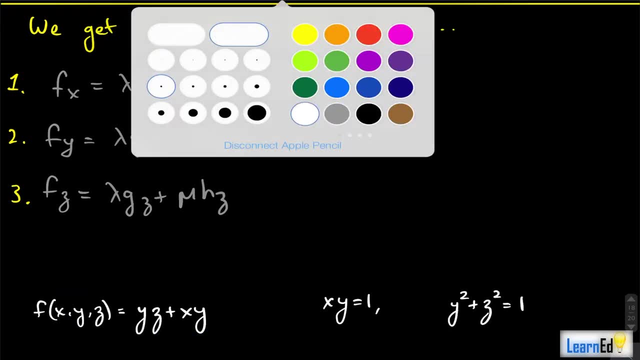 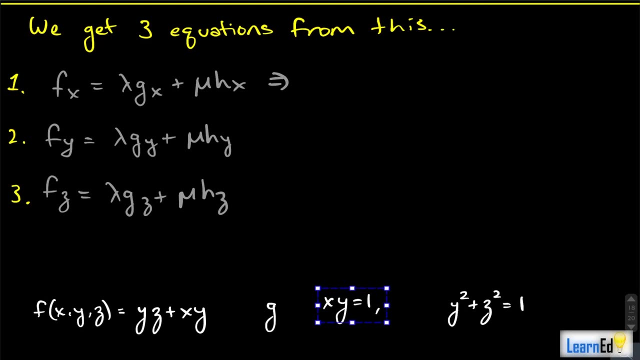 what g and h are. okay. That's maybe something you've been wondering is: what is this? So? if this is f, Okay, Then this guy is g. So g is going to be a function of x, y and z. 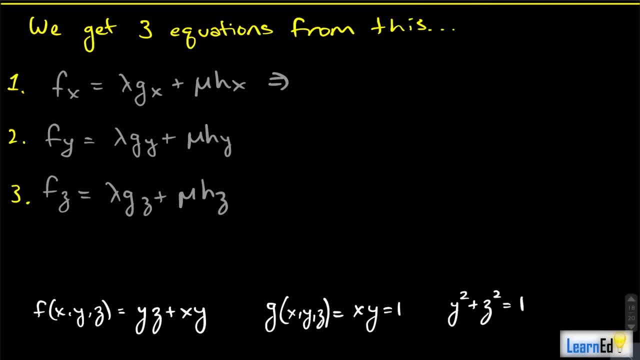 It's equal to that which is also equal to 1.. And you may be wondering: okay, well, you're not doing anything with the 1.. The 1 will come in later. all right, It will come in later when we actually are doing all the algebra. 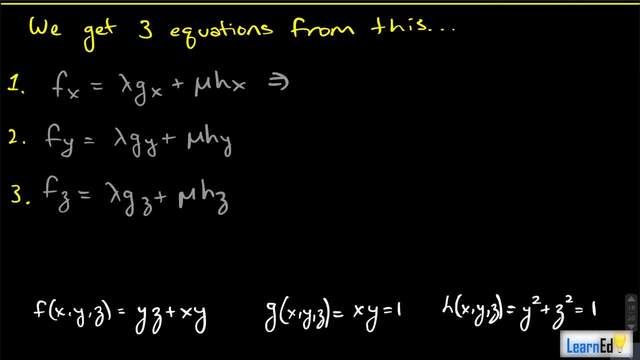 And there's your function h, like I said, and that 1.. And the h equation will also come in later, So we're not going to use it for now, but it will come in for useful later. The partial derivative of f with respect to x is just going to be y. 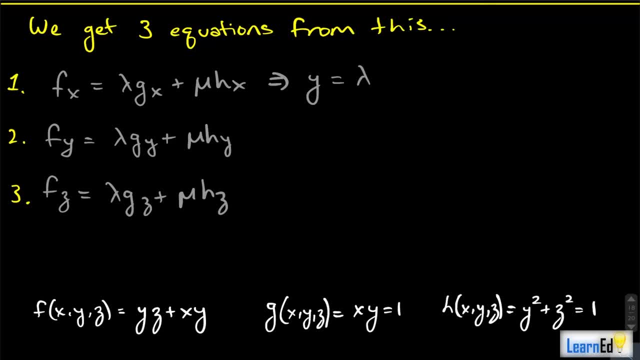 And lambda will stay there. The partial derivative of g with respect to x is going to be y. And then we get mu. The partial derivative of h with respect to x is going to be 0. So we can actually just get: y equals lambda y. 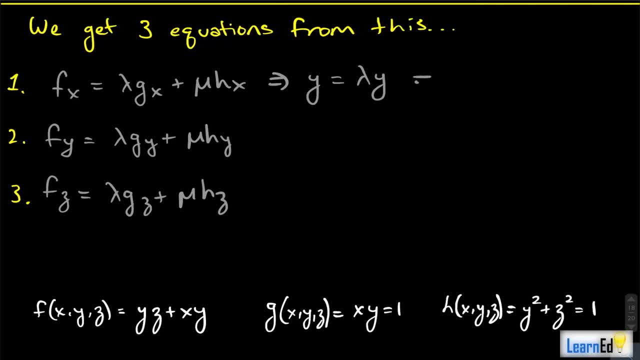 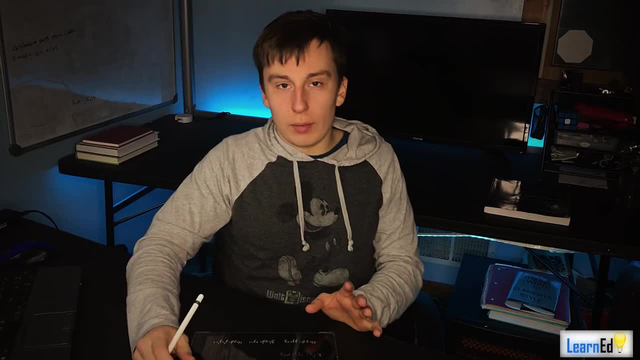 And if we divide both sides by y here we get that lambda equals 1.. Okay So, and by a quick reminder, lambda cannot be equal to 0.. Don't be like one of those people and just put your scalar as 0. 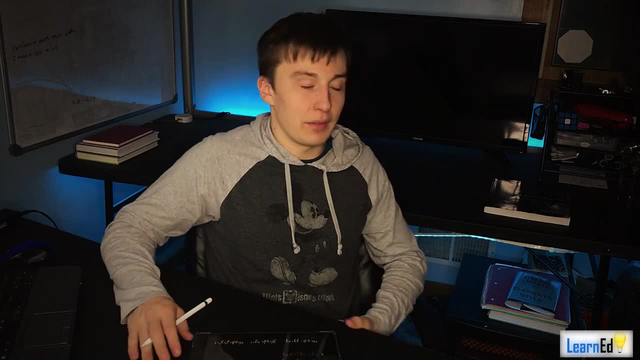 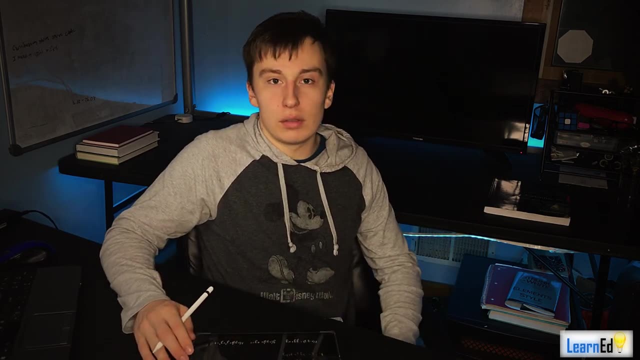 because that's not something that works with Lagrange multipliers. Okay, your scalar isn't 0. That would be trivial and that wouldn't be meaningful at all, So we're not going to make our scalar 0 here, Okay. 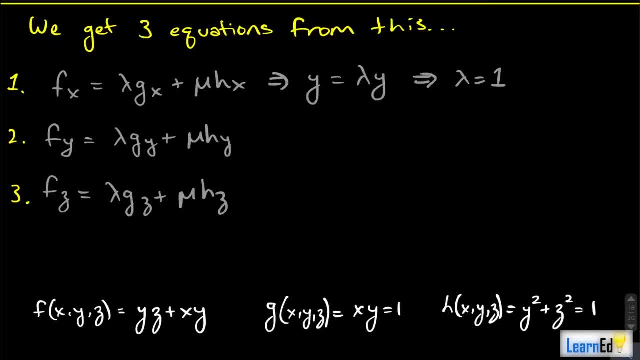 And you can research more about that if you're interested in exactly why we can't use 0.. But yeah, it just ends up being like a meaningless quantity. Anyways, let's move on to our next part. We have the partial of f with respect to y, is just going to be z plus x. 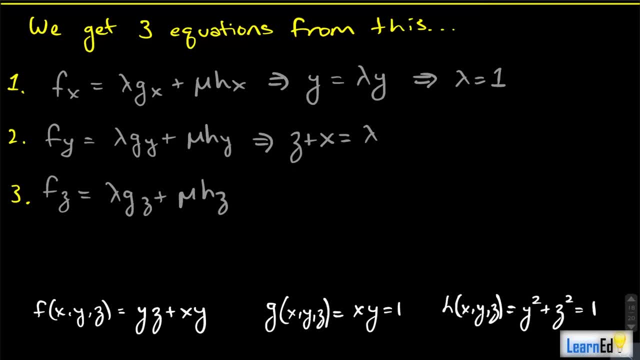 And that's going to be equal to lambda times, the partial of g with respect to y, which is x, And then we're going to add the partial of y with respect to h, No, sorry, the partial of h with respect to y, times mu. 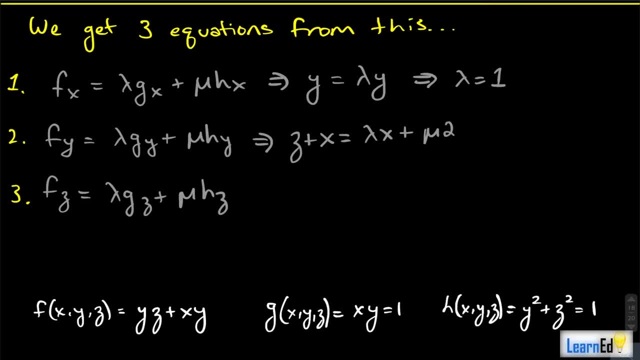 So that's going to be mu times 2z. Okay, Then we have our last one. So we have the partial of f with respect to z is y. We have that. this is equal to the lambda times, lambda times, gz, which is 0.. 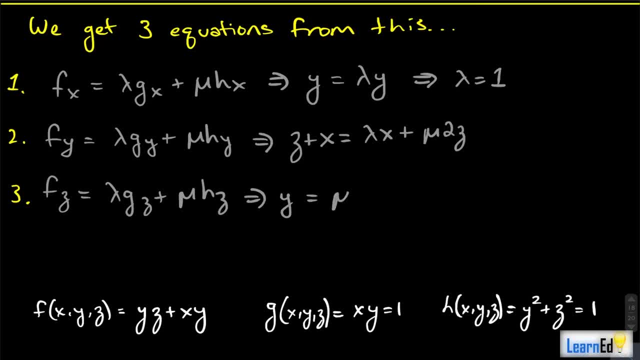 So this lambda will just go away. Then we have mu times hz, which is 2.. That'll just be 2z. I apologize, I think I made a mistake With respect to y. this is not 2z. 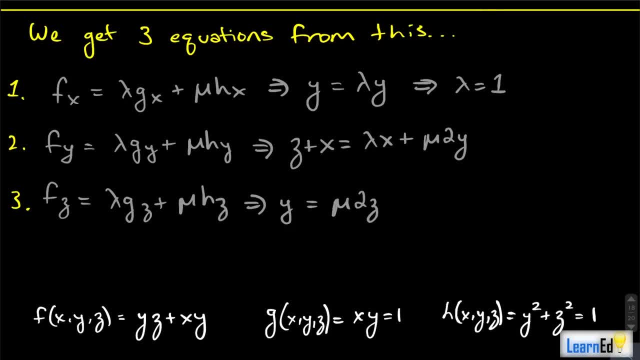 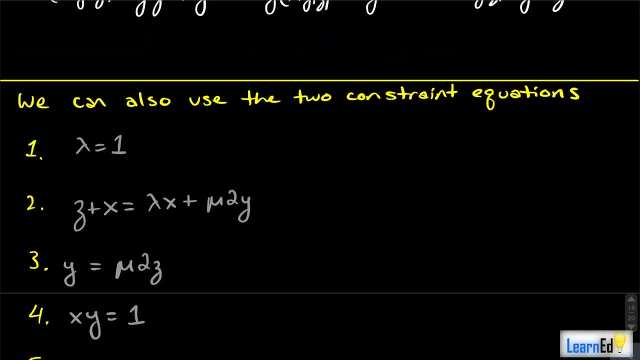 This is 2y. So now that we've solved these guys, all we have to do now is bring in our two constraint equations from before, And this is where I said that you know this 1 and this 1 will actually become significant. 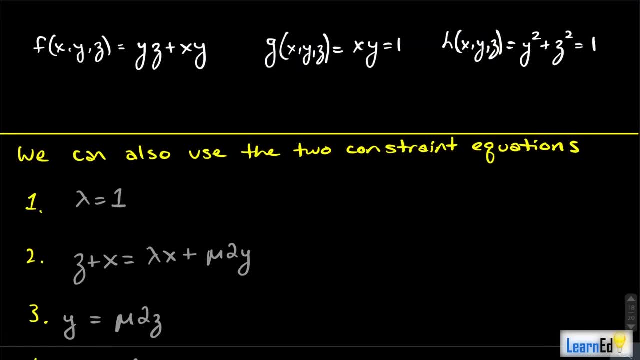 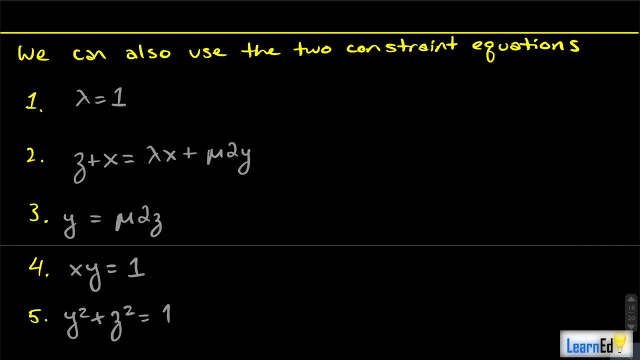 because now we're going to actually use them. So our two constraint equations we have xy equals 1 and y squared plus z squared equals 1.. We're going to use all five of these equations. Okay, If you have, If you just had lambda you didn't have, like. 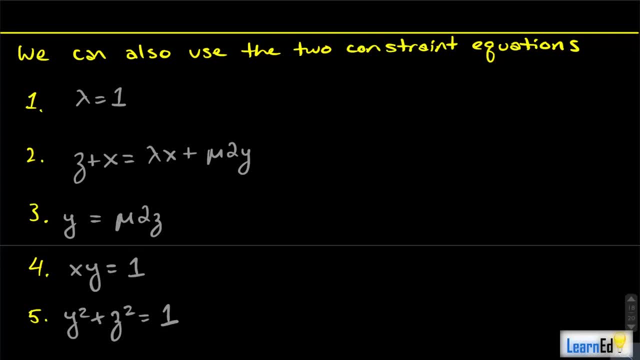 You didn't have an extra constraint equation. You would just have four equations, Okay, So you know that's something To always remember. It's you know, the amount of equations that you have depends on how many variables you have. 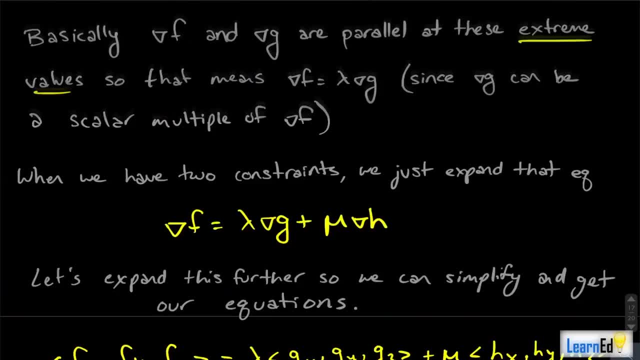 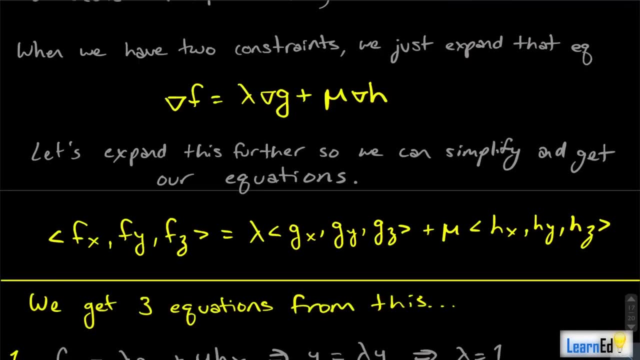 Like, if you, In this case we have a, We have a three-dimensional function, Okay. So we have those three variables x, y and z, And then we have lambda and mu. So we need five equations to solve for five variables. 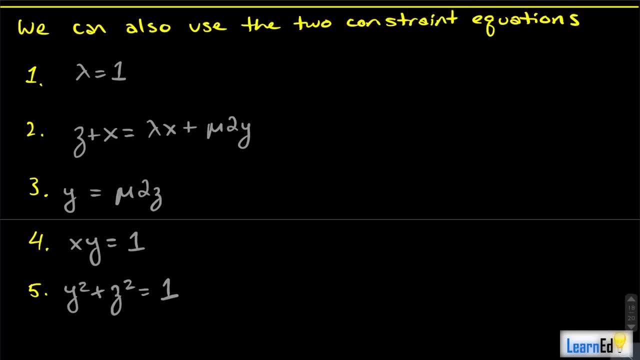 But we don't actually need to solve for lambda and mu. We can just find x, y and z and be done, All right. So let's move on to actually. Let's start solving for these guys And If we want to simplify this guy a little bit, 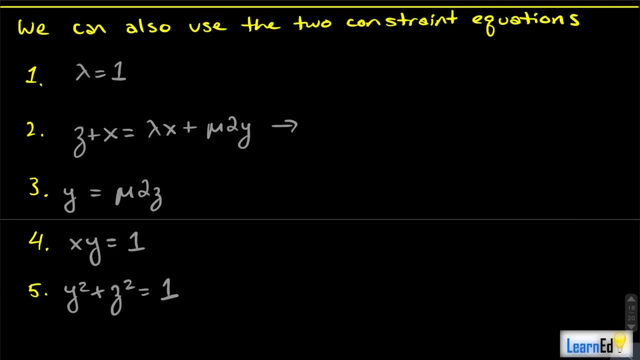 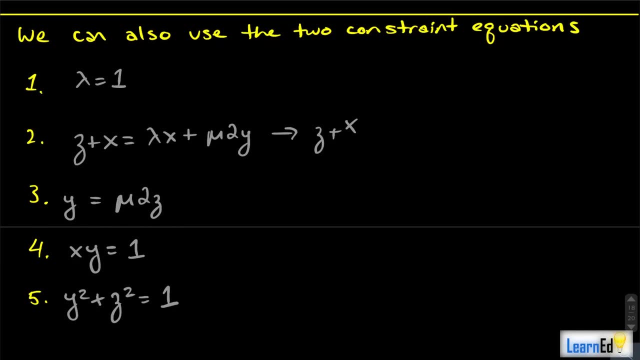 we can just say that z plus x- Sorry, that was a little messy. We can say z plus x equals lambda- is 1.. Okay, We already found that up here, which is just. you know it's useful. So we can say that this is x plus mu times 2y. 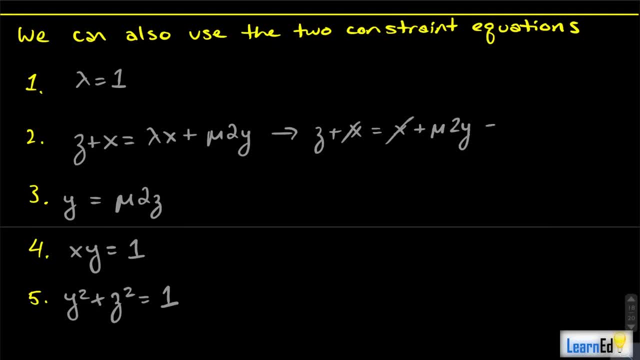 Okay, And the x's will just cancel off here. So we get that z is equal to mu, or we can just write this as 2mu y. Okay, It looks a little nicer that way. Now, if that is the case, 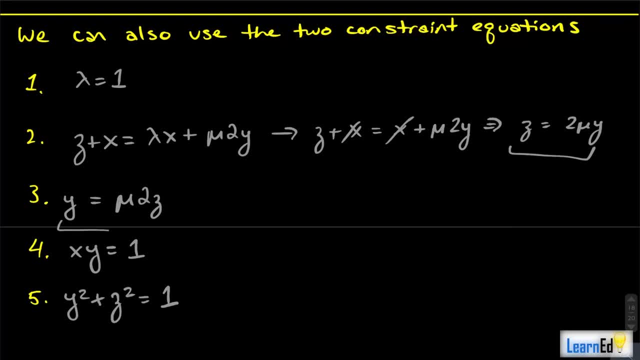 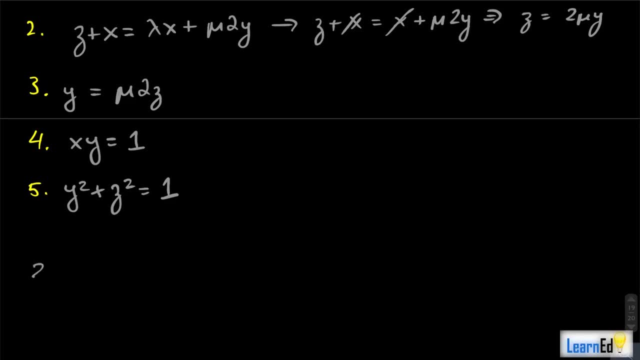 then I mean this looks pretty similar to equation 3.. So what I'm going to do is I'm actually going to divide these two equations and see what we get. If I divide 2 and 3, I get z divided by y equals. 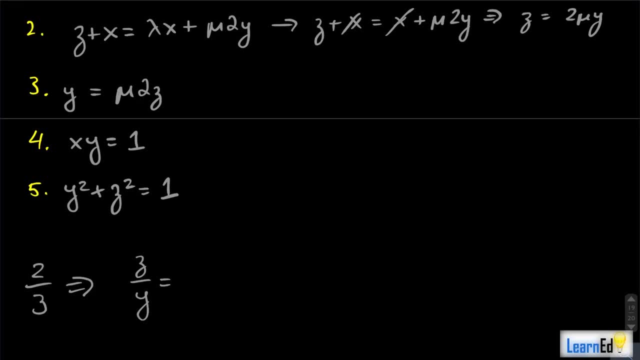 The mu goes away and the 2s go away, We get y over z. So what we get is that z squared equals y squared, And I'm not going to solve for z and y, because, Because what it can do is just plug these guys. 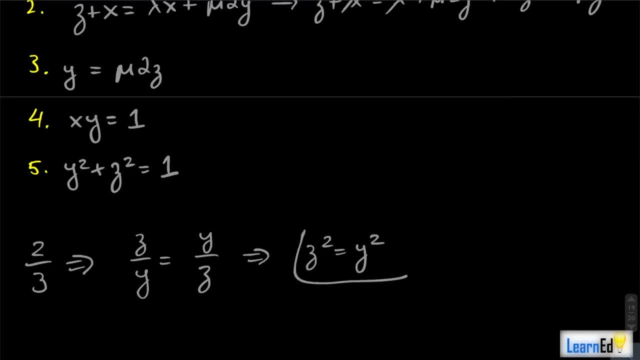 And this is what you need to watch out for. I have this and I don't want to like make my life harder by just squaring both sides or anything, So I'm going to use this equation over here, Okay, Because I can just plug these in right here. 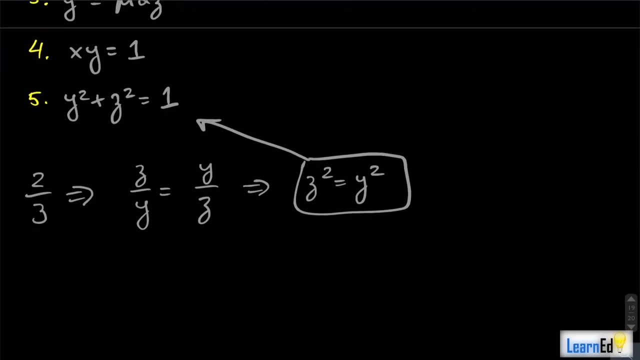 and then actually find out what these things are, rather than just kind of beating around the bush and just simplifying more and kind of running into a dead end. Okay, So if z squared equals y squared, then I can just write from equation 5: 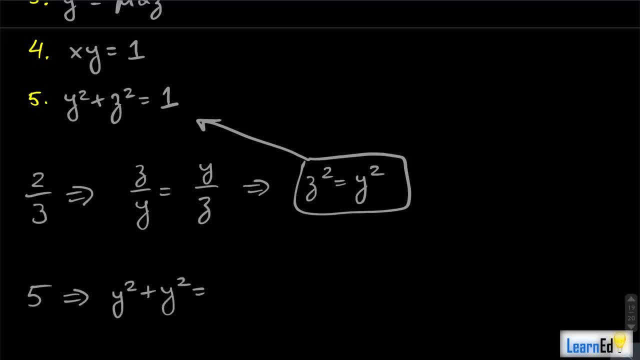 that y squared plus y squared equals 1.. And that gives me that 2y squared equals 1 and I can write that as y squared equals 1 half, Taking the square root of both sides, I get that y is equal to plus or minus rad 1 half. 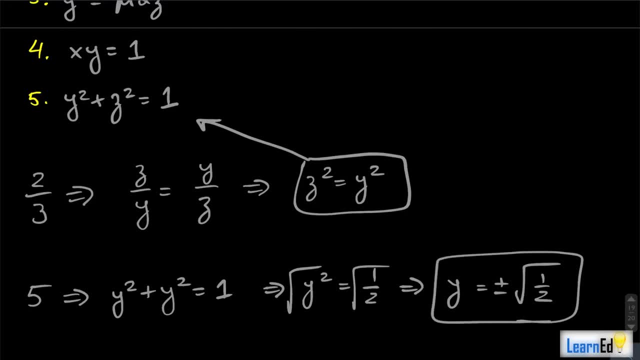 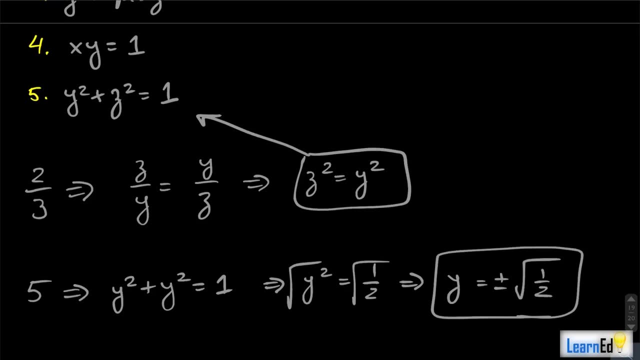 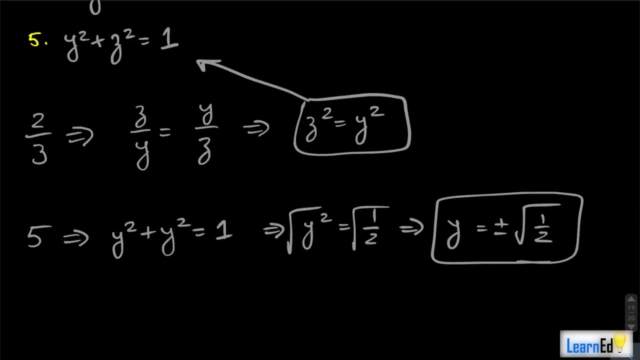 Now, this is where you need to be the most careful. Okay, And when I was originally looking at this problem, this is actually where I, you know, struggled a little bit, Because the thing about z right now, okay, z squared equals y squared, okay. 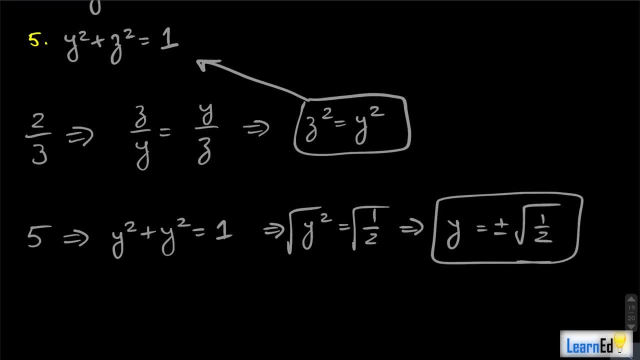 z squared. it doesn't matter if z is positive or negative. Okay, It could be anything. So when y is positive, rad 1 half, z can be plus or minus rad 1 half. So it can be, you know, if y is positive. 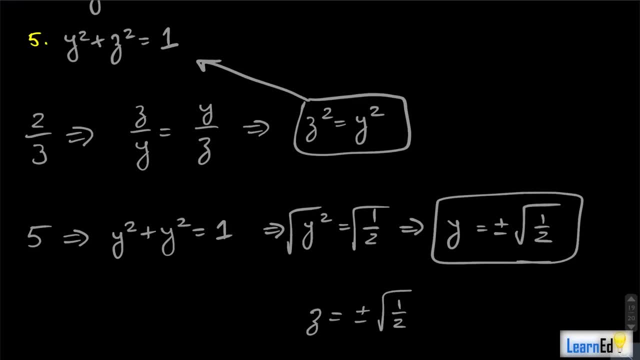 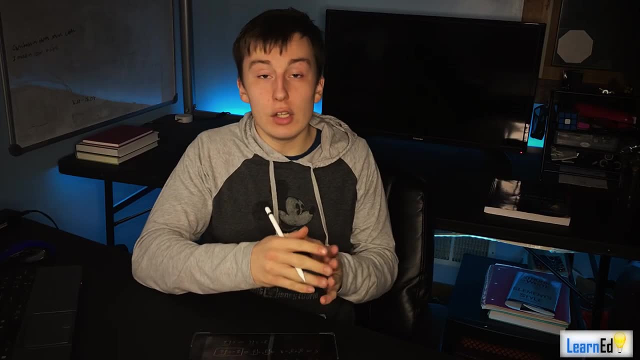 then z can be positive. If y is negative, z can be negative, Or it can be the other way around, Because the sign doesn't matter, okay? So if y can be two things, z can be four things, Okay. 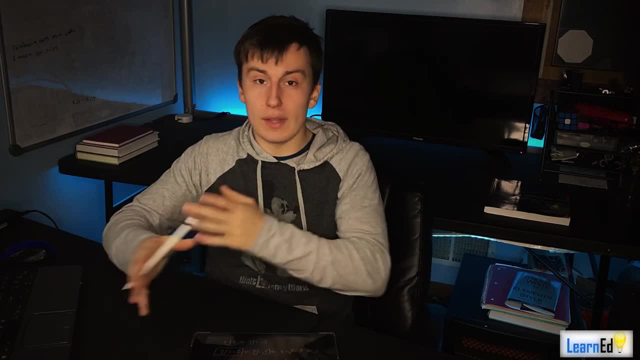 And you know, you can do it the other way around too. So if z, if you said z, can be two things, then y can be four things. Okay, Because it doesn't. it truly doesn't matter what the sign is. 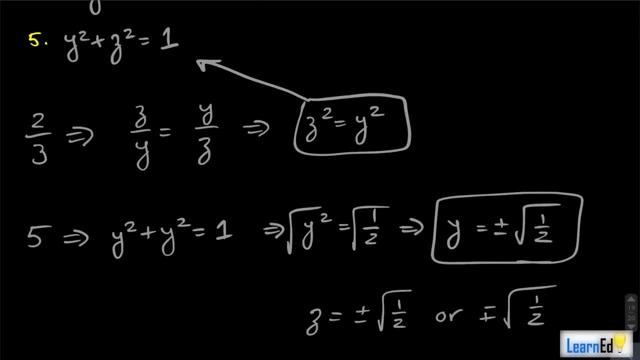 Okay. So it wouldn't be sufficient enough to say that z is plus or minus 1 half, because if you did, then if y is positive, then you're saying z has to be positive. Okay, That's not the case. 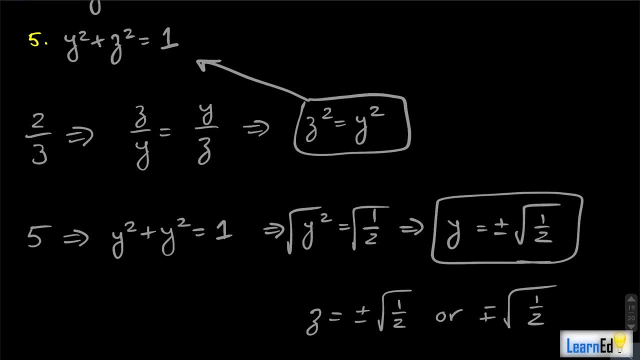 z can also be negative when y is positive. So you have to have actually four cases of z to compensate for this. Okay, And that's just kind of the limits of when you have multiple plus or minuses in your solutions. that's the actions that you have to take. 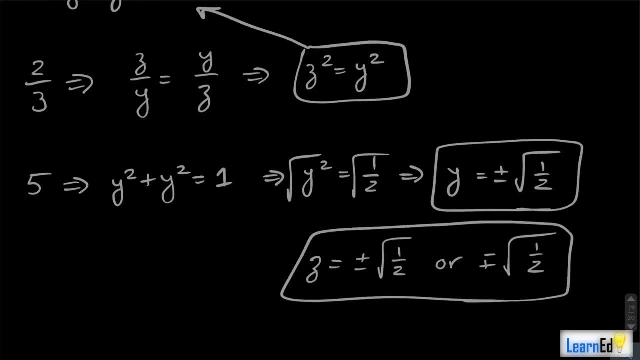 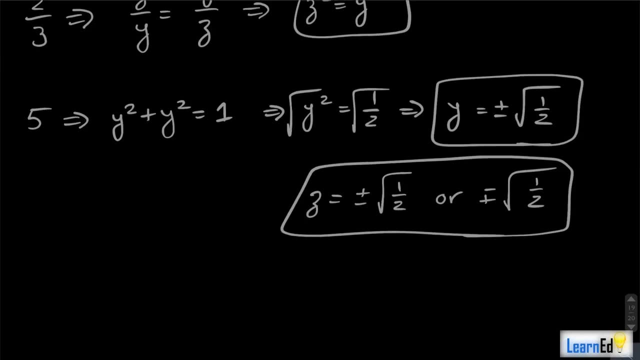 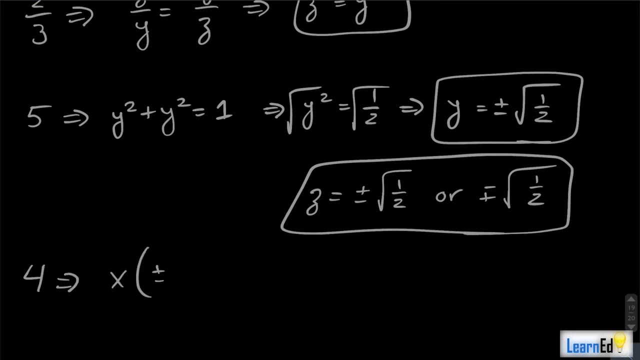 So that's why that z, and we also need to find x. Well, we have that xy equals 1.. Okay, So if xy equals 1, we use equation 4, and we get that x times plus or minus red 1 half. 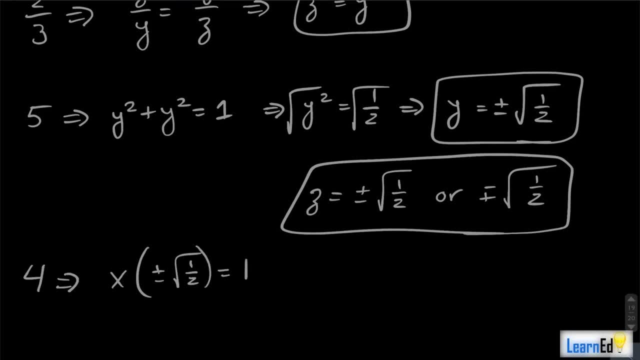 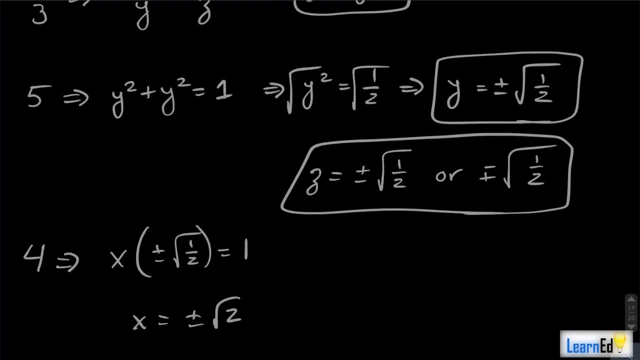 equals 1.. And if you divide by the square root of the plus or minus square root of 1 half on each side, you get that x is equal to plus or minus red 2.. Okay, So now you have your x, y and z. 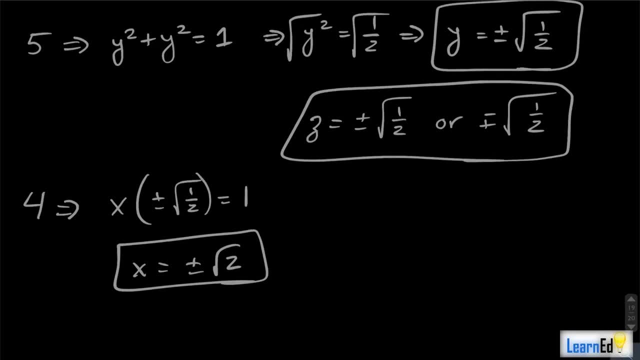 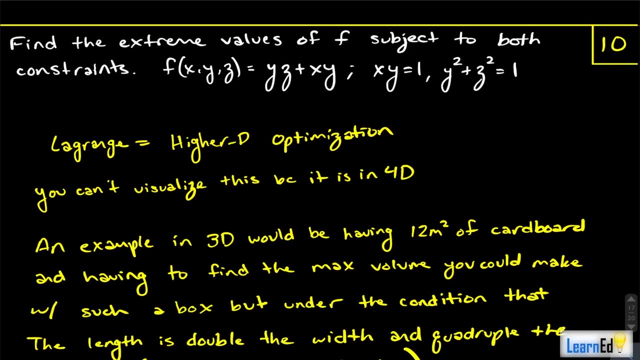 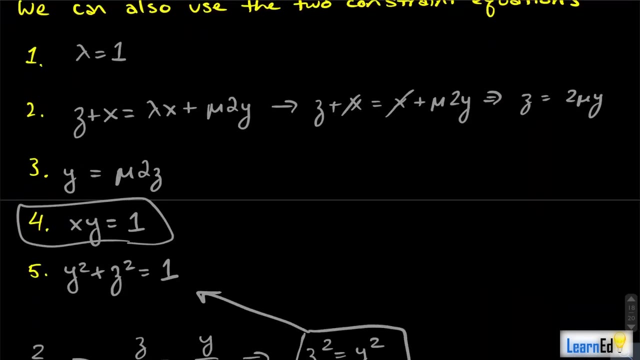 So you're going to have four different extrema to work out with. Okay, Remember what our original problem was asking for: We're finding the extreme value, So we're finding the extrema of f, Okay, And we want to actually find the value. 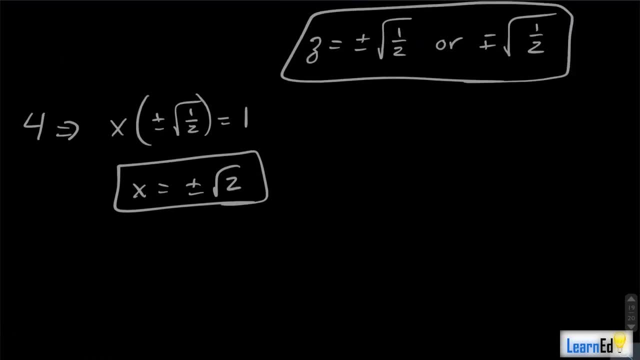 So we can't just like write the coordinates and call it good. We have to actually find the maximum Or, sorry, find the values of f. Okay, That's what it means by extrema Right. So if we find f at our first one, 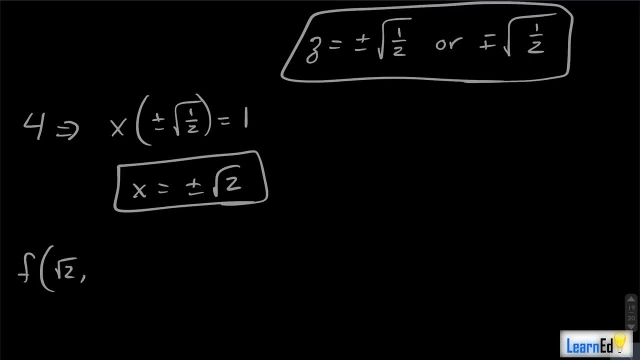 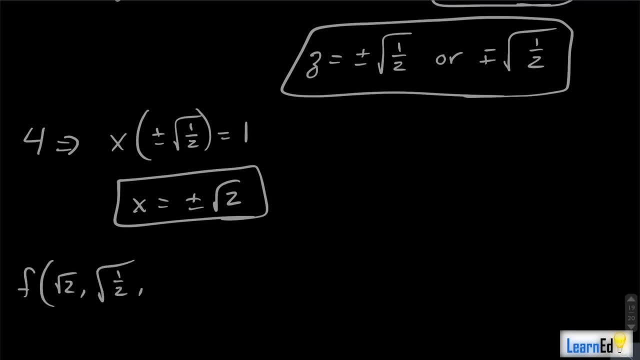 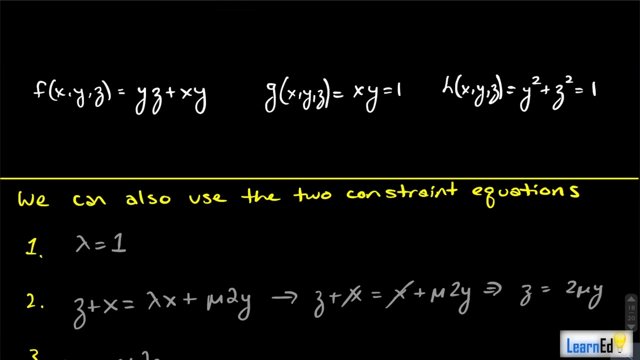 so let's say x is red 2, we'll say y is the square root of 1 half and we'll say that z is the square root of 1 half What we'll get. and remember what f is, I'll bring that down. 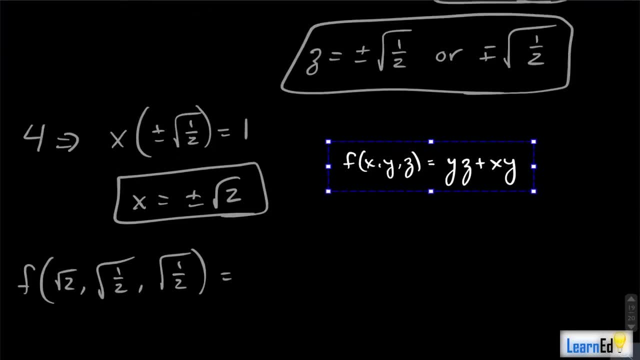 So we have it. Oh, I skipped. Okay, F is right there. So we have y, which is square root of 1 half times z, which is square root of 1 half plus red 2 times 1 over red 2.. 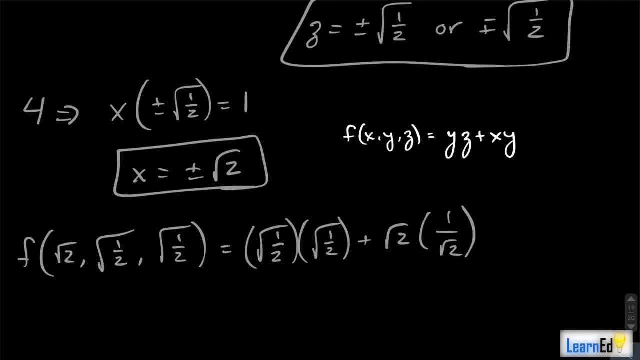 Okay, It's actually nicer to write this as 1 over red 2 rather than red 1 half, So it just is less to worry about And you can see easily that the red 2s cancel off here and you end up with 1.. 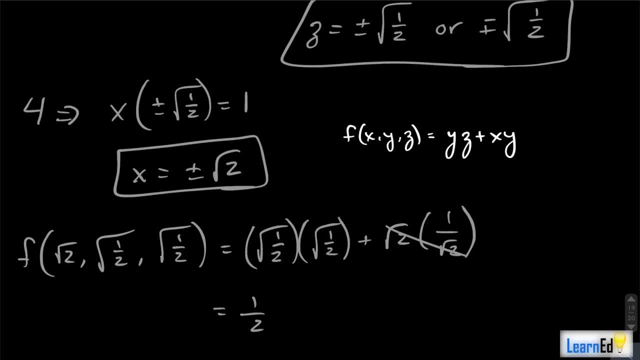 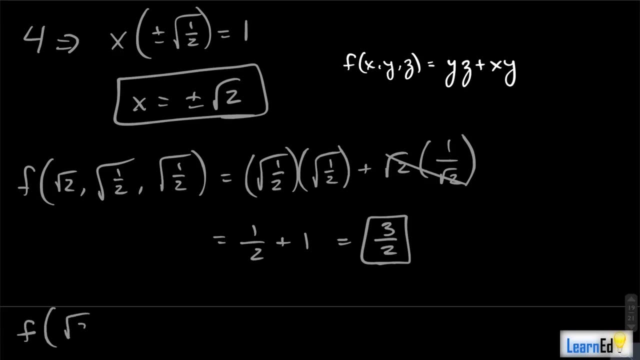 So red 1 half times red 1 half is 1 half. Then you have plus 1, so you get 3 halves here. So next is going to be red 2, red 1 half, and then we'll do when z is negative. 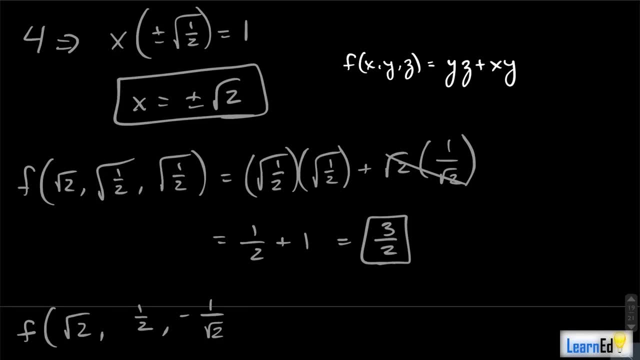 So we'll write it. I need to be more consistent with the notation, so let's just do like that, Okay, So this is going to be equal to y, which is 1 over red 2, times z, which is negative, 1 over red 2,. 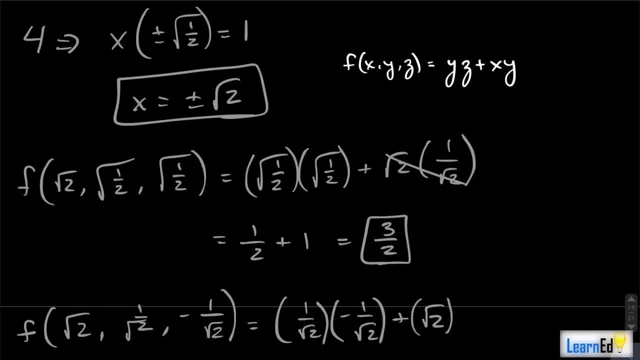 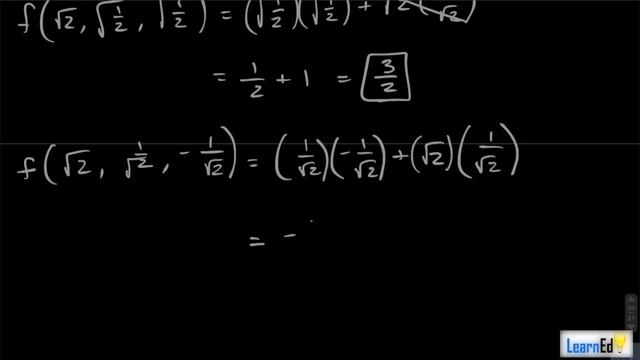 plus x is red 2, and y is 1 over red 2.. You get that this is equal to: we have a negative 1 half plus 1.. That gives you 1 half. So already you have multiple extrema. 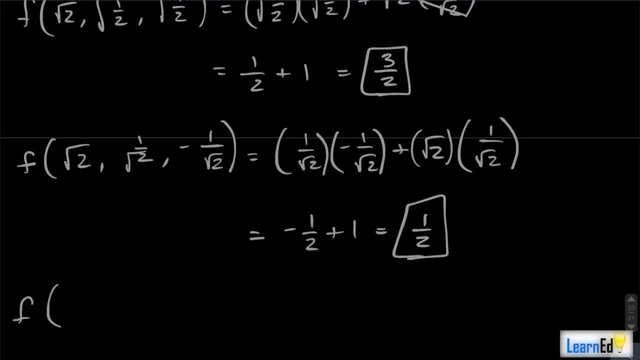 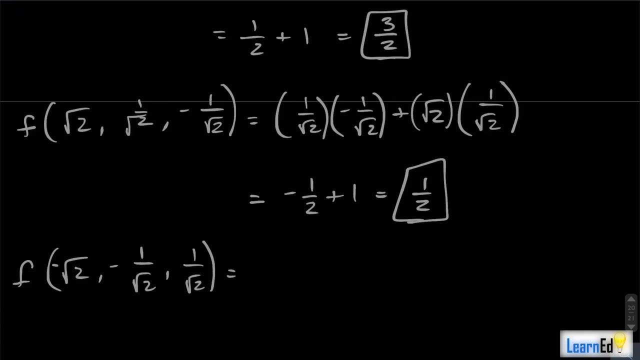 Now, if you keep going here, you get red 2, oh sorry, you can do negative red 2 now Negative 1 over red 2 and 1 over red 2 to get y times z is going to be negative 1 half. 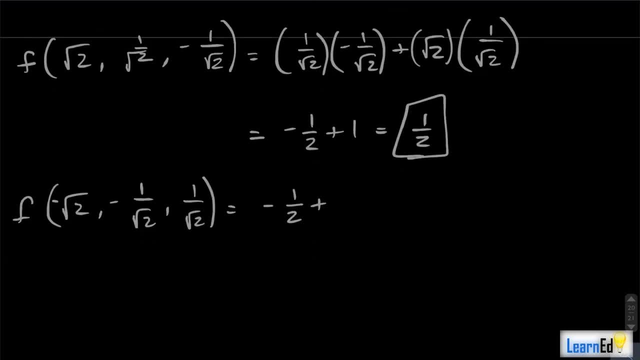 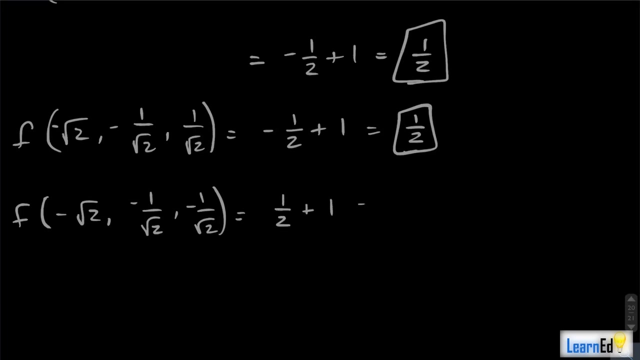 plus xy is just going to be 1, and you get 1 half again. And lastly, if you did all these things as negative, you get, remember, yz plus xy. So we have a 1 half here and then we'll get a plus 1 here. 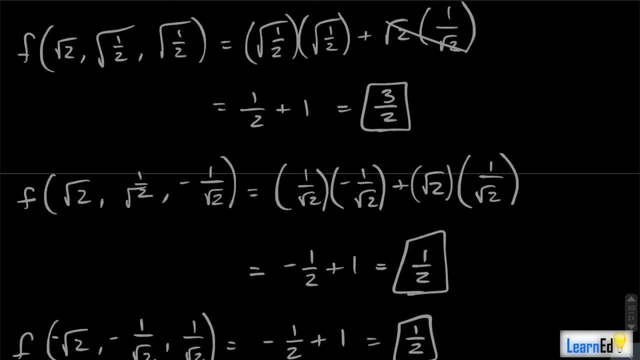 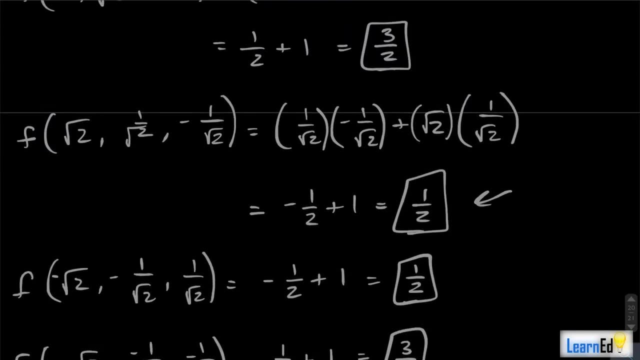 and we'll have a 3 halves. So our two, our two values are going to be 3 halves and 1 half. So you can see here that then 1 half will be a minimum because it's smaller than 3 halves. 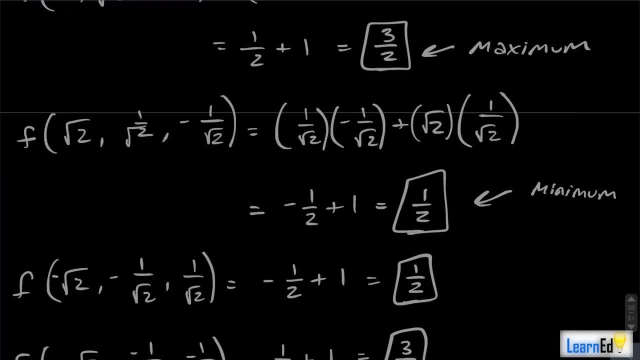 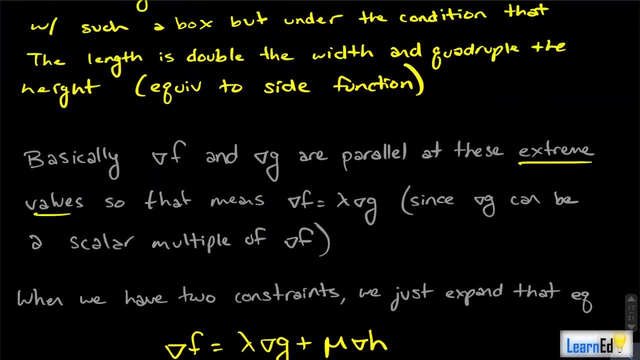 so this guy will be a maximum And that's it. Okay, so Lagrange multipliers are a you know, and I'm going to go over this whole thing real quick, just because Lagrange multipliers are a tough topic, because it's so lengthy. 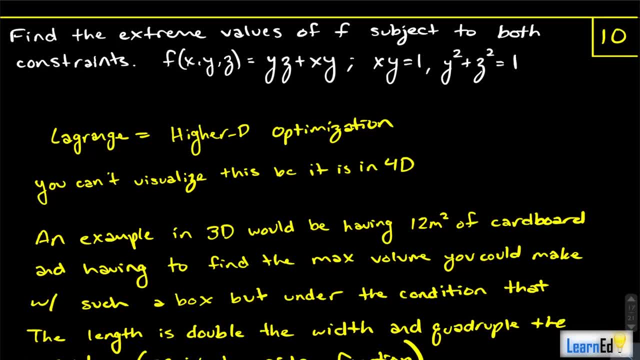 It's kind of like partial fraction decomp, Because it's a lot of algebra you know. So this is basically, you know, a higher dimensional optimization problem. Okay, I gave you an example of kind of what Lagrange multipliers can be useful for. 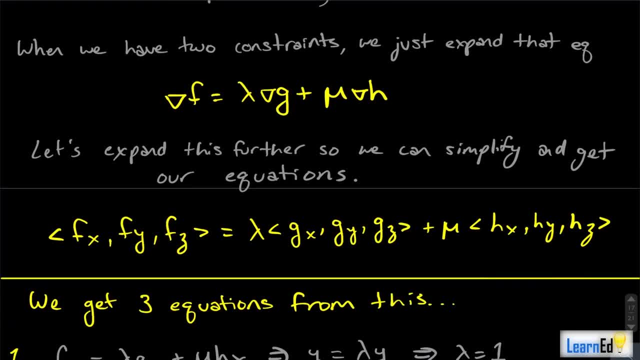 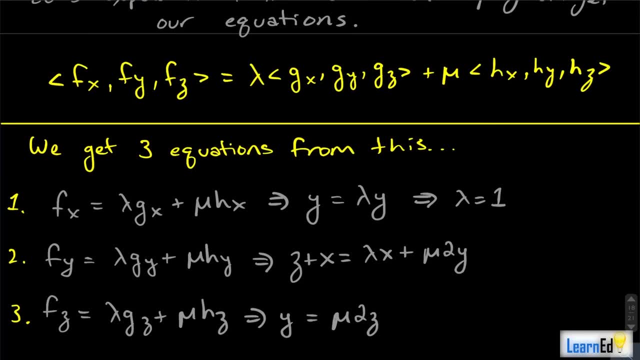 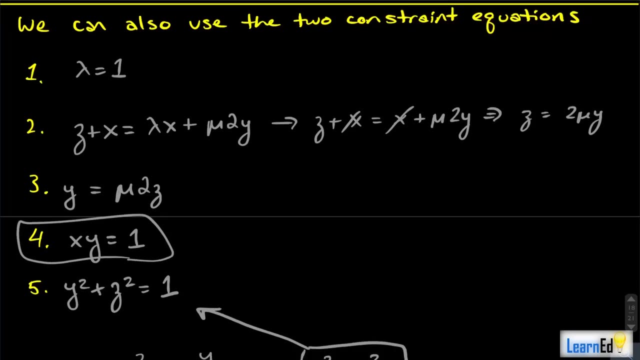 Okay, We talked about how we set up the Lagrange multiplier equation And you know, we start out getting our first three equations from this big thing. All right, We use our constraints with our five equations and then we're just solving for all the values of x, y and z. 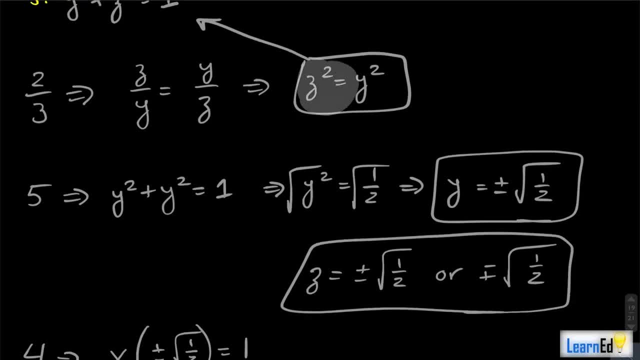 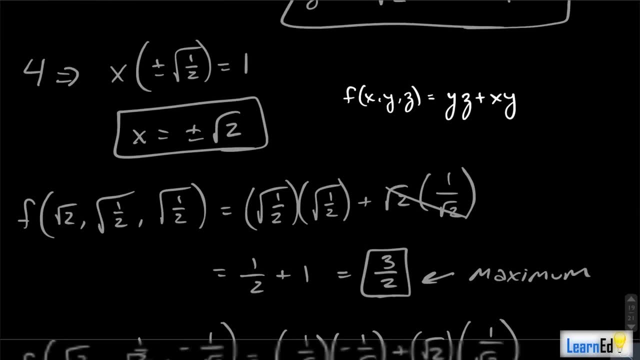 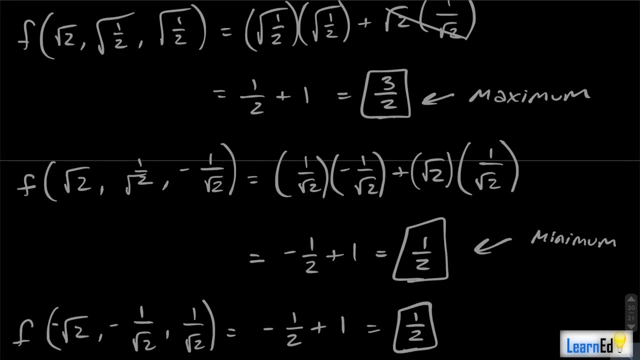 Okay, We found those, So we found not here. We found y, We found z, We found x And then we just found the actual values of the extrema Right. So let's say that this function was like: what do we have? 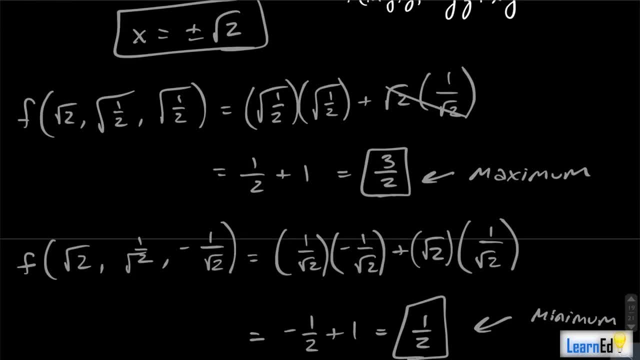 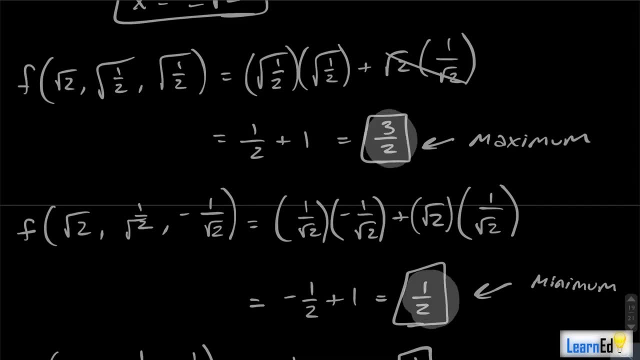 So this is, yeah, This function. So let's say that this function of x, y and z is w. So we found that w is three halves and w is one half. That's the max and the min, Okay. 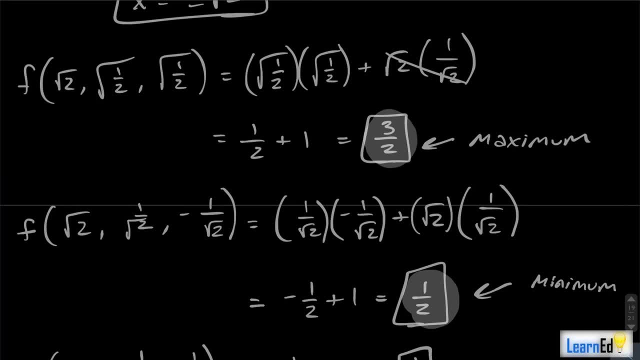 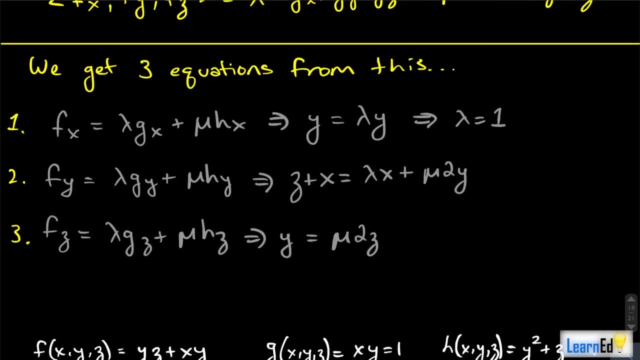 So you know, that's the whole idea of Lagrange multipliers. So it starts off with algebra, or it starts off with a little bit of partial derivatives and it ends with some algebra And that's really it. Okay, So really lengthy but honestly not the hardest thing in the world. 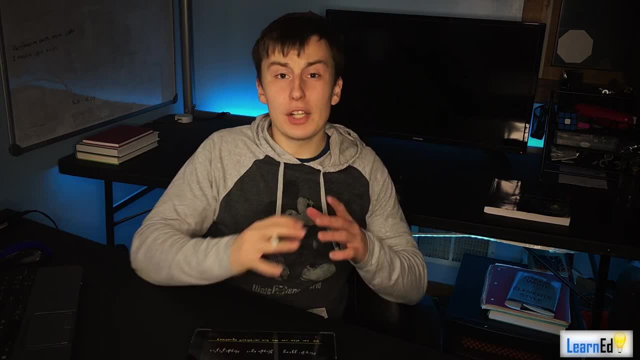 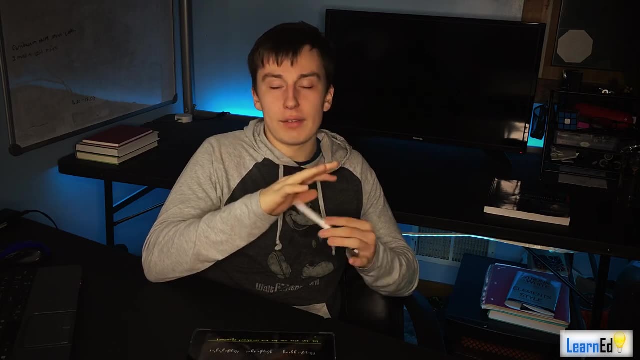 All right, So that's going to do it for part one of our Calc 3 final review. Next time we're going to be going over- in the next video- we'll be going over some double integrals, triple integrals, and then we'll be going over change of variables as well.